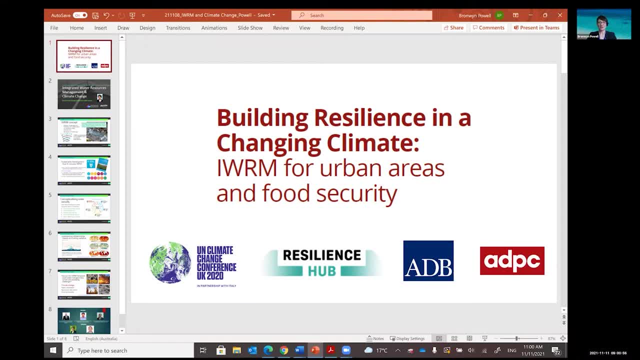 and this Resilience Hub event, supported by Asian Development Bank and the Asian Disaster Preparedness Centre. So, to begin with, we have an exciting program for you today. We have three speakers who will speak to integrated water resource management generally and disaster preparedness. We'll focus on cities and the impact of climate change on cities, and then the impact 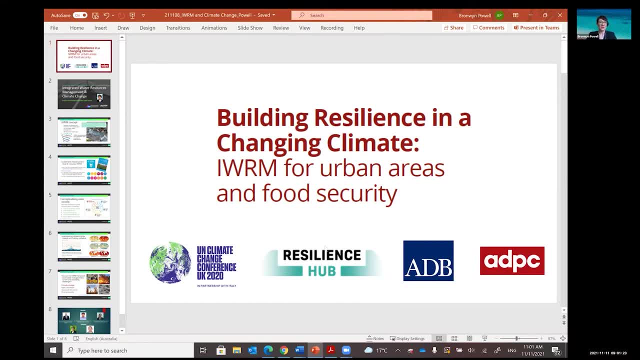 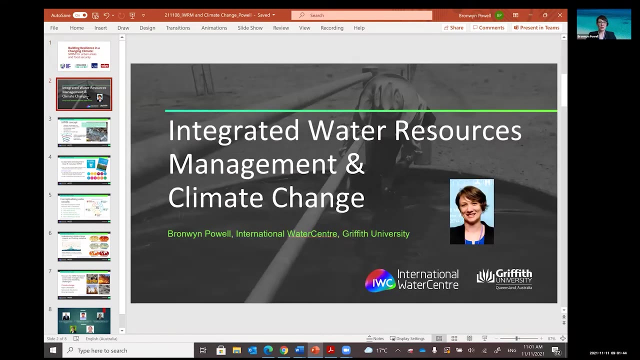 of climate change, on food security in Asia, We will then have a panel session, and two panellists will join us for that. So first of all, I'd like to just set the scene by talking about providing a bit of context, and then we'll go to our speakers. So, on this topic of integrated water resource management and climate, 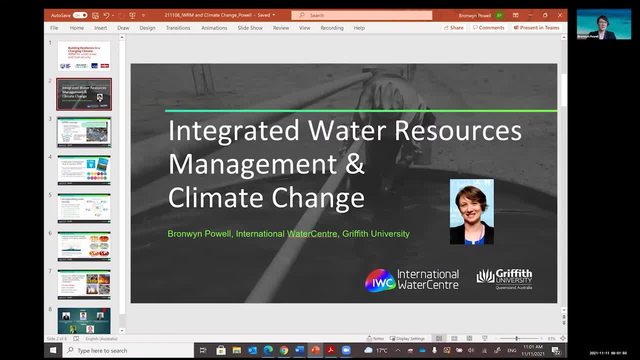 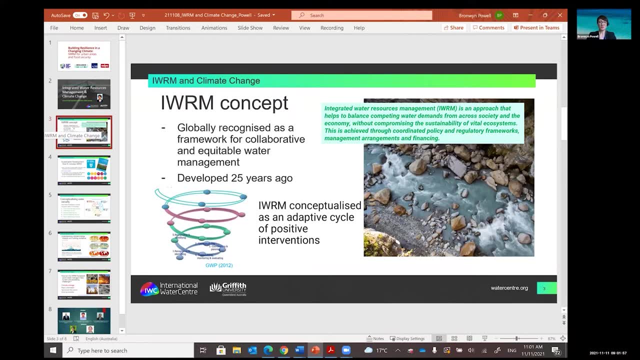 change. it's a big topic. There's a lot to cover in this, But where did we start? Well, integrated water resource management concept has been around for 25 years. Many of you will be very familiar with it. It's globally recognised. It's been around for a long time. It's been around for a long. 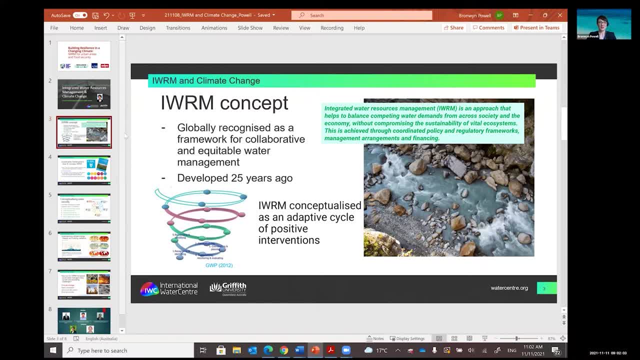 time. It's a frame that has been developed as a framework for collaborative and equitable water management. We would like to just have a look at how it's developed over time. So it has been in some cases conceptualised as an adaptive cycle of positive interventions. It deals with competing. 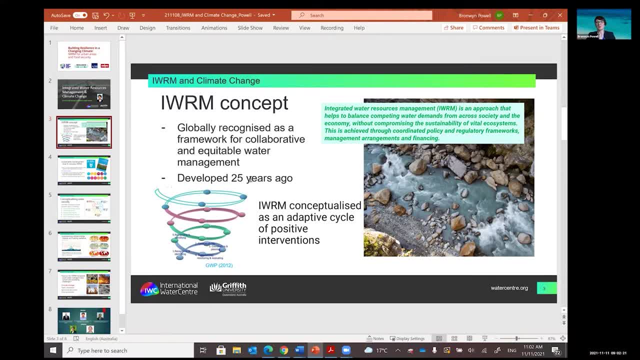 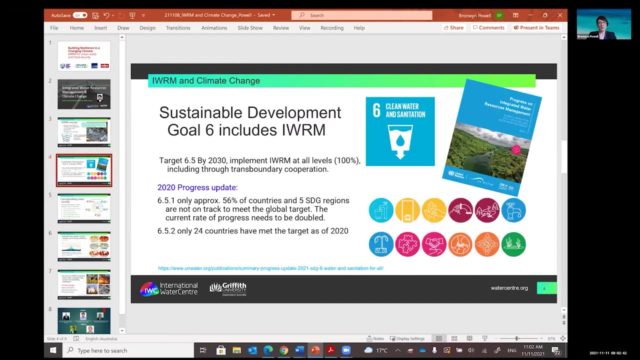 demands across society and the economy, but aims to not compromise sustainability of vital ecosystems. So I think that this is where climate change is having the impact that we can't just. we are seeing ecosystems are reaching tipping points and being very negatively affected by an intensifying hydrological cycle. So where are we at with IWRM as a concept? Well, it's well. 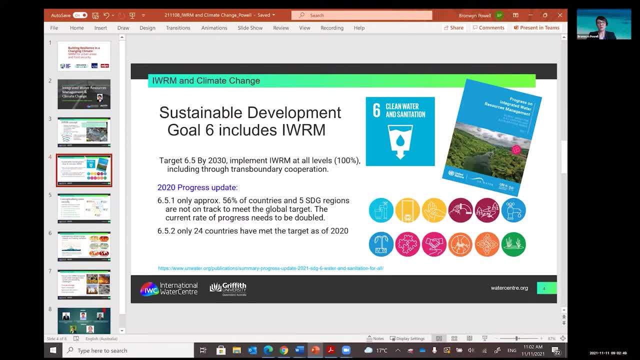 integrated into SDG 6, which is water and sanitation for all, but considering sustainability as well and water resource management. So it's mentioned in target 6.5, which is about the implementation of integrated water resource management at all levels And in 2020, we saw 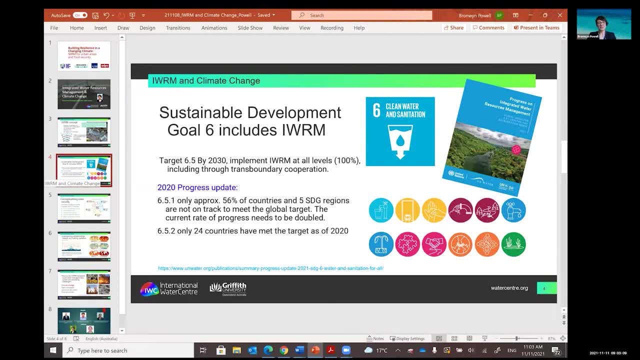 the progress update that only about 56% of countries in the regions are on track to meet this global target. And one challenge of IWRM is it's a process orientated goal, whereas other goals are a little bit easier to achieve. So we're seeing a lot of progress in the process. 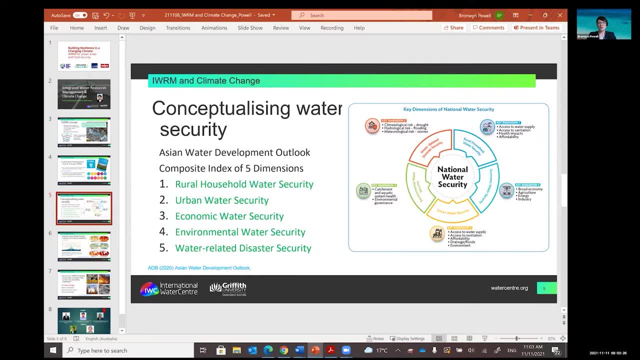 and it's easier to measure. So how can we conceptualize water security? Well, one way this is done is through the Asian Development Bank's Asian Water Development Outlook, which is a composite index containing five dimensions: rural, household, water security, urban water. 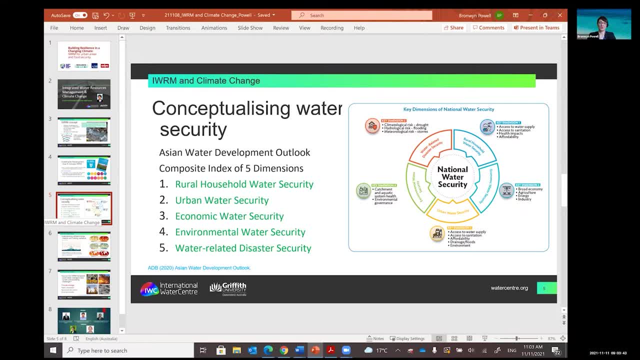 security: economic water security and environmental water security. And then climate change comes into this fifth dimension, which is water-related disaster security. So today we consider the three of those elements And we're going to look at the five dimensions. So we're going 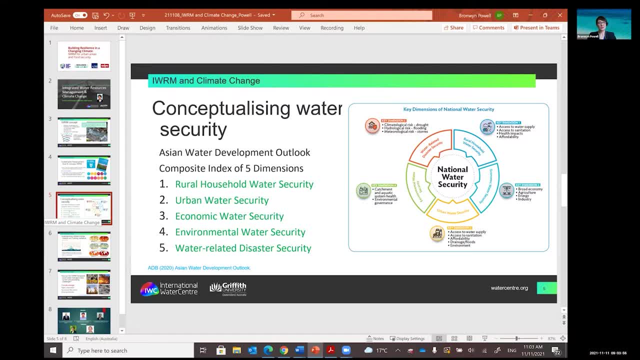 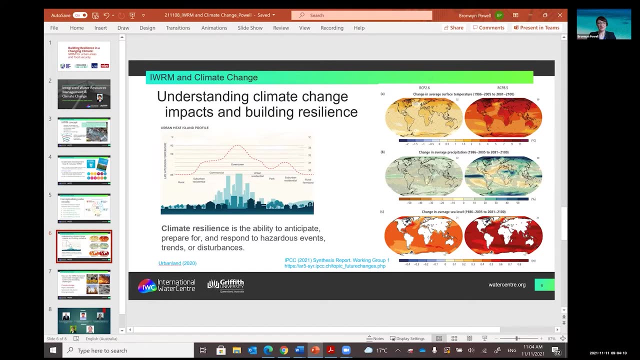 to look at the five elements in more depth: urban water security, economic water security, which includes agriculture production, and then water-related disaster security. We're focusing a bit more about understanding climate change impacts and building resilience. We see here a heat island diagram of cities, So we know temperatures are increasing in cities Also that. 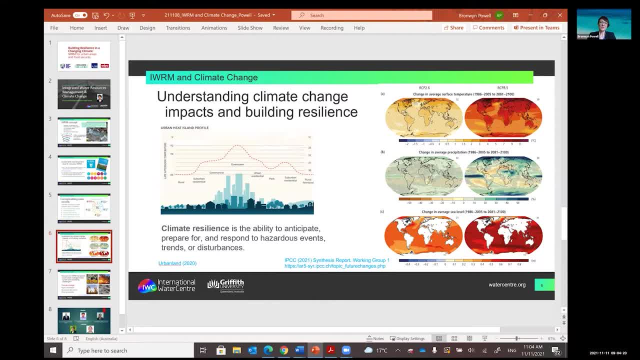 means higher evapotranspiration, And also we're seeing more and more intensification of severe events: droughts, floods, etc. What is climate resilience? Well, it's the ability to anticipate, prepare for and respond to hazard events, trends and disturbances. So 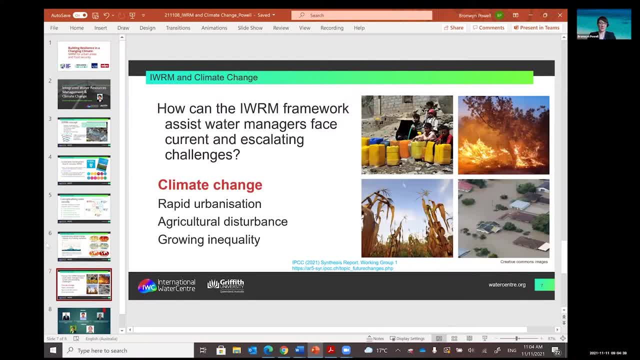 one of the big questions for today's session is how can the IWF framework assist managers to face current and escalating challenges, the biggest being climate change and rapid urbanization and agricultural disturbance and growing inequality. Our speakers will provide a lot more depth onto those topics. So, if I could introduce, our first speaker is Mr Hans Gutmann, who 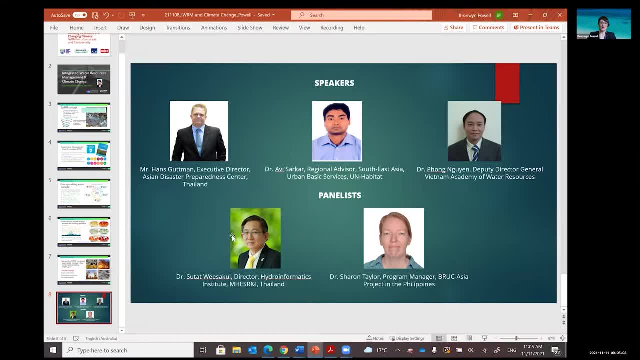 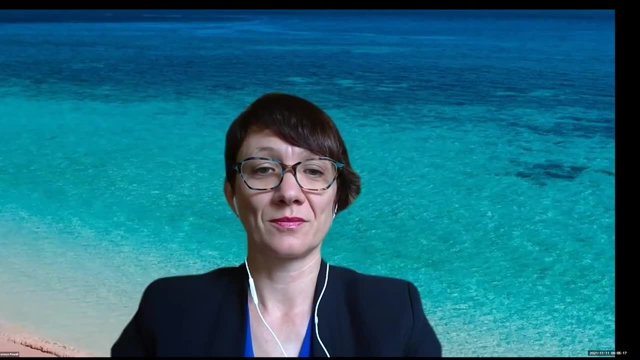 is Executive Director of the Asian Disaster Preparedness Center in Thailand. You can see there all our speakers and panelists today, And we'll introduce those as we go along. So over to you, Hans, Thank you, Thank you, And let me 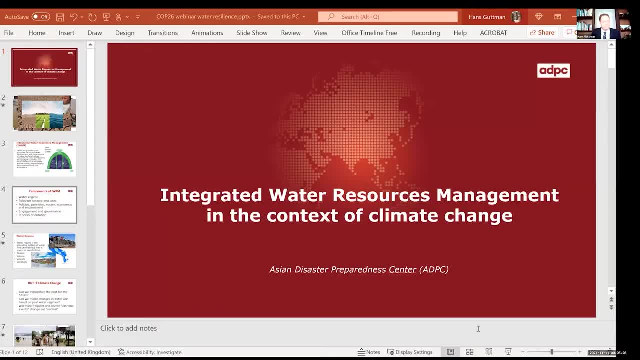 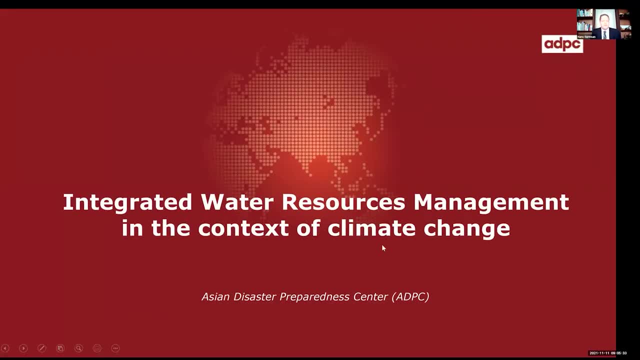 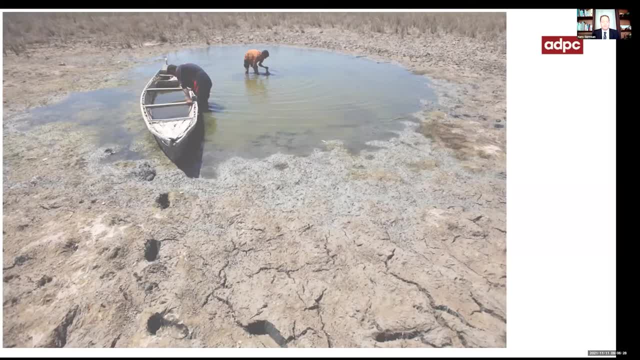 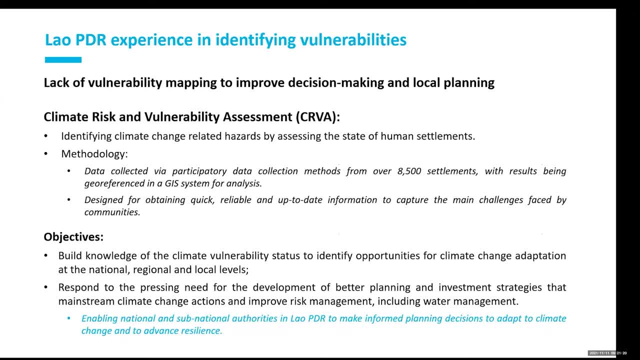 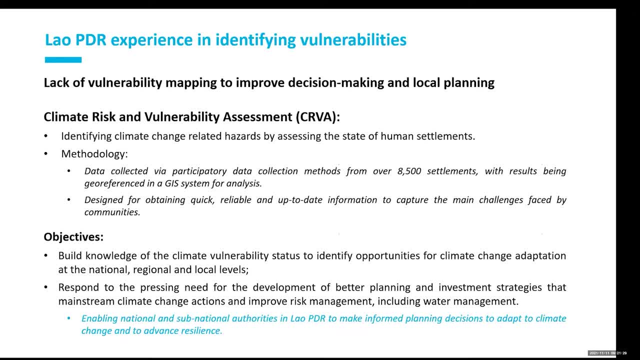 UN Habitat. we partnered with the Ministry of Natural Resources and Environment and developed a national climate risk and vulnerability assessment, which was aimed to identify the climate change related hazards, such as floods, droughts and storms, and assessing the state of human settlements. To do this, what we have done is that we collected data from all the settlements in Laos using participatory data collection methods. 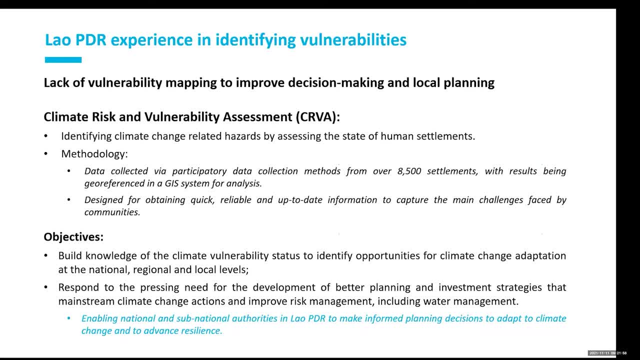 with results being georeferenced by a GIS system for analysis. So what this methodology enabled us to do was to quickly obtain very reliable, up-to-date information to capture the main challenges which are being faced by the communities. So, in short, the objective of this project is to create a global climate risk assessment. 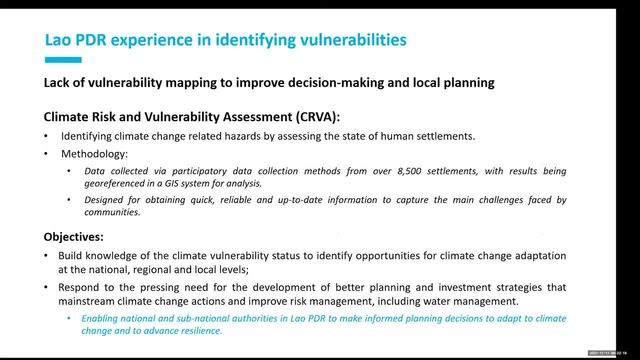 and the objectives of the assessment were, firstly, to gain knowledge of the climate vulnerability status, to identify climate change adaptation opportunities at the national, regional and local levels. Secondly, it was also to respond to the need to develop better planning and investment strategies to mainstream climate change consideration. 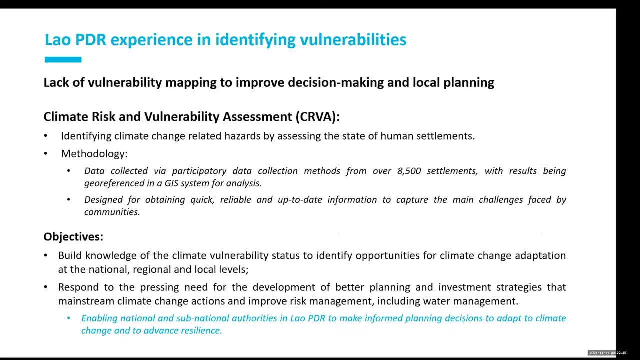 and, at the same time, to improve risk management, including that of water management efforts. Our effort with MONREA will enable the national and the sub-national authorities in Laopadia to make informed planning decisions to adapt to climate change and increase resilience. We have since received a number of requests from different development partners to make the data available for their programming efforts. 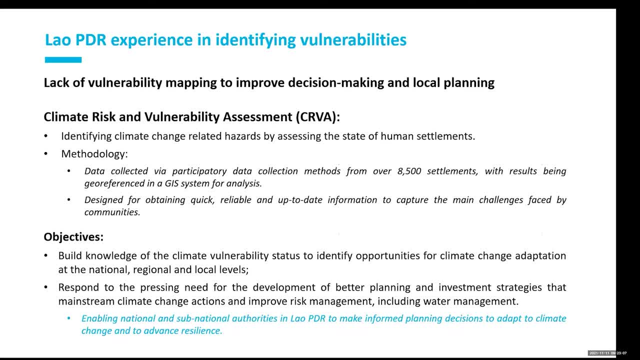 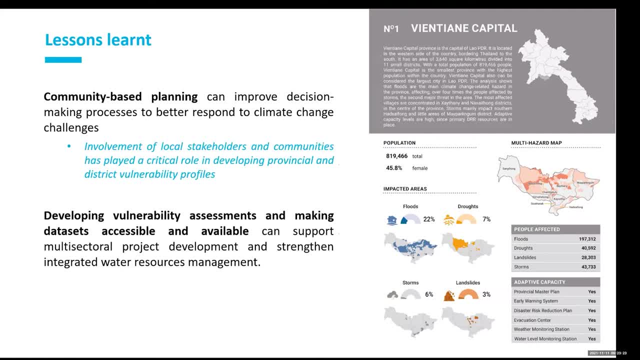 And just to finally talk about a bit of the lessons learned, is that community-based planning can improve decision-making processes to better respond to climate change challenges. And just to finally talk about a bit of the lessons learned, is that community-based planning can improve decision-making processes to better respond to climate change challenges. 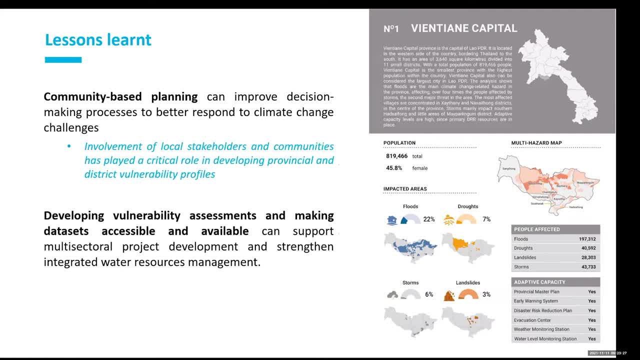 And just to finally talk about a bit of the lessons learned, is that community-based planning can improve decision-making processes to better respond to climate change challenges. And just to finally talk about a bit of the lessons learned, is that community-based planning can improve decision-making processes to better respond to climate change challenges. 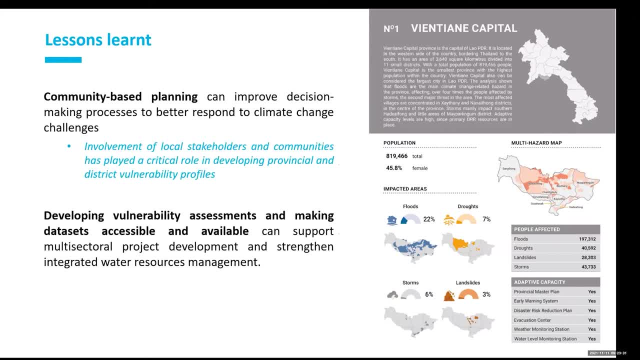 And just to finally talk about a bit of the lessons learned, is that community-based planning can improve decision-making processes to better respond to climate change challenges. And just to finally talk about a bit of the lessons learned, is that community-based planning can improve decision-making processes to better respond to climate change challenges. 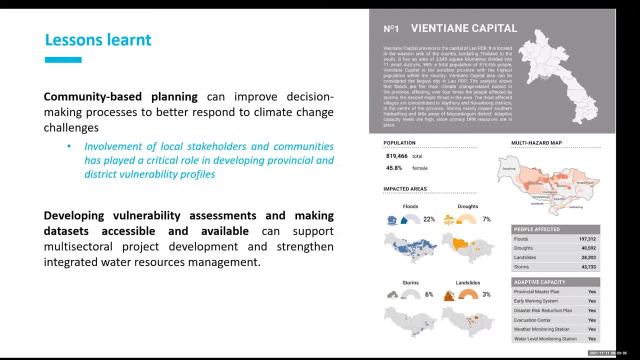 And just to finally talk about a bit of the lessons learned, is that community-based planning can improve decision-making processes to better respond to climate change challenges. And just to finally talk about a bit of the lessons learned, is that community-based planning can improve decision-making processes to better respond to climate change challenges. 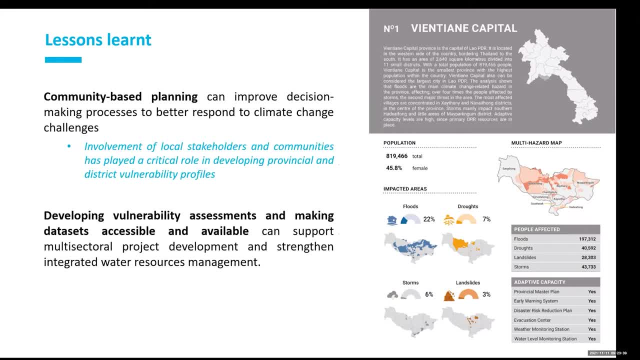 And just to finally talk about a bit of the lessons learned, is that community-based planning can improve decision-making processes to better respond to climate change challenges. And just to finally talk about a bit of the lessons learned, is that community-based planning can improve decision-making processes to better respond to climate change challenges. 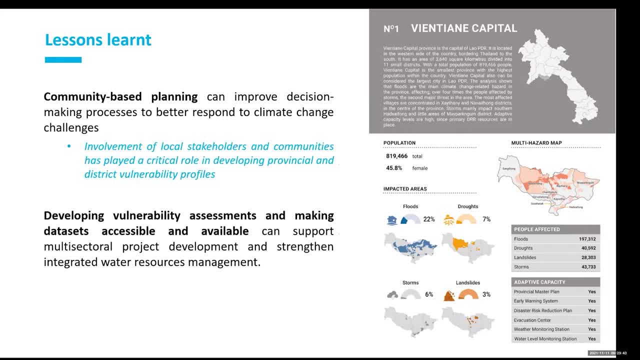 And just to finally talk about a bit of the lessons learned, is that community-based planning can improve decision-making processes to better respond to climate change challenges. And just to finally talk about a bit of the lessons learned, is that community-based planning can improve decision-making processes to better respond to climate change challenges. 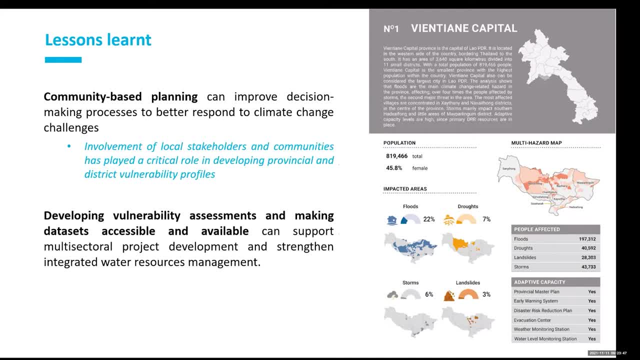 And just to finally talk about a bit of the lessons learned, is that community-based planning can improve decision-making processes to better respond to climate change challenges. And just to finally talk about a bit of the lessons learned, is that community-based planning can improve decision-making processes to better respond to climate change challenges. 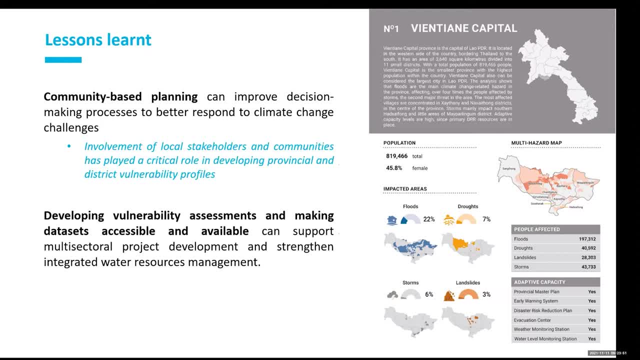 And just to finally talk about a bit of the lessons learned, is that community-based planning can improve decision-making processes to better respond to climate change challenges. And just to finally talk about a bit of the lessons learned, is that community-based planning can improve decision-making processes to better respond to climate change challenges. 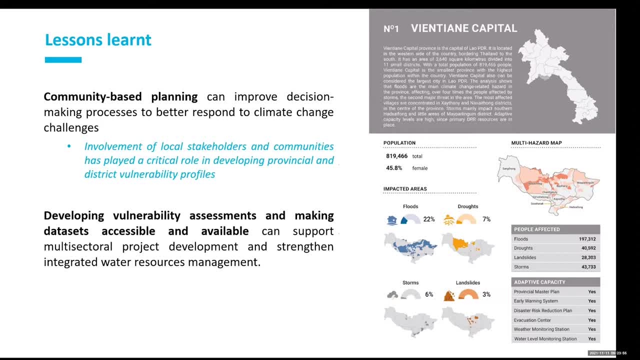 And just to finally talk about a bit of the lessons learned, is that community-based planning can improve decision-making processes to better respond to climate change challenges. And just to finally talk about a bit of the lessons learned, is that community-based planning can improve decision-making processes to better respond to climate change challenges. 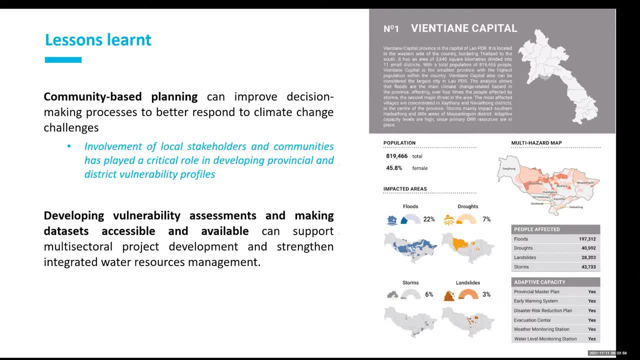 And just to finally talk about a bit of the lessons learned, is that community-based planning can improve decision-making processes to better respond to climate change challenges. And just to finally talk about a bit of the lessons learned, is that community-based planning can improve decision-making processes to better respond to climate change challenges. 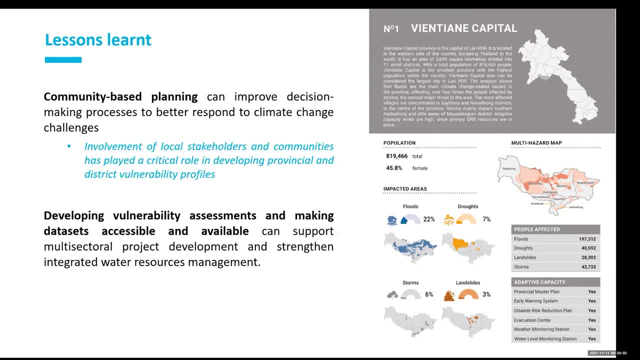 And just to finally talk about a bit of the lessons learned, is that community-based planning can improve decision-making processes to better respond to climate change challenges. And just to finally talk about a bit of the lessons learned, is that community-based planning can improve decision-making processes to better respond to climate change challenges. 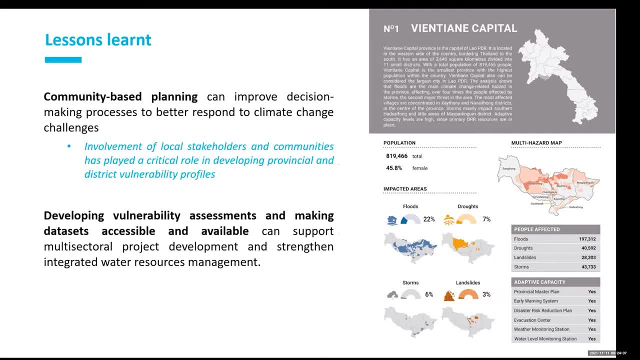 And just to finally talk about a bit of the lessons learned, is that community-based planning can improve decision-making processes to better respond to climate change challenges. And just to finally talk about a bit of the lessons learned, is that community-based planning can improve decision-making processes to better respond to climate change challenges. 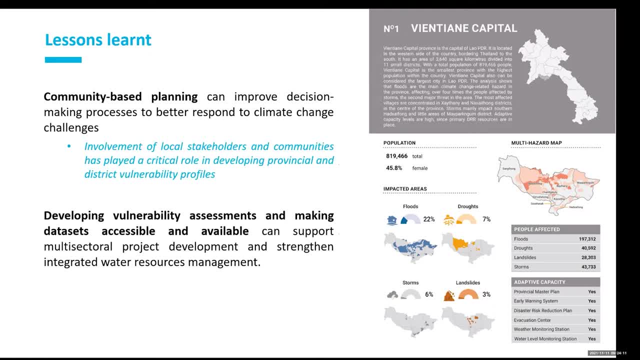 And just to finally talk about a bit of the lessons learned, is that community-based planning can improve decision-making processes to better respond to climate change challenges. And just to finally talk about a bit of the lessons learned, is that community-based planning can improve decision-making processes to better respond to climate change challenges. 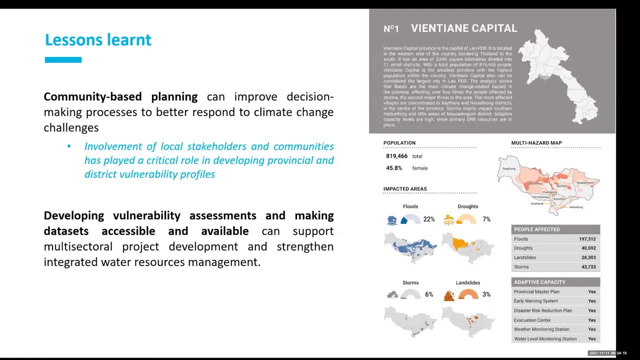 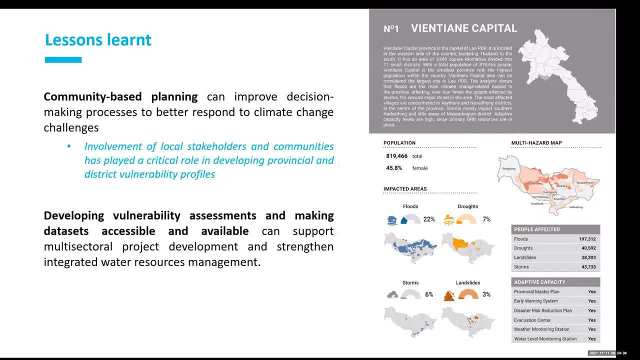 And just to finally talk about a bit of the lessons learned, is that community-based planning can improve decision-making processes to better respond to climate change challenges, sectoral project development and strengthen integrated water resource management. As I had mentioned earlier that many of the developed partners are reaching out. 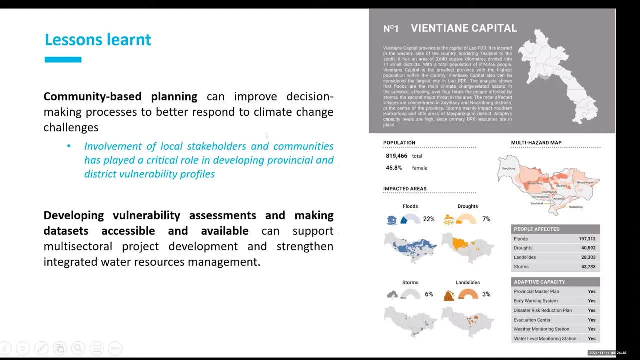 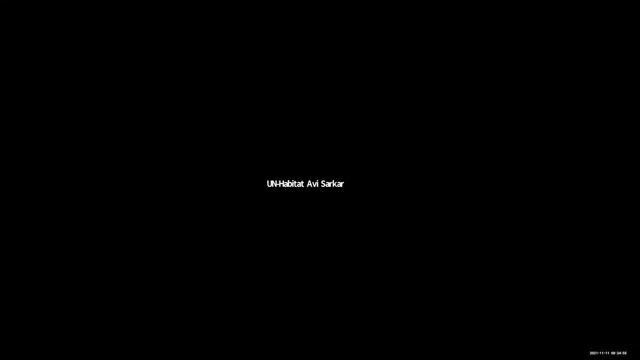 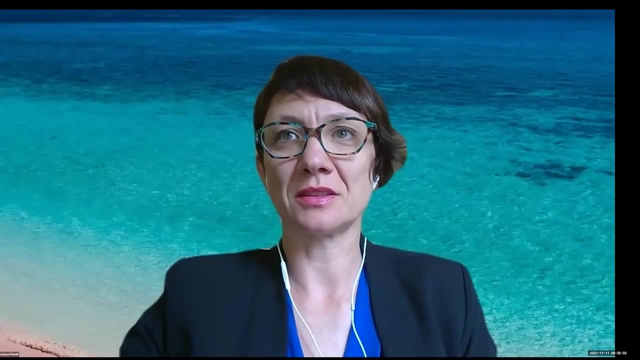 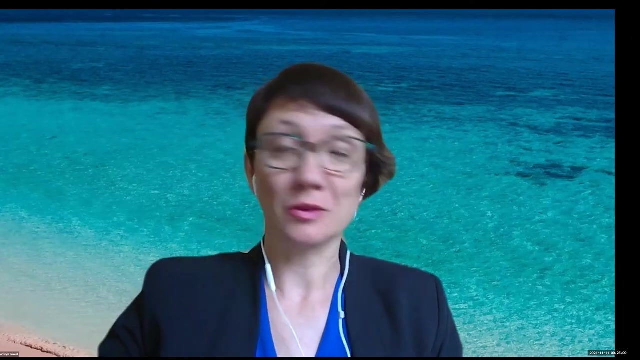 and we are cooperating and collaborating with them on this issue, Thank you. Thank you so much, Avi. That was fascinating to hear about the massive data collection exercise you have been through there And I'm looking forward to asking more questions about that during the Q&A session. 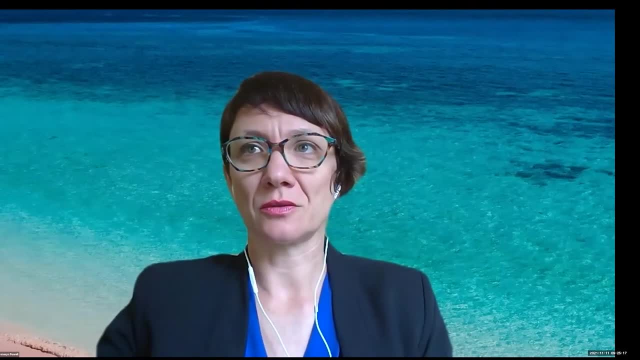 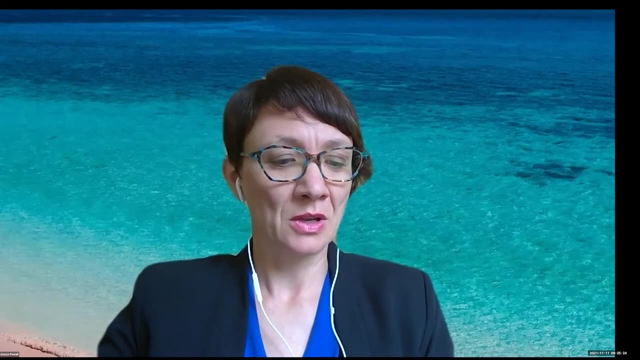 Now I'd like to introduce our next speaker. It's Dr Phuong Nguyen, who's the Deputy Director General from the Vietnam Academy of Water Resources. We're looking forward to him speaking about climate change impacts on food security and irrigation. Thank you, 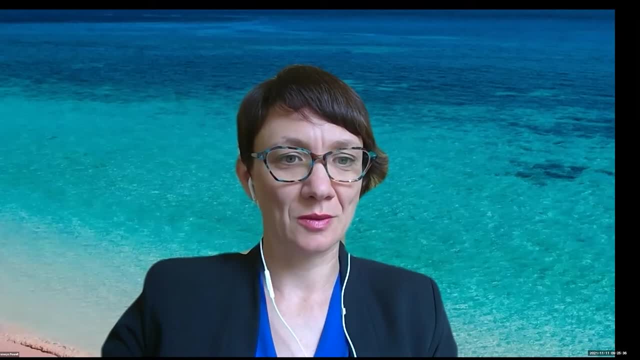 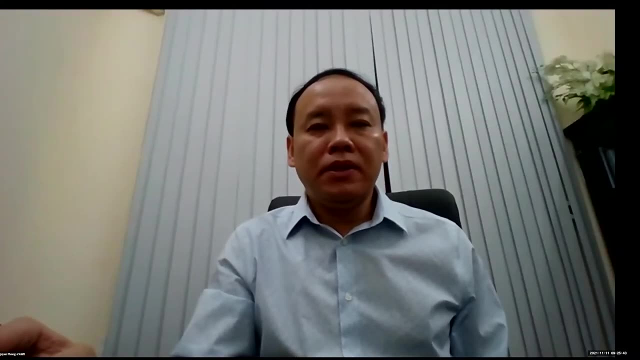 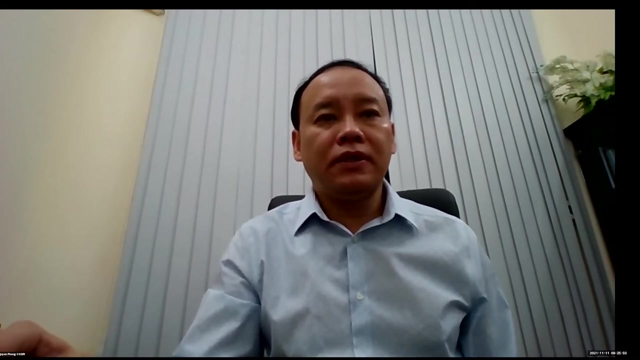 And Dr Phuong, please feel free to now share. I'll share your screen as well and slides. Okay, thank you very much. I would like to thank ADB and ADPC to give me a chance to talk a little bit about adaptation measures for the food securities. 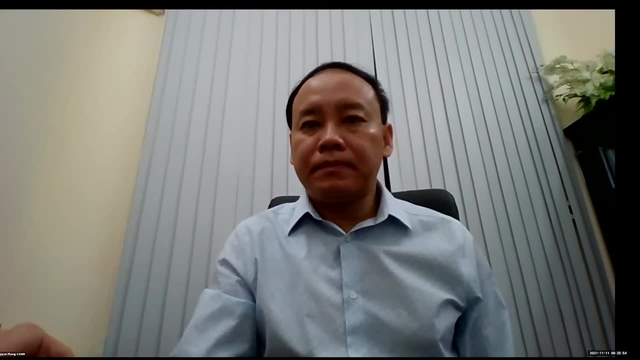 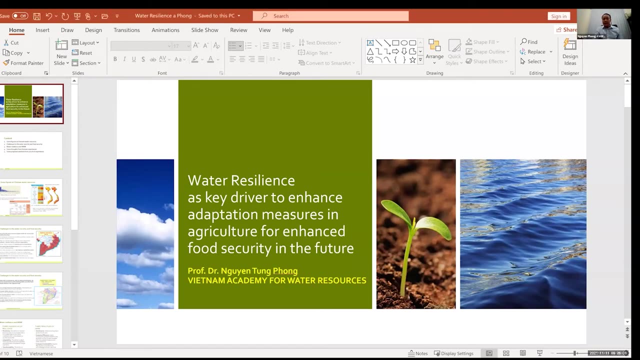 and also for the agriculture, Okay. Okay, can you see that? Yes, we can see that. Maybe try presentation mode. Yes, we can if you want to. Yes, now is the moment. Thank you, Thank you, Okay. 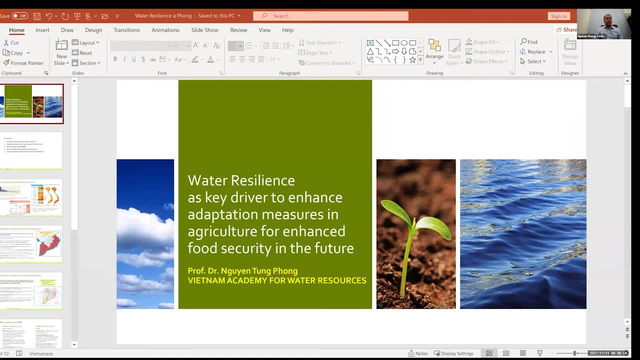 So first, so my presentation including five contents. First is some peers on the Vietnam War resources. Together is the challenge of the world's security and food security. Third ones ishte тр, trotzdem and safety and resilience at ID secretariat, And the fourth one is 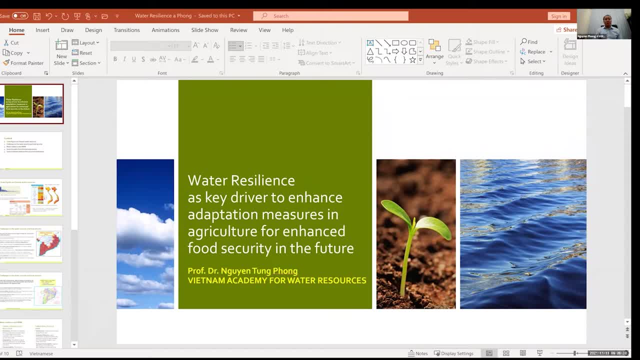 some thoughts from Vietnam experience, and the fifth one is some proposal solution. This is our role: to include this data, the practical experiences. so i would like to start with the some figures on vietnam war resources and you would see that most of the river basin in vietnam will experience different levels of the 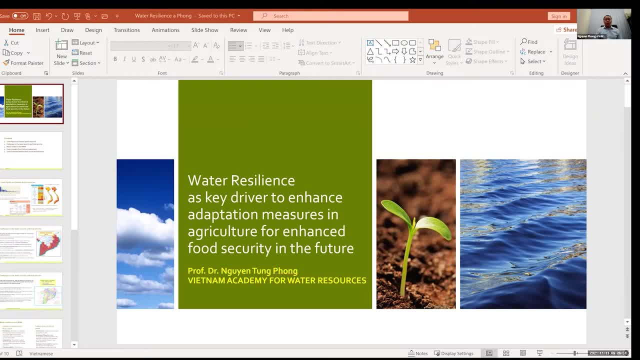 stress, by using the water exploitation index in the. so we would see, you would see that all the river basin would be a scale of waters in the futures. and the second one is the, the worry use of agriculture's account. sorry, sorry, i need to interrupt, dr fong. i'm sorry with the slides. 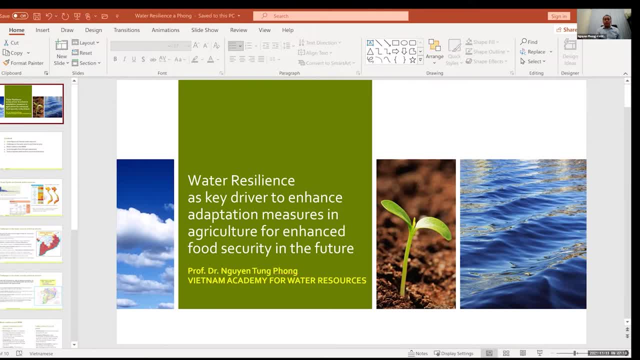 are not progressing with what we can see. are you moving ahead? you could not see the presentation there. i can see, but it's not changing slides. okay, yeah, uh, dr form, if it's okay, adb will share the slides. you can tell: next, next, next. okay, now, you see that. i will see that. 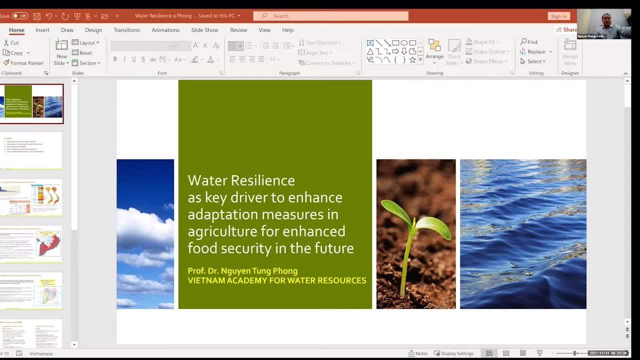 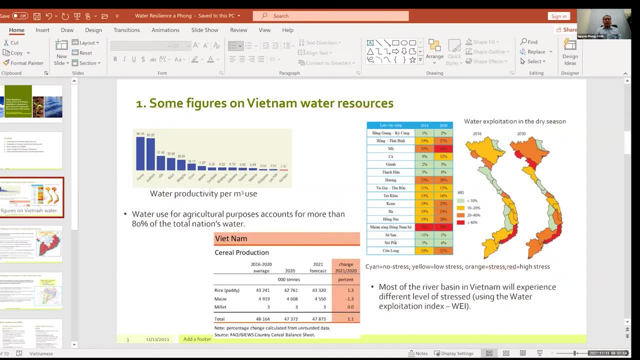 no, it's still the same. no, so maybe, um, we can request a. if you stop sharing, we can request adb. oh now, oh, no, you see that moving. yeah, now it's moving. okay, i use it. it's a better, okay. good, all right, thank you. so, uh, okay, so we're used for any conscious that propose accounts for more than 80. 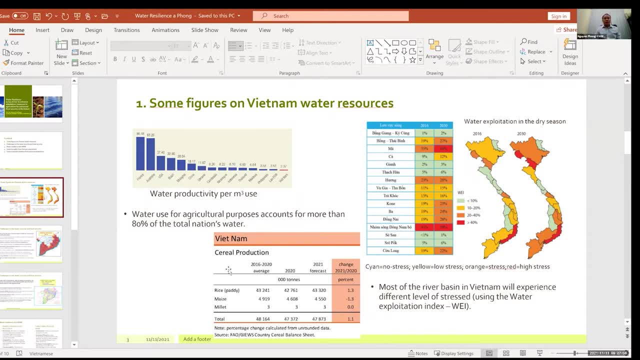 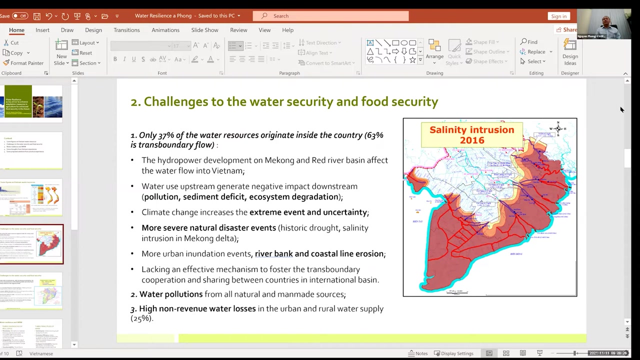 of total nation wars. and the third one is a world of activities is quite slow in vietnam, so that only uh a lot of um 2. uh, save 37 us dollars. that's uh the gdp created from the one square one cubic meters of the waters. and, and talking about the challenge of water security, that 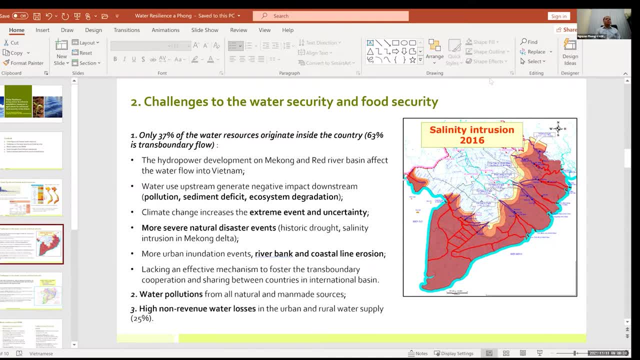 and full security. so only uh 37, 67% of who are resourced or is native inside of the Vietnam country, So 63% from the outside. So meanwhile the hydropower development in Mekong River or Red River quite affected the. 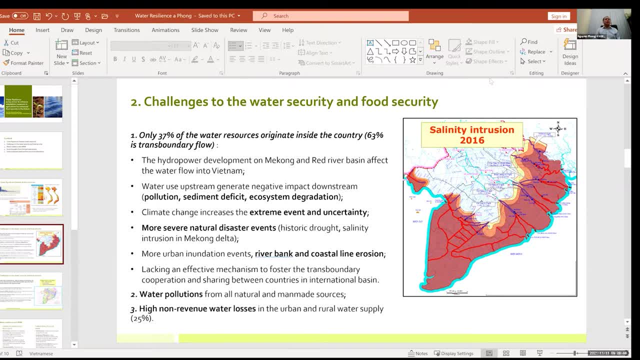 water flow in Vietnam. Second one is the activity in the upstream, So also generated negative impact due to downstream Is pollution, sediment deficit, ecosystem degradation And the third one, as Ham also mentioned and so my colleague also mentioned, about climate change, increased. 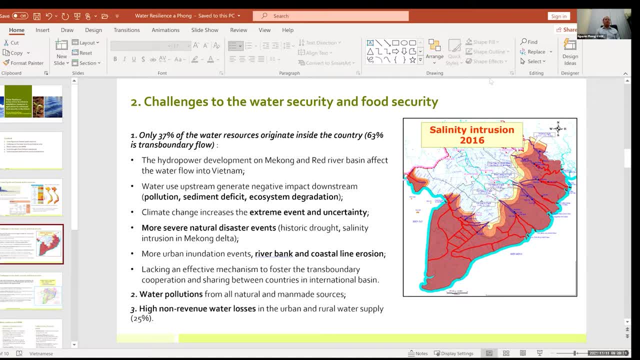 to the extreme. even instead of uncertainty, It also creating more sub-nature disaster. even So, historic droughts appear. The salinity region in Mekong Delta is increasing in recent years, And also more urban actually increase Diversification. 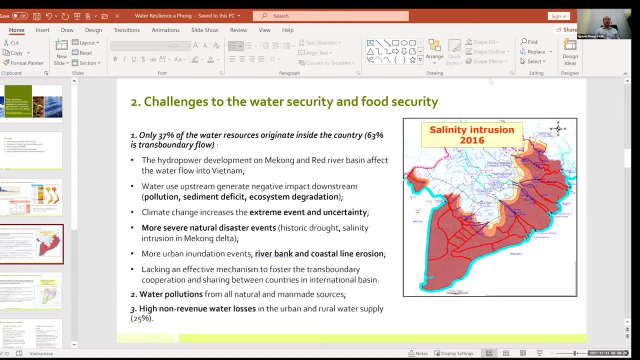 inundation event, river bank and coastline erosion is happening more and more seriously. So I think it's an effective mechanism to foster strong boundary cooperation by sharing the data, sharing the information in the country, in the basins. The second one is water. pollution also creates very negative impact to the agricultural production. 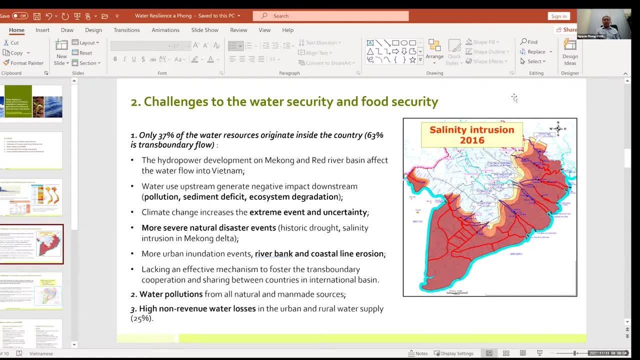 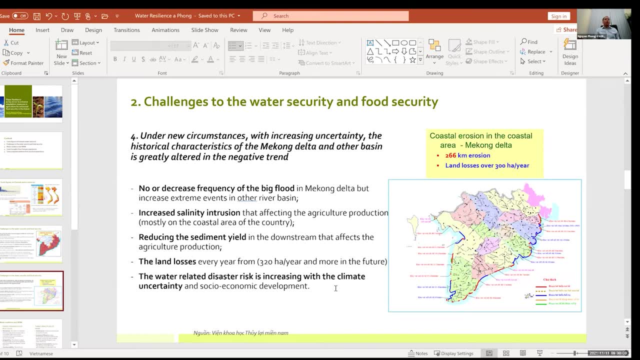 and the high non-revenue water losses in the urban and rural water supply is also increasing. And the fourth one is under new circumstances with increasing uncertainty, the historic characteristic of the Mekong Delta especially, and other river basin is greatly under in the negative trend. 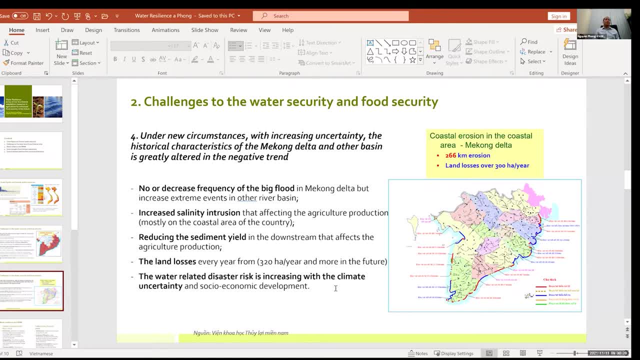 No decreased frequency of the flood in the Mekong River come to the downstream. the increasing sandicity is chosen so that affected agricultural production, mostly on the coastline areas of the countries. So the reducing of sediment is in the downstream. that affected agricultural production as well. 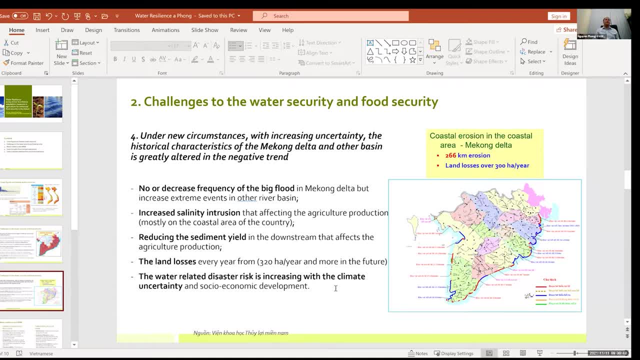 The land losses every year for the sea level rise and also the exploitation of the groundwater for the aquaculture also create very negative impact. So I think it's an effective mechanism. Thank you The Leyvarek series. So, talking a little bit about the water, resilience and IWPIM, Hon's also mentioned a lot of questions. 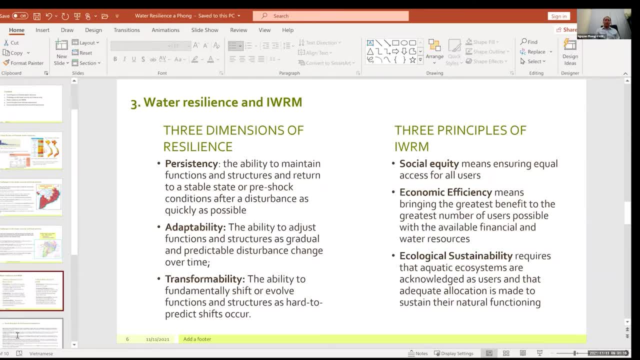 about the IWPIM and how we can change our approach or how we can change thinking to do the IWPIM for food security or the agricultural production. So let's see a three dimension of the region is the persistencies, adaptability, transport abilities. 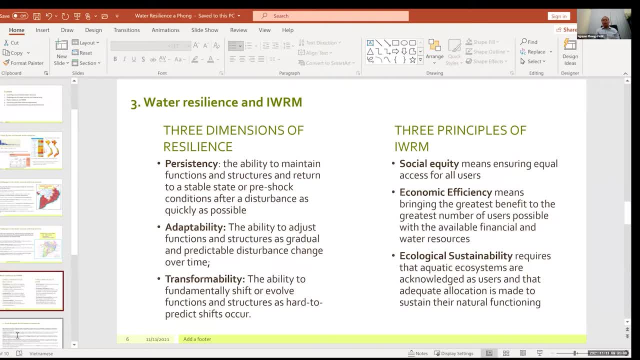 Meanwhile, the three principles I think that Han also mentioned very clear in his presentation, that's, social equity, economic efficiency, ecological sustainability. So I don't want to go more deeply about this, but just remind you a little bit about the linkage. 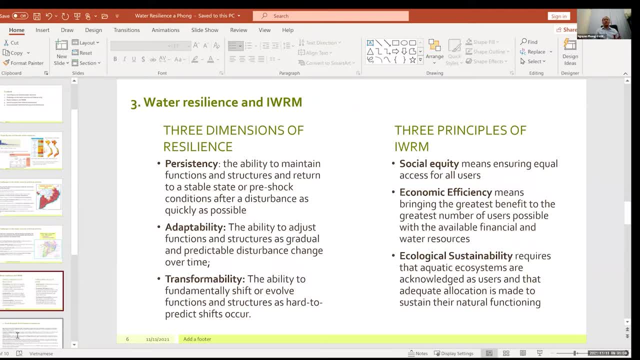 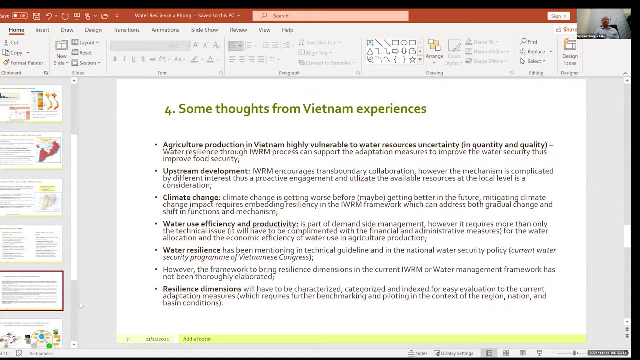 as a connection between three dimension of resilience and the three principle of IWRM. So some thoughts from Vietnam experiences So that for sure that agricultural production in Vietnam is highly valuable to the world: resources and certainty and quantity and quality And upstream development impact. 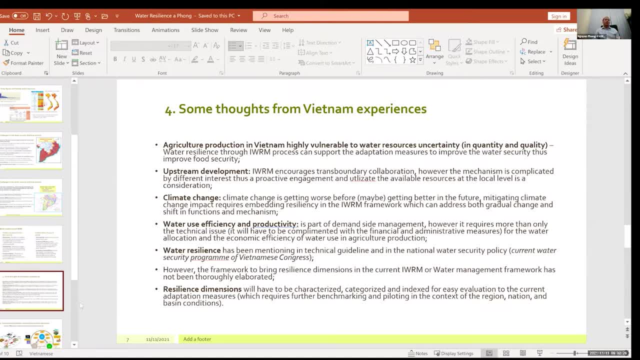 from the upstream also create a lot of the negative impact for the downstream, and IWRM encourage transboundary collaboration mechanisms, And climate change is getting worse- maybe getting better in the future, no one knows. So it's creating a lot of the worry related disaster. 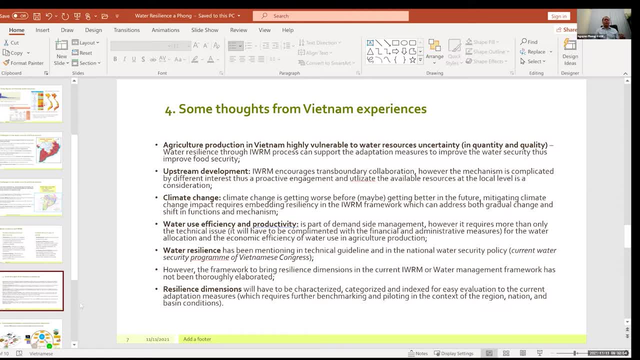 to the agriculture production, So it so requires IWRM from work, need to be changed or need to be having another approach To worry efficiency or water productivities and so need to be increased in the agriculture production. So water resilience is really now is the most interest of our government. 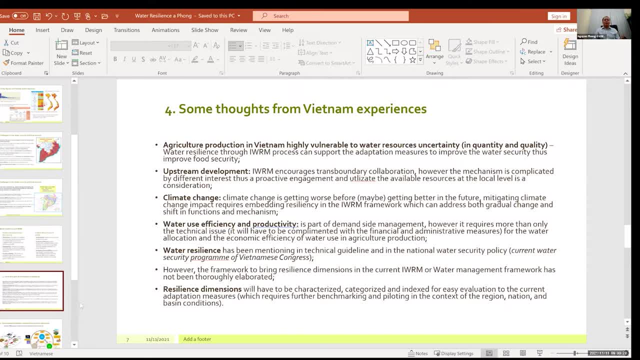 So the national assembly does approve the national assembly does approve the national world security program. So it's also created a lot of measures, adaptation measures for the agriculture, production, and so for security And also the resilience dimension will have to be a character. 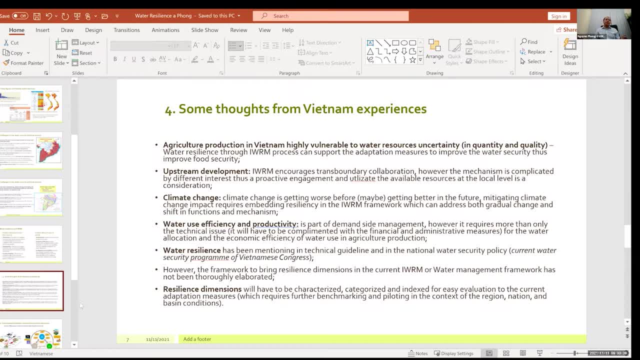 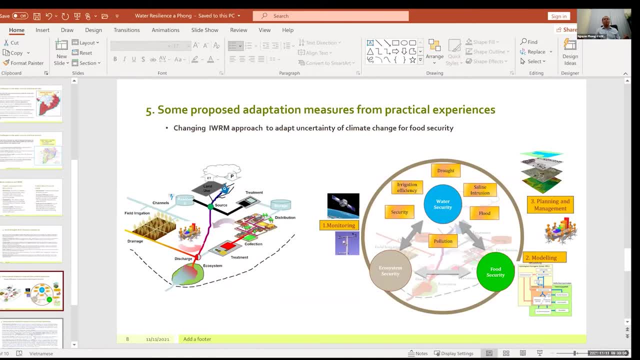 Thank you. Now I come up with some proper adaptation measure from a practical experience. So changing IWRM approach, maybe a solution of the measures to adapt, and certainty of climate change and food security. So we look at the next ecosystem, The next of water security, food security. 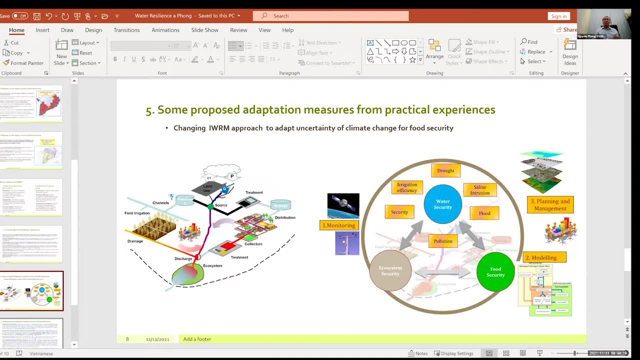 and ecosystem security Now effecting by a lot of to water related records, execution work, water-related disasters, drought, salinity intrusion, flood pollution and also water efficiency. with the use of efficiency, water productivity is unconscious And, in the meantime, indeed. 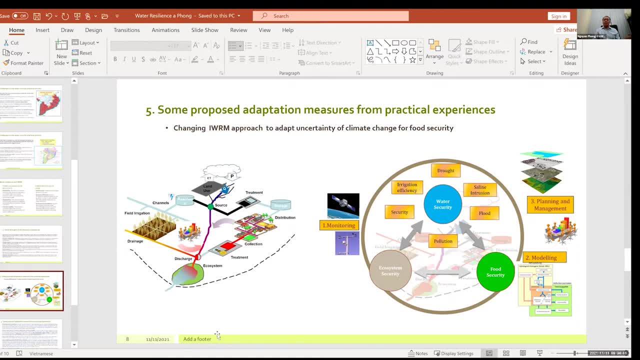 also a lot of the technologies for monitoring, for planning and so for management, using different technologies like decision transformation in terms of the agricultural production, in terms of the disaster warning or forecasting, So optimizing water for agricultures. So look at the restructuring agricultures sectors. 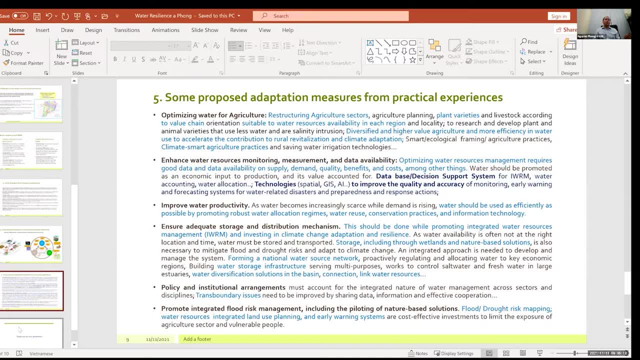 by using the plant variety to the value chain, orientation, Shiftable to water resources, availability into each region, So how much water we can have in the future. So it's a very serious need for the forecasting and water accounting and also diversify in higher value agriculture. 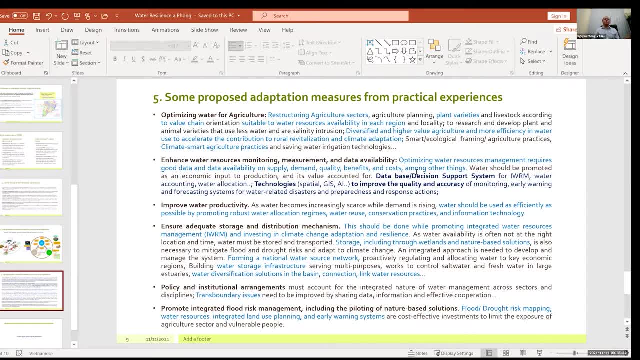 for more efficiency but to use less water. So it's also a very important solution in matters in our country And especially in Mekong Delta. So we can also find the solution for the smart farming, eco-risk farming in our country. 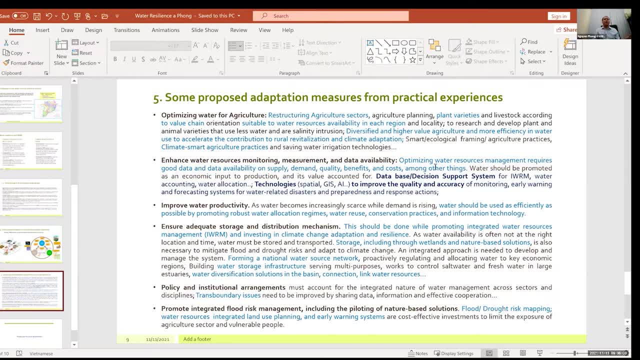 of classmate climate, smart agriculture practices and saving water irrigation technologies. The second one is enhanced water resources monitoring and measurement and data availability, So optimizing water resources managing by using good data and data availability on supply, demand and quality and benefit. 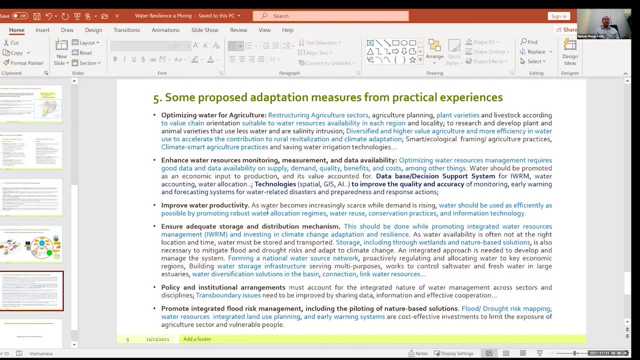 and cost. amongst addressing So, water should be managed and considered as economic input to the production, agriculture production and is value accounted. So data-based decision support system for IWRM water accounting, water correlation, with the support by the technology. 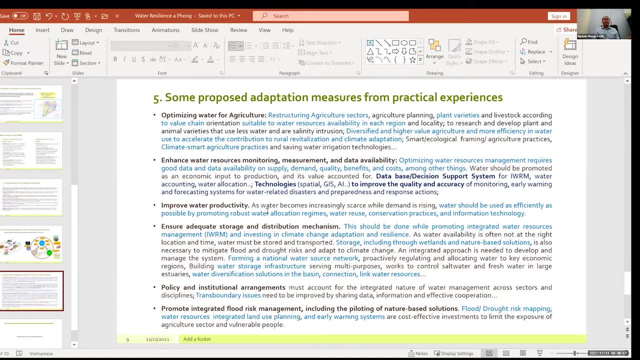 especially on GIS and efficient intelligence and so on to improve the quality and accuracy of water, early warning system over related disaster and also preparedness and respond actions. So improves the water productivity and so very important adaptation measures. 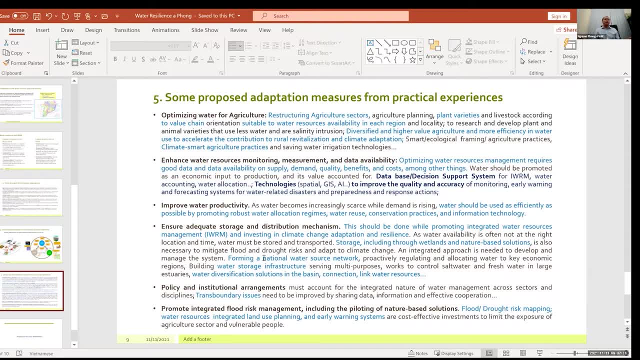 especially in the agriculture production, So ensures it creates storage attribution mechanism. it should be done while promoting the integration, integration with the water resources management, and investing in climate adaptation and resilience, So in our national water security program. so the measures on, so, on that. 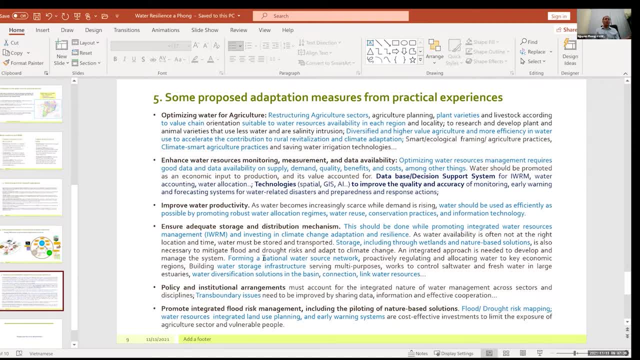 in storage, including through wetland and nature-based solution necessary to mitigate the flood and drought risk. and unintegrated approach to manage the system, So forming a national water sources network for actively regulating and allocating water to the three reasons. 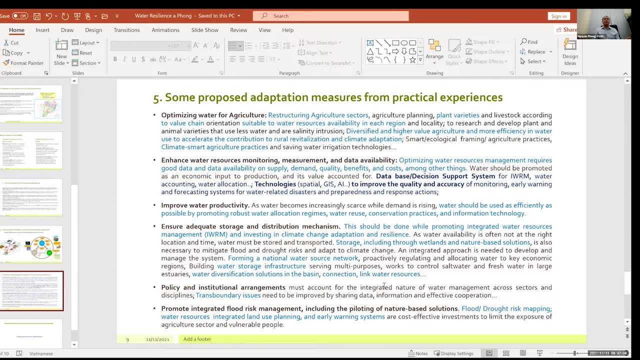 to mirroring the water storage infrastructure serving multi-purposes work to control sour water and fresh water, and estuary and water diversification solution in the basin or connection and link water resources within the basin and the different basins. 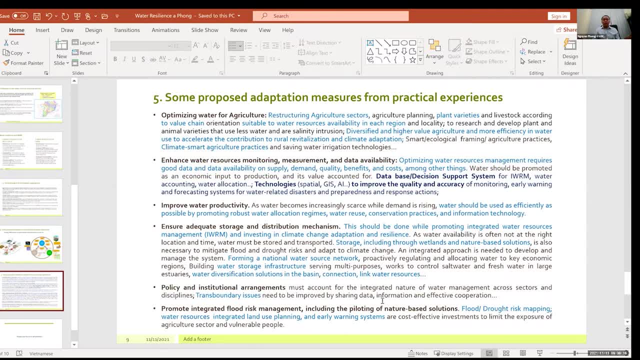 So policies and institutional arrangement also must account for the integrated nature of water resources management. So trans-borderly issues need to be also improved by sharing information and effective cooperation activities and program To promote integrated art-based management. drought management, including piloting a nature-based solution. 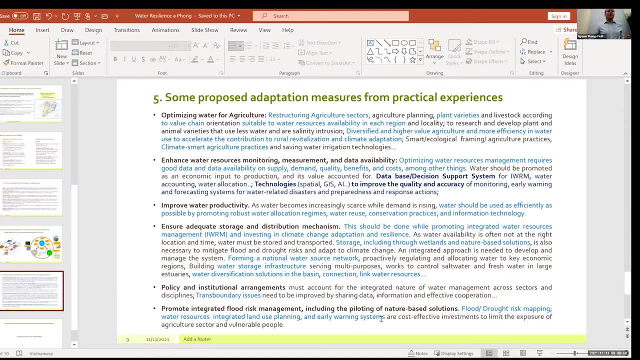 So it should be integrated to the land use planning and early warning system, cost effective investment to the agricultural sectors. So that is some proposed adaptation matters for the practice from the our practice experiences for the agricultural production and also the food security. 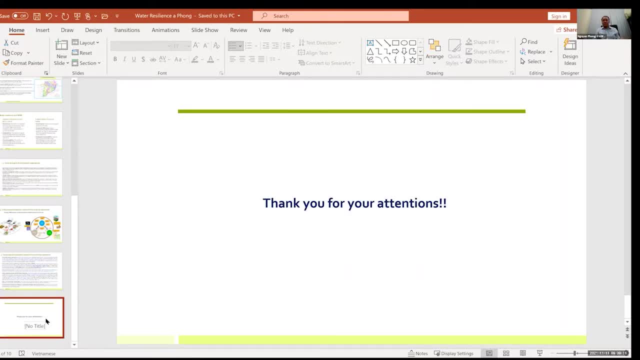 Thank you for your attention. Thank you, Thank you, Dr Fong. Thank you, Thank you, Thank you, Dr Fong. Thank you so much, Dr Fong. There was it covered a lot of ground in that presentation. 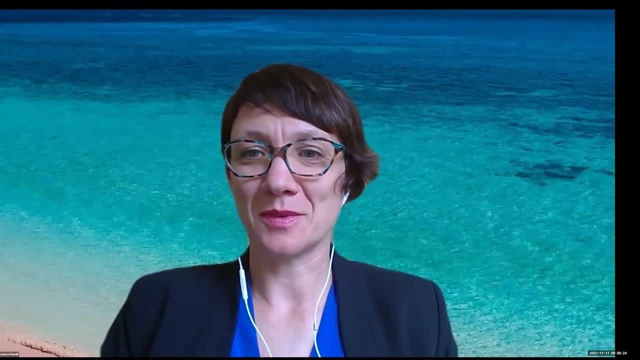 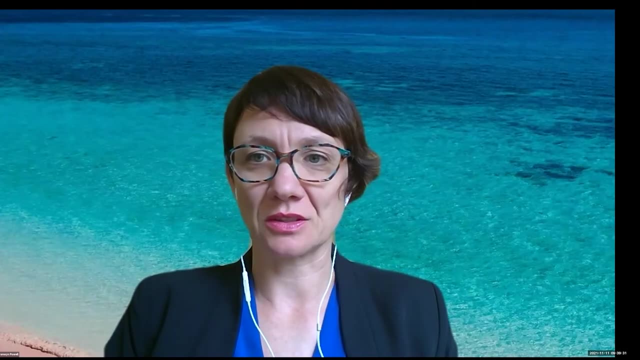 and I think our audience will have some, probably some questions for you. We I think we do have time for a couple of clarifying questions before we move to the panel session. We did receive one for Avi. I'm wondering, Avi, if you could answer that question. 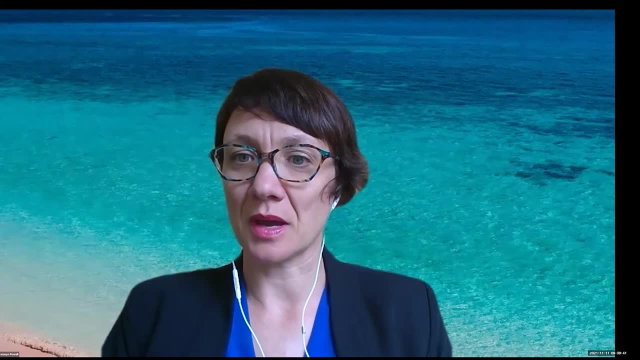 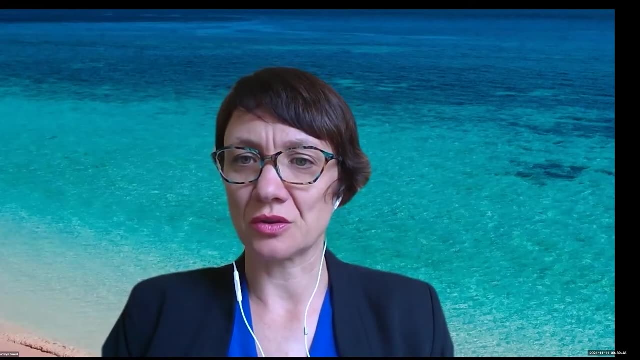 You put it in the chat, but maybe, if you could answer that question, could speak to that a little bit about all of that extensive data that you said that you collected from those thousands of settlements. Did you have that data disaggregated by sex, age and disability? 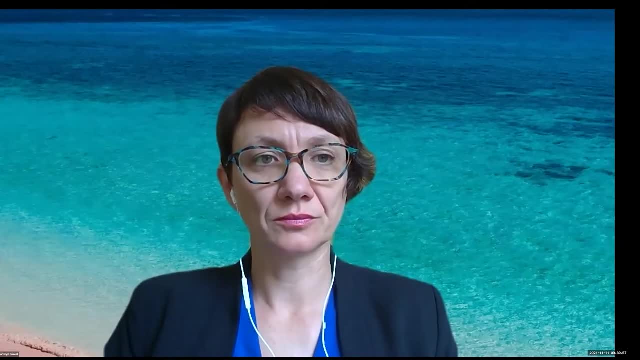 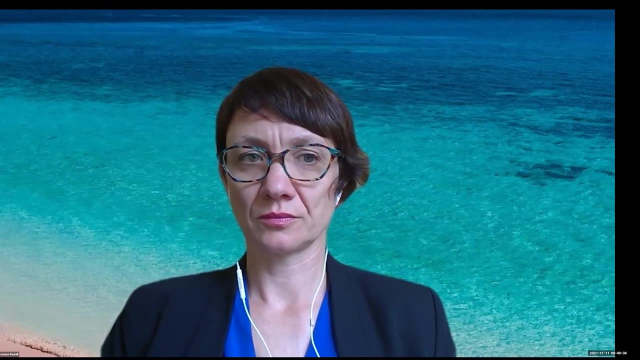 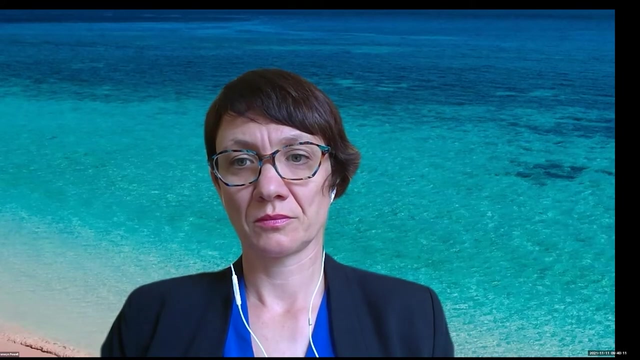 Yeah, thank you, Bronwyn. So yes, as I replied that we have some of the data sets on detailed data sets on community profile, definitely on the population disaggregated by sex, but unfortunately we do not. we hadn't collected on the disability, But what I would take this: 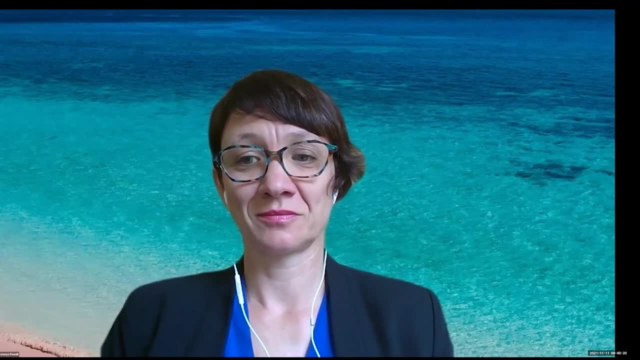 opportunity to quickly mention is that this was a big exercise. all settlements in Laos, urban and rural, 7.2 million sort of spread in this 8,500 settlements In a development balance probably it would be a big project But the million at least $1 million budget. But we actually did this project with zero budget. 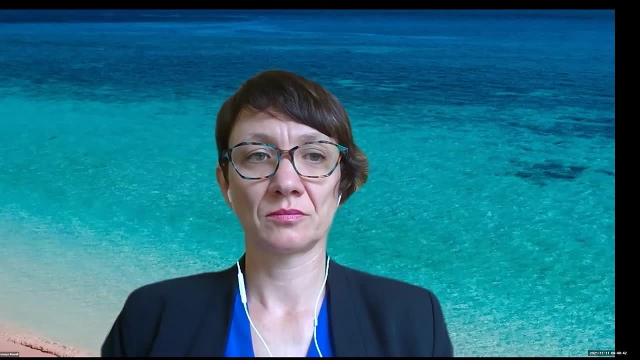 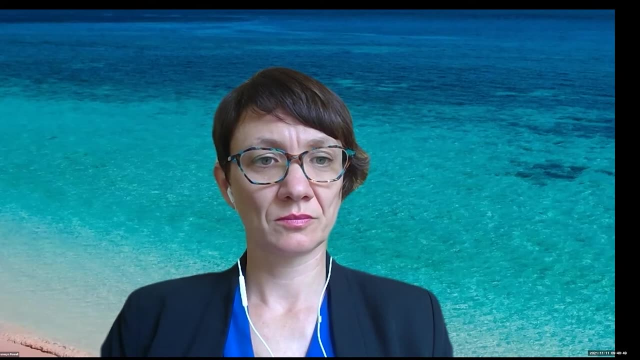 availability, because it was a National Assembly request from the Ministry of Natural Resources and Environment and who then in turn requested you and habitat. of course we had staff who were available to do that work, But I think it also talks of the great leadership when you are. 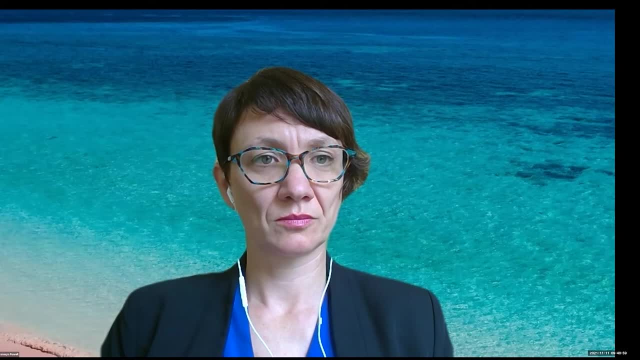 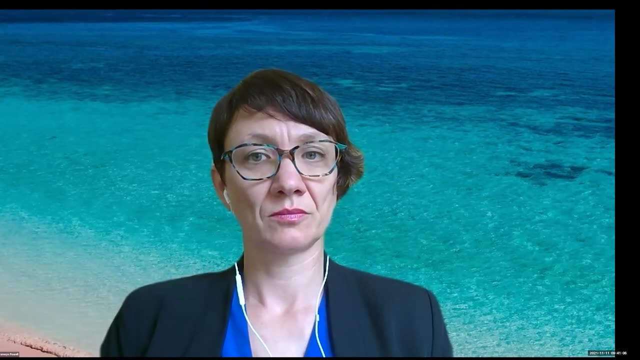 interested. the minister really pushed for. it used all the provincial and the district offices available to collect the data from the settlements. so the whole exercise was done in three months time, which I think this amazing, considering that there are so many challenges that could come. 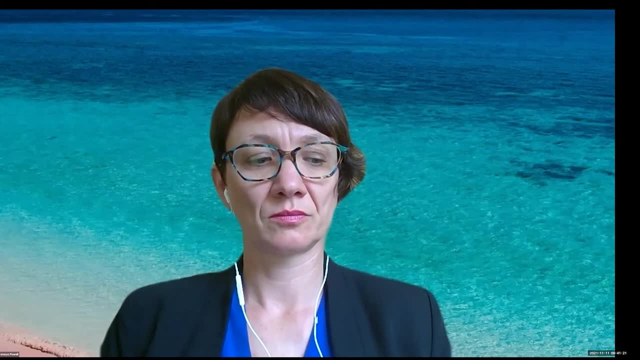 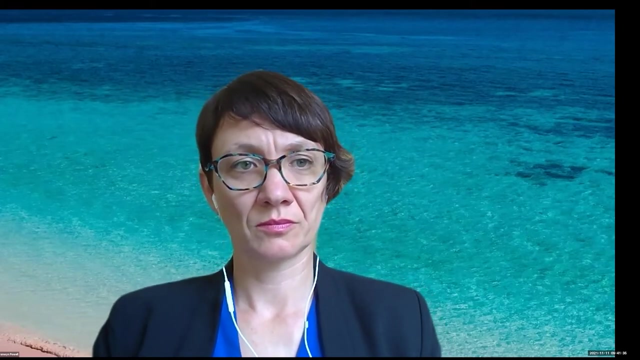 across. so the original national assembly request was for eight provinces, but then we thought that if we had to do, why don't we do for the all 18 provinces? so now we have a great data set available in Laos which can be used for a number of work, that different development. 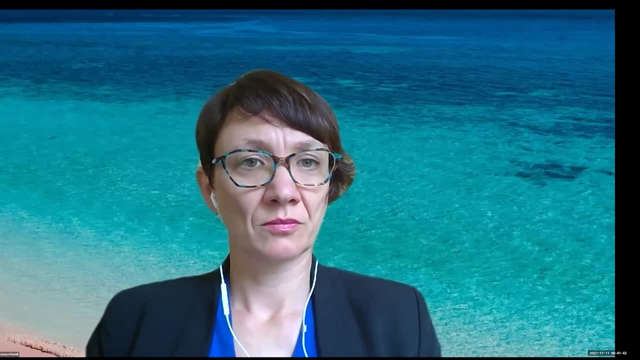 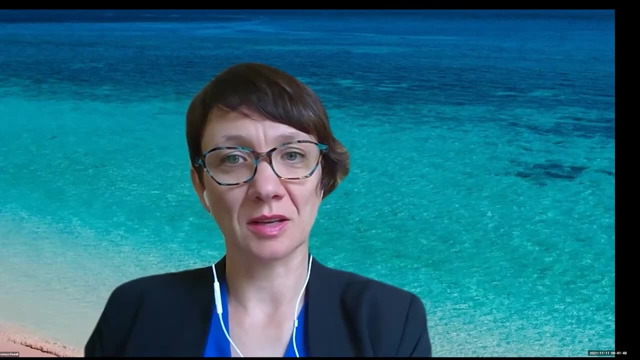 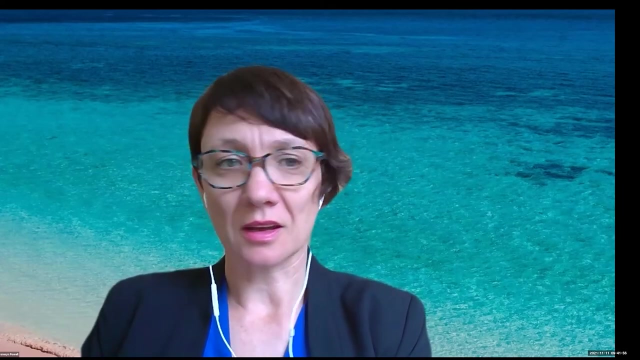 agencies are currently engaged in. yeah, thank you. yeah, thank you, Avi. I mean that's amazing rapidity of a project at that scale and a great example of it being embedded in the government systems, and replicable. so thank you for that further information. now. we also did have a 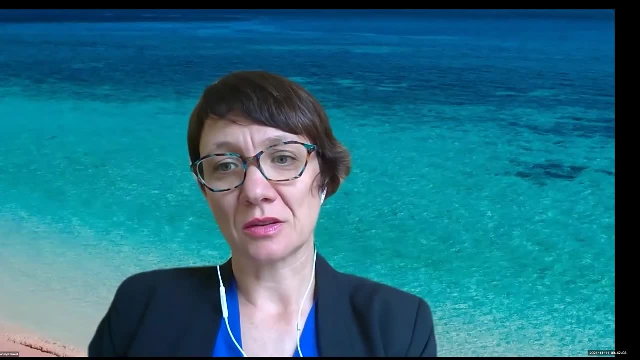 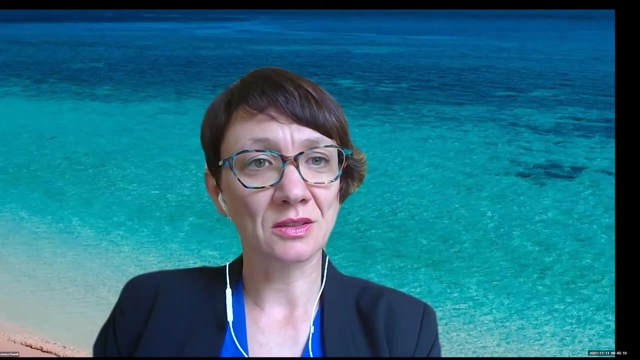 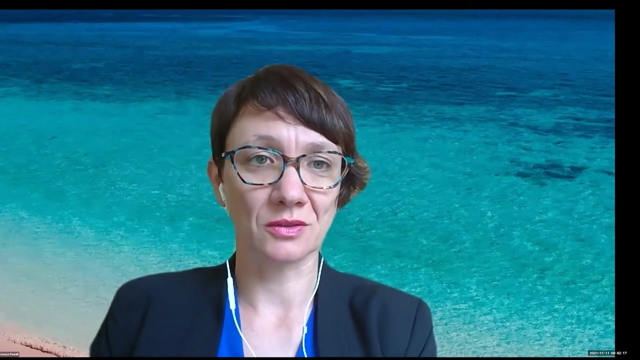 question for Dr Phuong. it's just, it's quite a broad one, but perhaps you could just point out the question is to do with why Vietnam's water resources are insecure or not as secure as previously, and if you could just highlight what you would see as the key issues, because 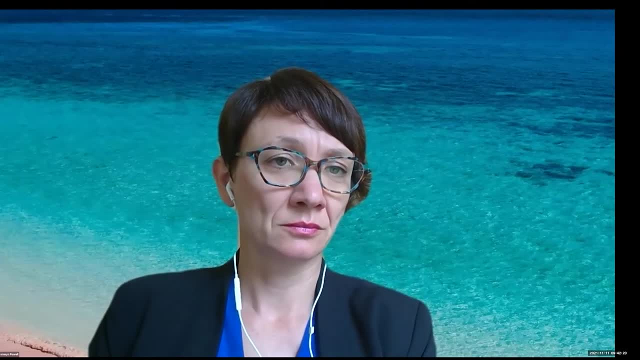 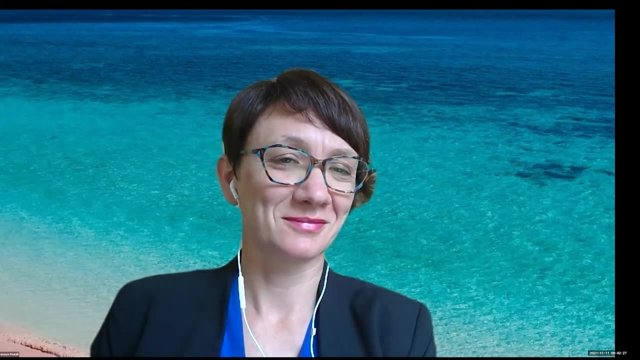 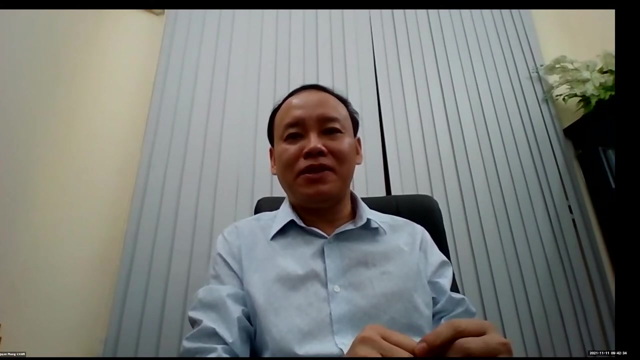 obviously there would be many okay. so actually I think that we just prepare- I also the member of the group- to prepare the national security program. so that would be a very, a lot of reason why Vietnam is insecure in world resources. so I mentioned at the beginning that more than 60 percent of the world resources come from the 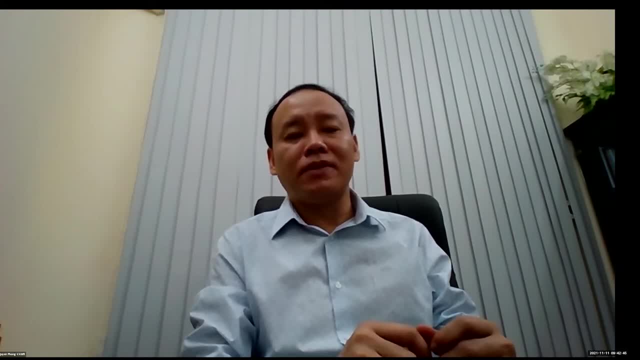 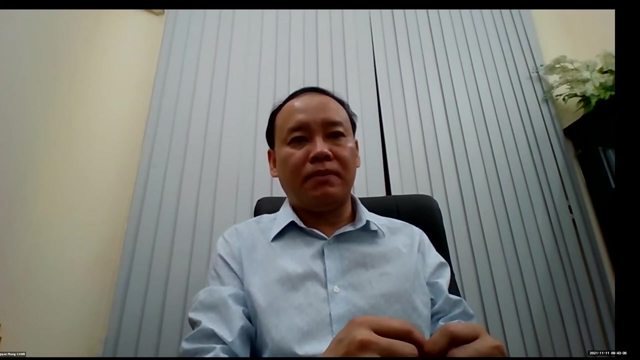 outside, so only 30 percent. the 37 percent from the inside come from the inside of Vietnam. the second one is we are really affected by the, by the, by the disaster related with world related disasters. so more and more uncertainty and more and more extreme by the, by the climate change. 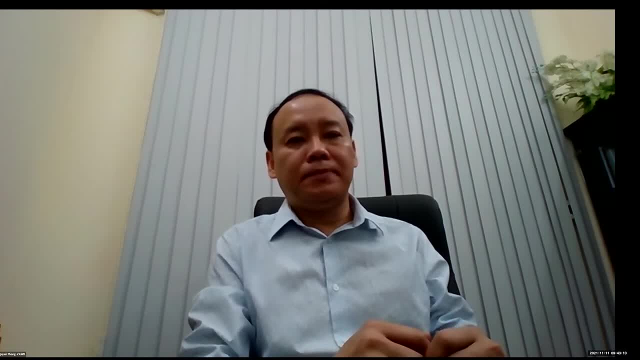 by the climate change impact. the third one is the. the third one is also the groundwater so affected by the exploit exploring the, the groundwater for the other countries, for the, also aquaculture, so it's also very, very, very seriously impact the. the fourth one is the. 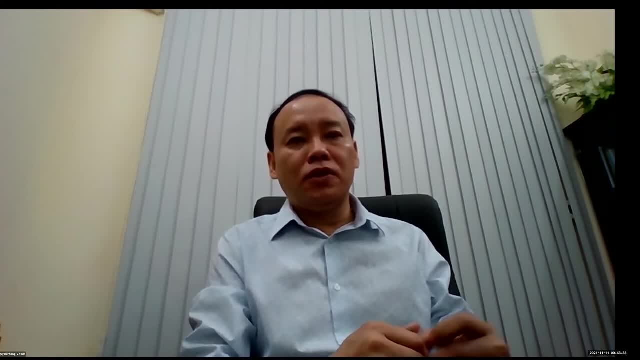 the irrigation system and also the, the water dam is decreasing, so the efficiencies of the irrigation system and and quite low. so we need a lot of effort to, to, to, to improve, improve the, the, the irrigation system. and the fifth one is also important- is a participation of the water. 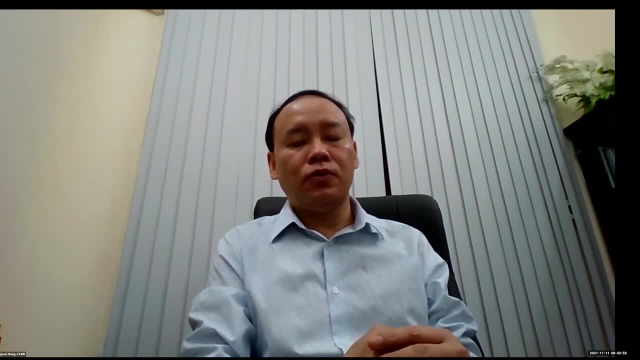 user groups to to help to to reduce the water losses in the urban and rural areas. so a lot of and also the. the next thing also the, the regression of the, the price of quality, so it's really impacted the uh, to the, the world resources inside of vietnam. and the next reason also could be uh could be important reasons is: 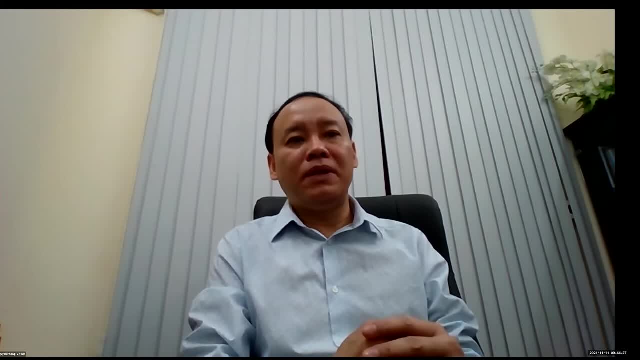 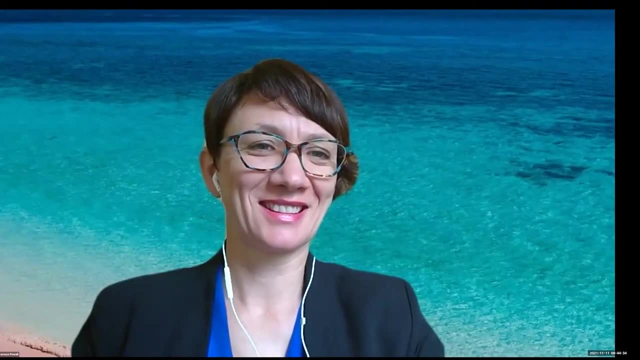 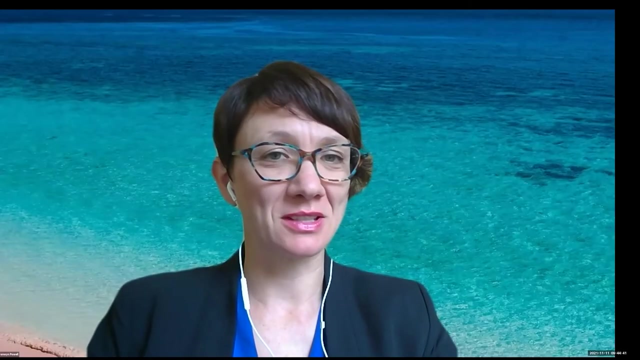 uh, the sharing the water, different the basin, different region, so a lot of of things to be shared. so you can contact me directly, then you can. uh, we can talk more about this. thank you, dr fong. that was comprehensive answer and, as i've guessed, many, many reasons for lack of security. 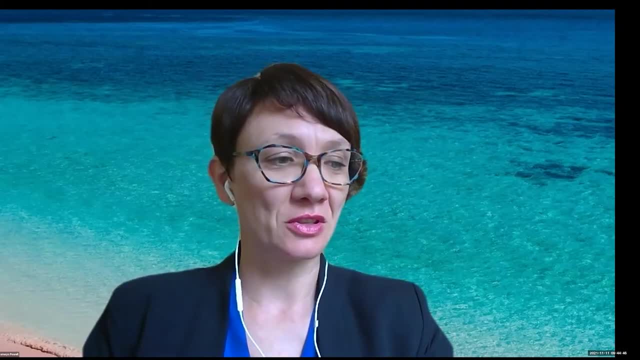 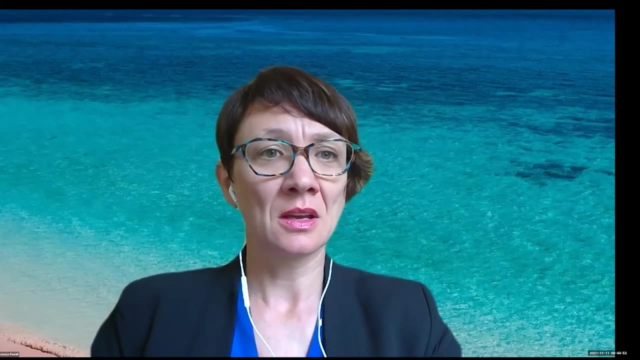 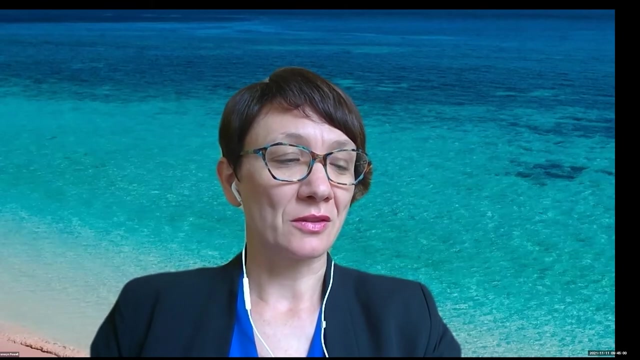 in water. um, so now i'd like to take the opportunity to introduce our panelists. panelists, if you could please turn your cameras on, and also speakers, if you could have your cameras on. that would be. first. i'd like to introduce dr sharon taylor. so sharon taylor is working for the philippine. 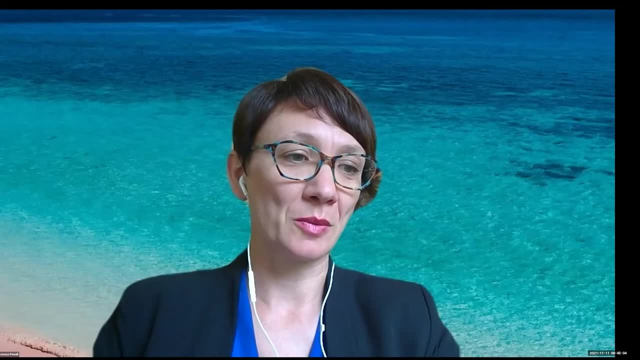 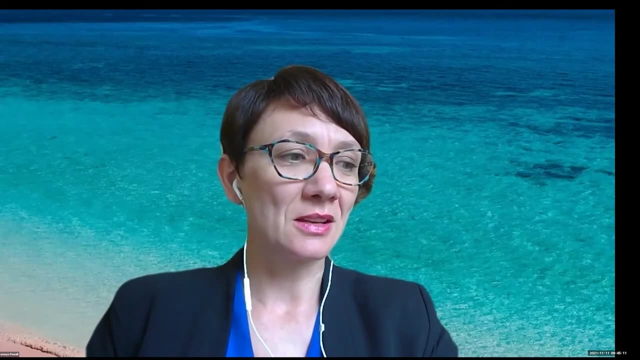 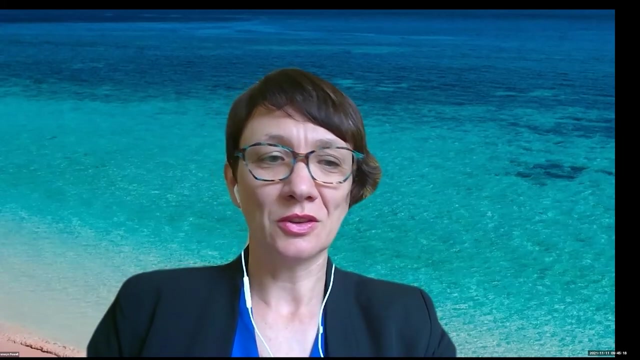 rural reconstruction movement, which is a local ngo implementing the program with oxfam called building resilient urban communities in asia, and is joining us, i think, from the philippines, of course, and also we have dr sutat wesakul, who is from the, who is the director- sorry- of the hydroinformatics. 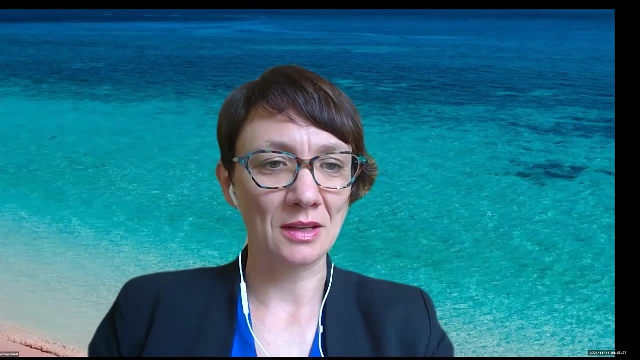 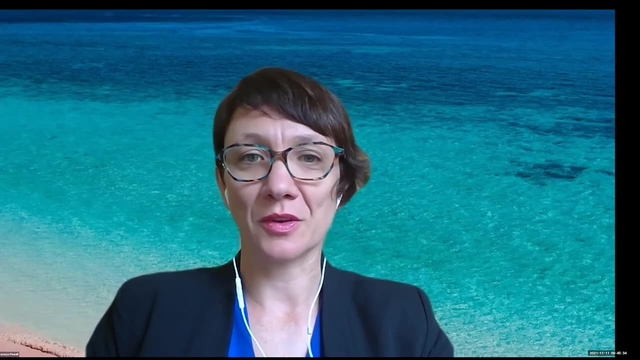 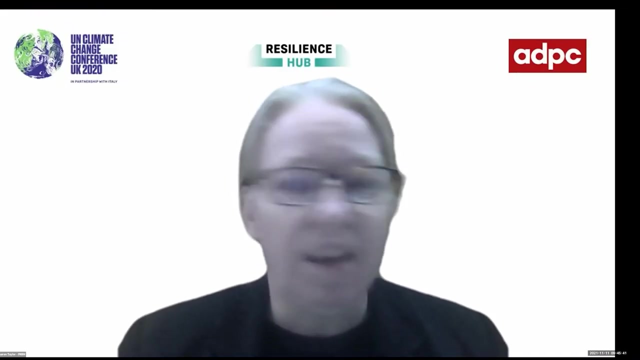 institute in thailand. so thank you both for joining us. i might just start with: uh you, sharon, and your thoughts and impressions and from those presentations and how they relate to your urban resilience program. yeah, um, thank you, roman, and thank you to all the speakers for very comprehensive 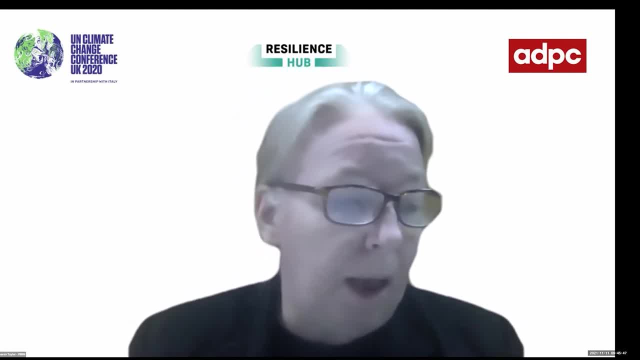 outlines of the issues with um, iwrm as it relates to the supply, the distribution and the impact on food security, and i think the iwrm and the iwrm framework It is an infrastructure, that the iwrm has a very comprehensive structure, and so i think that this is an important project to be thinking about and also in terms of 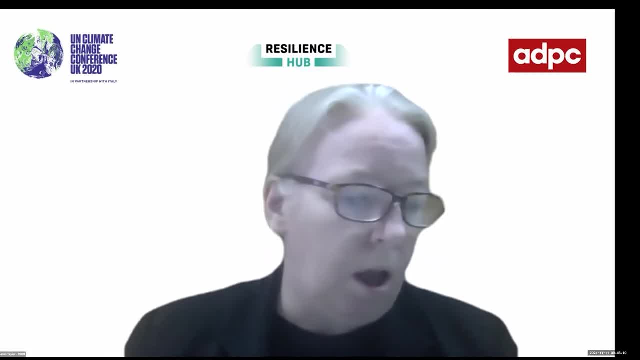 the, the workingility and the purity that that presents as well. that was very comprehensive in terms of the key lessons. in terms of how does it relate to urban resilience projects that i've been involved with here in the philippines? yeah, it's in sync completely. um other issues we need to look at and 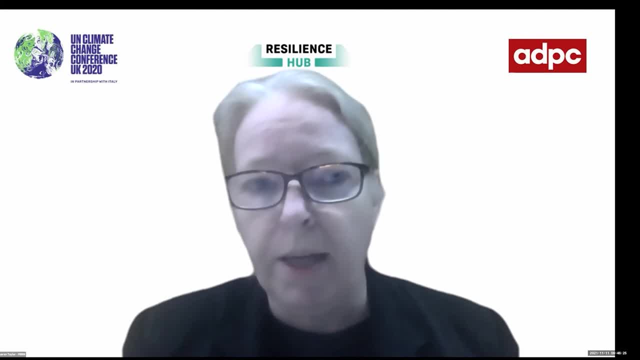 we've looked at in terms of just calculating what is the existing supply and demand that has to be brought into any iwrm framework. there's a lot of work to do in the iwrm framework to have a bit of a. Yes, you've got the population increase, but you've also got to look at the daily changes between nighttime, daytime, as workers come into urban areas, applying demand for water as well. 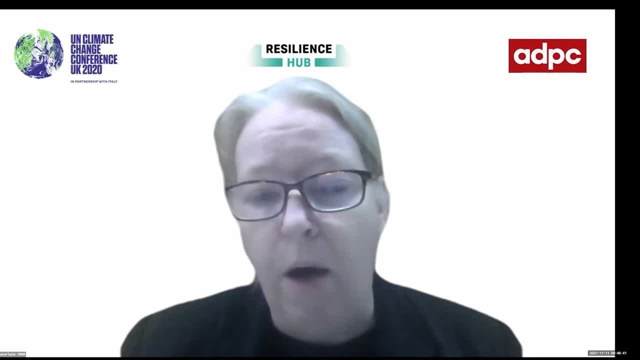 I think in terms of how urbanization is impacting on the uptake of IWRM and especially in the context of climate change, climate-related disasters, the hydrometeorological impacts, I think we need to address the existing challenges with the uptake, first in terms of governance. 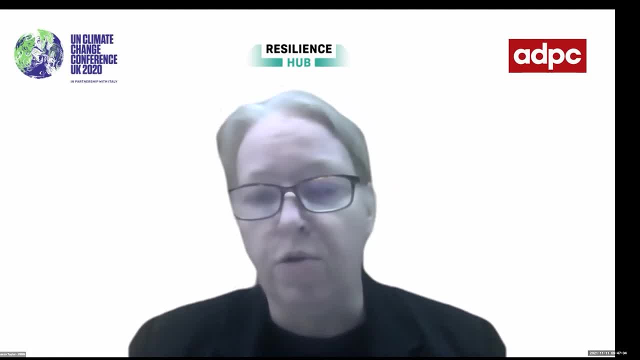 Especially in the Philippines and I know in other countries, different government agencies have different responsibilities When it comes to water management, whether it's supply distribution, planning, etc. we need to bring into that system the agencies involved in the forecasting: the climate change scenarios, the flood monitoring and forecasting climate change commission. all of these need to be able to coordinate, collaborate for the equitable. 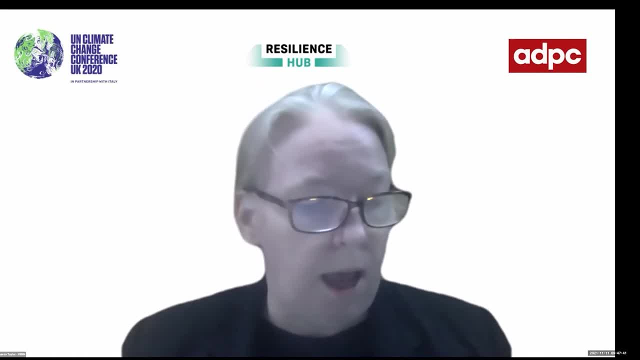 management. IWRM Private sector is also involved heavily here in the Philippines in terms of distribution, in terms of treatment and filtration of water resources. One thing that is lacking, and that was highlighted by Avi's presentation, is the community focus. So that was very good to see the community assessments that were done, which we've done in our communities as well. 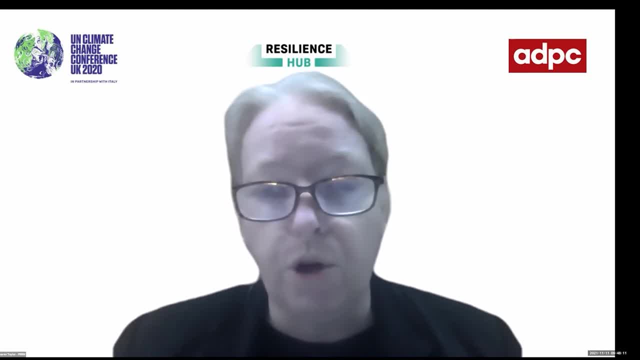 to look at a gender responsive, socially inclusive elements to IWRM. So working through vulnerability and adaptation assessments, bringing in the climate change scenarios and how they impact on the challenges already felt when it comes to water supply and usage for residential use, commercial use, food security- all those factors 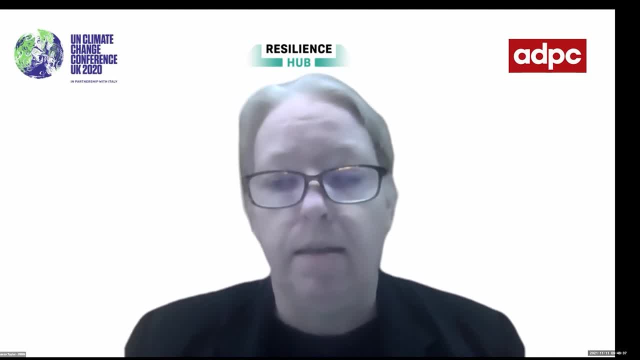 And then basically that can be brought in to update the IWRM, The IWRM systems in place. So basically, address existing challenges, bring in the community voice into the list of stakeholders responsible for the implementation of IWRM, bringing the climate change scenarios. 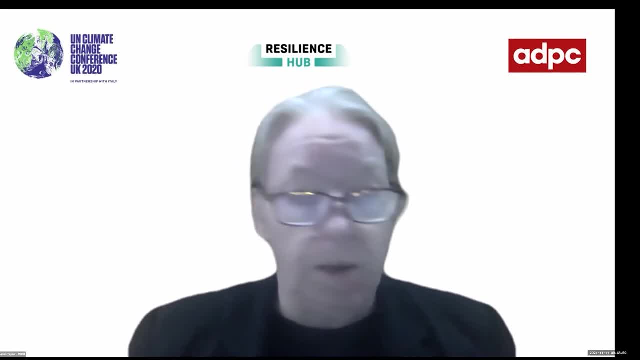 And looking at the impact assessment matrices when it comes to climate change scenarios and improving the governance In terms of urban planning which I think was brought in- and by the last year, The last presenter as well- to address the competing needs for the water resource, We also have to look at how do we sustain the water source as well in an urban environment, or are we reliant on? 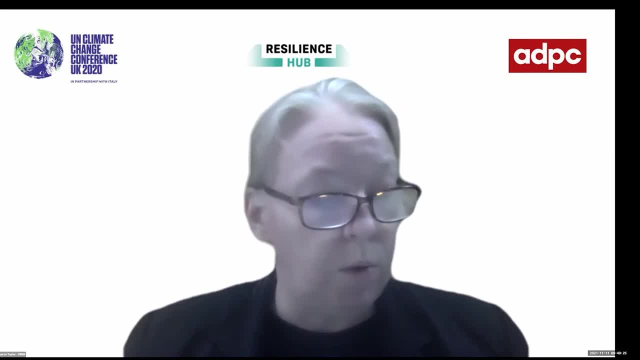 looking at the river basin management as a whole, which I think was also brought up by Avi as well in his presentation. So it's very, very complex when you get into the urban setting. It's complex in a rural setting. how much more so. 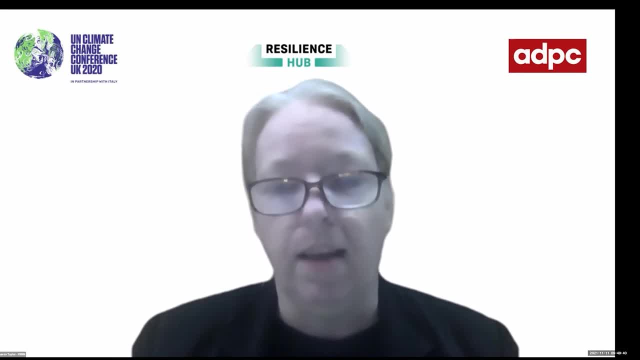 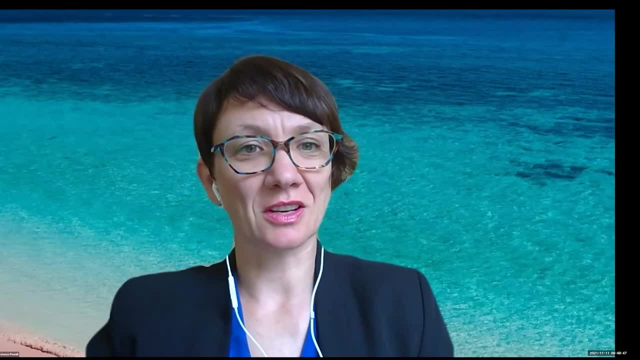 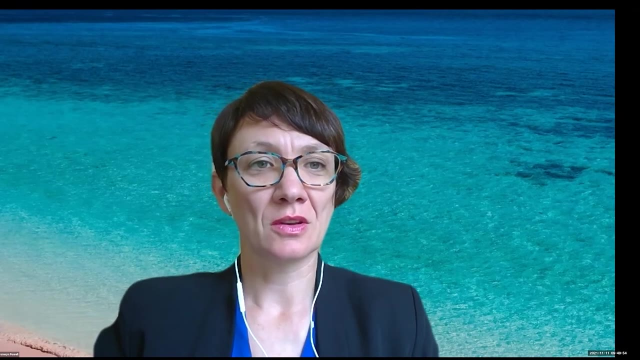 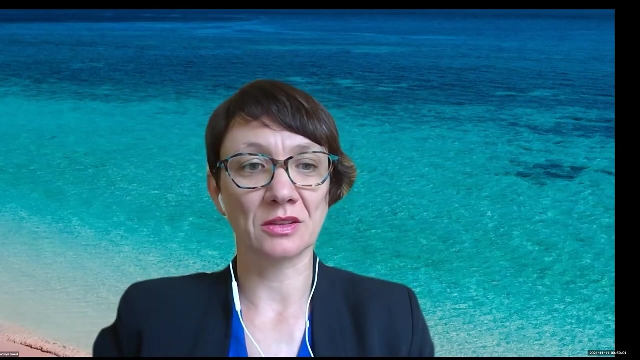 The challenges of urbanization and then climate change on top of that. Thank you very much. Thank you so much for those insights, Sharon. All excellent points And, as you say, very complicated. Now, if we could go to you, Dr Suttat, on your reaction or views and responses to the presentations and what you think hydro informatics can bring to the table, 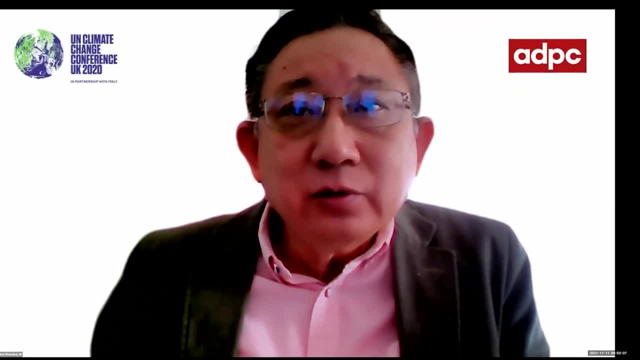 I think they have a presentation to have a good presentation. I think they have a presentation, they have a good presentation. they have a good presentation, they have a good representation. but I would like to add the system that if you have the climate change, 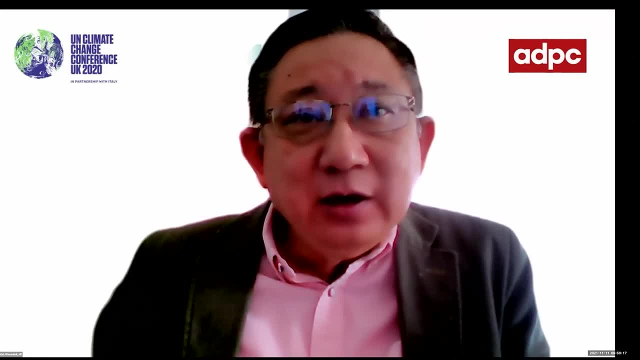 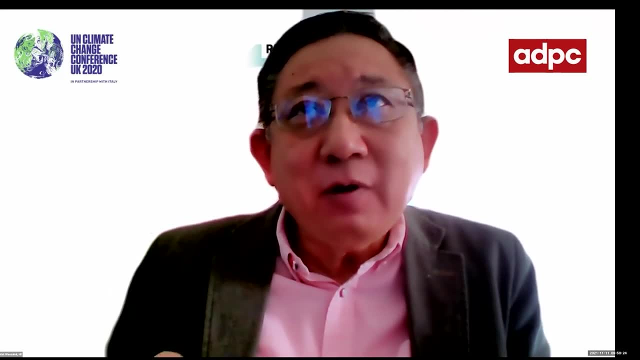 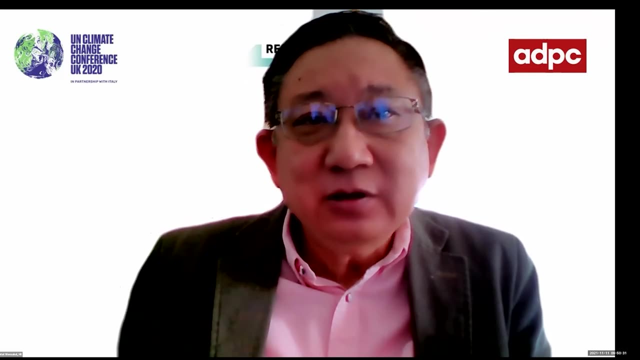 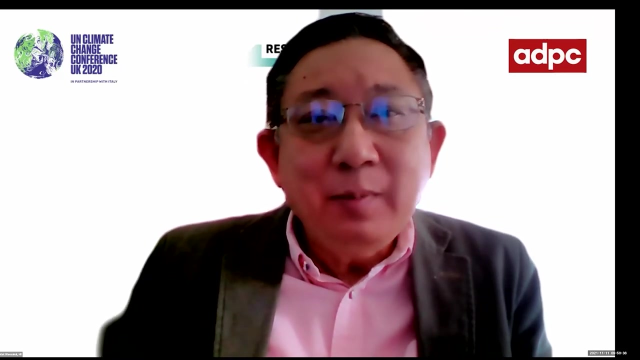 it deals with uncertainty and variability. Therefore, the present IWIN do not have include this directly. Therefore, I would like to propose that if you have the robustness system linked to the IWIN so that you can test the solutions before implement, you can test the variability of the climate and then the robustness system will show the degree of 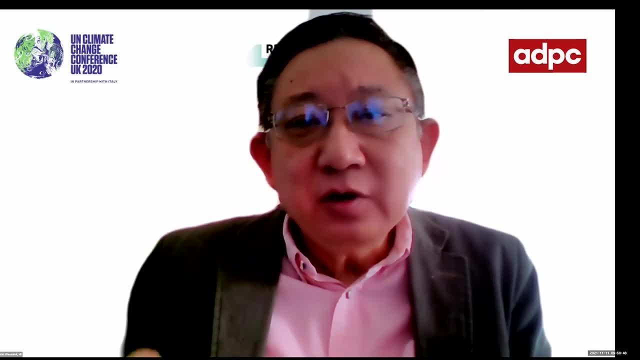 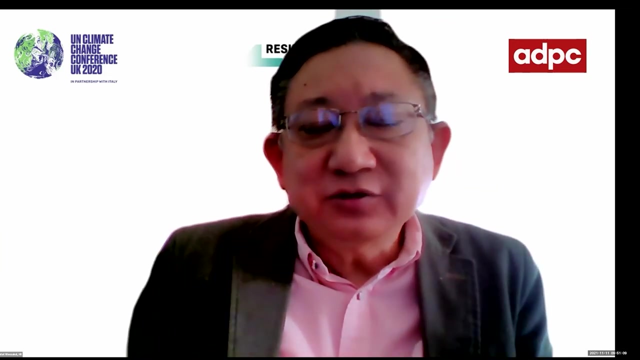 resilience. The robustness system will show some of the possible solutions which can link to multi-criteria and multi-function of the IWIN. So that will complete the system. That is for my comment- Listen to the speaker- which they have implied already. 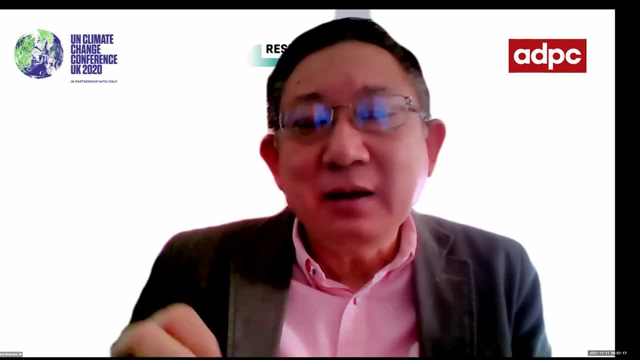 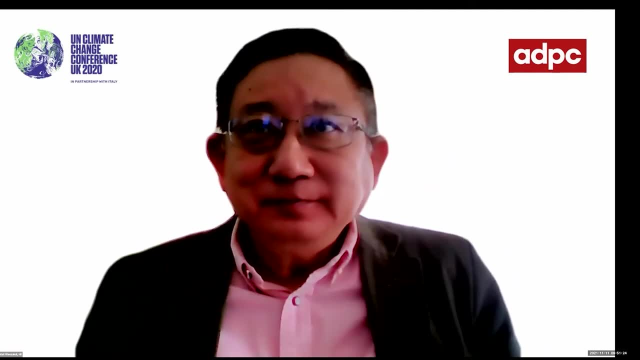 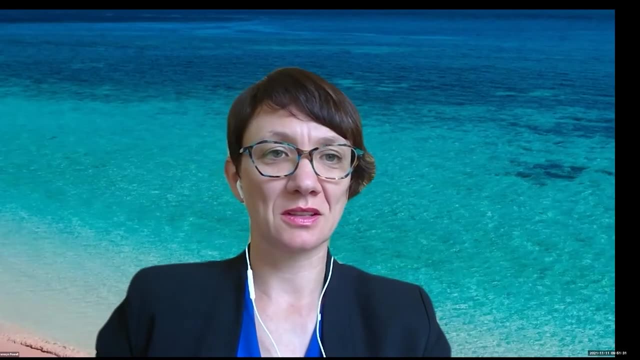 but I would like to wrap up into the system and put on the top of the existing IWINs. Yeah, thank you for that, Dr Sudhat. I mean we're dealing with quite big systems, Obviously the agricultural system- we've seen the detail issues arising there in Vietnam- and of course also 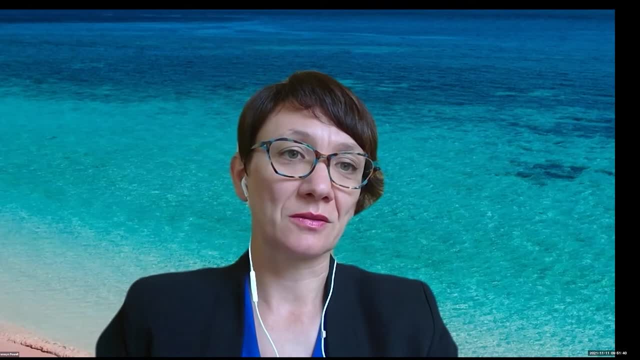 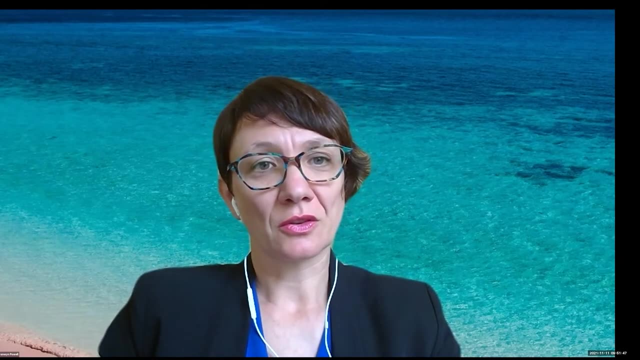 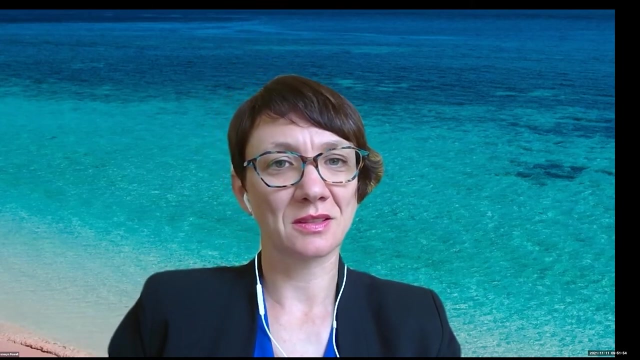 in Laos, the extensive and data collection around urban issues. I wonder if we could go to the panel and just ask the question. I mean, how do you see IWRM in this space? Is it still fit for purpose kind of framework You've just raised, Dr Sudhat? 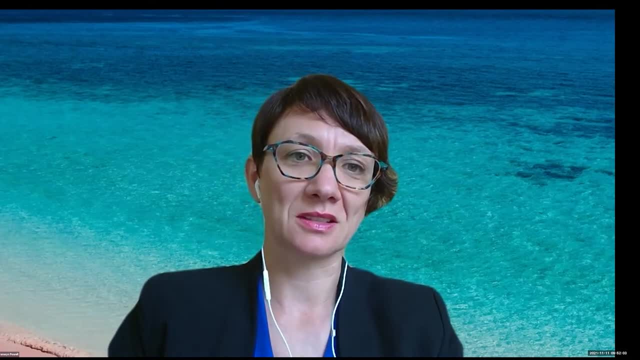 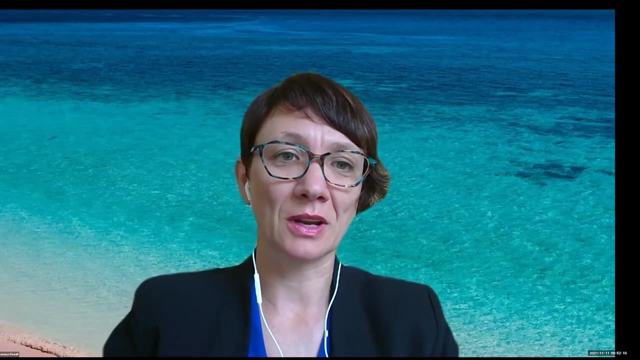 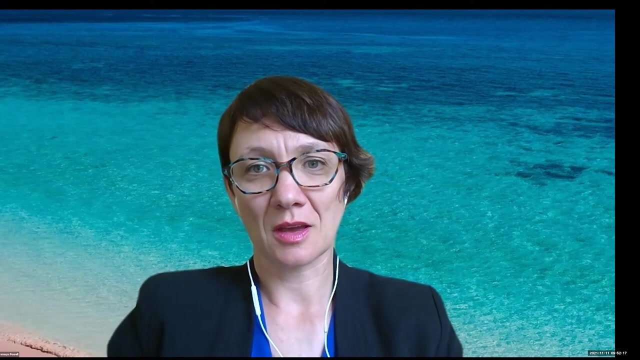 that it doesn't have the robustness, it doesn't have that ability to test uncertainty and kind of beyond what has it been experienced in the historical record. How can we adapt IWRM? Do we think it's the right framework to move us forward? Maybe I'll start with you, Hans. 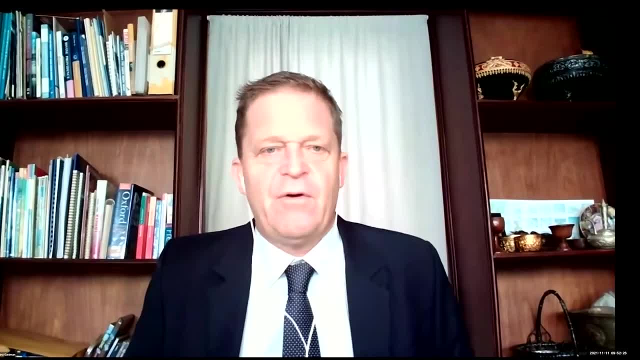 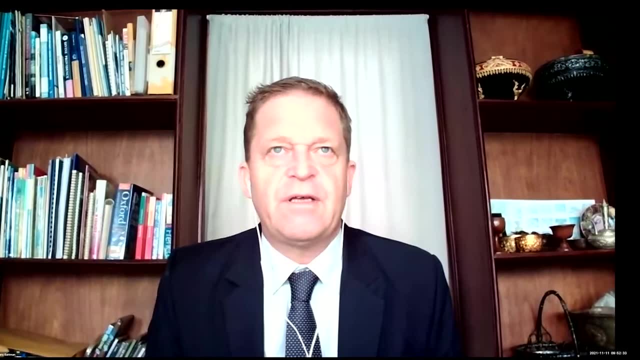 Oh, thank you. I think I can only echo what Sudhat was touching upon in terms of working on tweaking the system, perhaps, but also looking at some of the fundamentals in order to be able to deal with the directional change predicted by climate change. but perhaps, 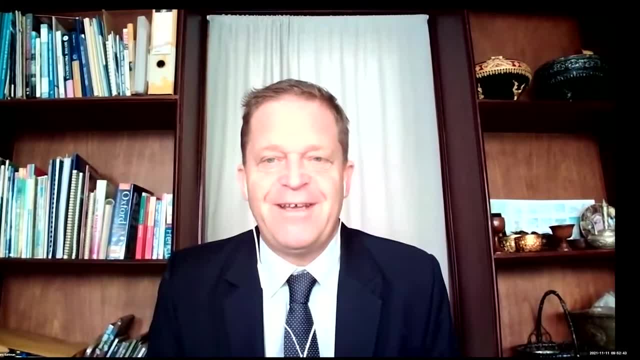 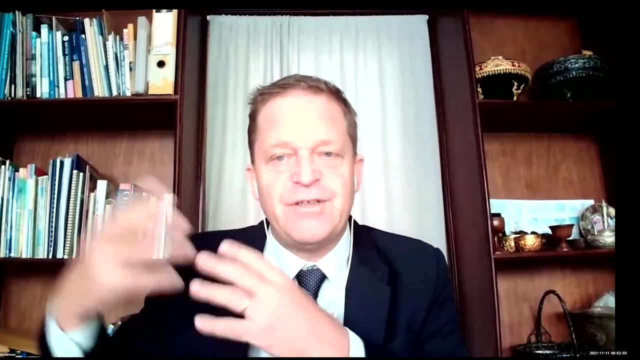 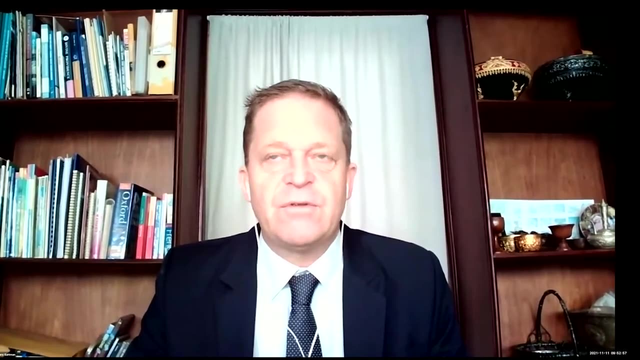 more importantly, the uncertainties that are introduced, as I touched upon historical facts that we tend to use now, or prediction based on global models, et cetera, and downscaling. So how to be able to deal with that without ending up with so much uncertainty that it's difficult for. 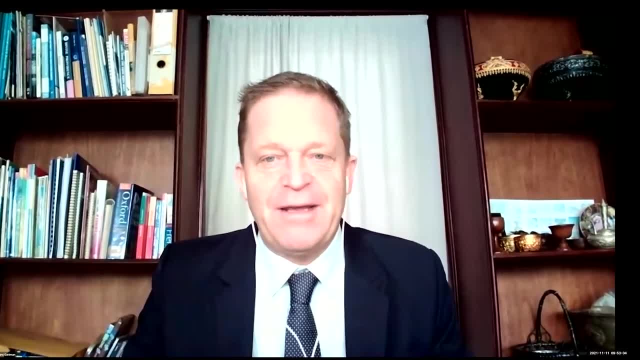 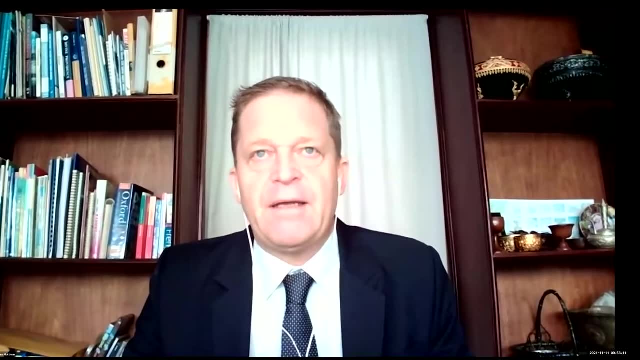 people to have facts about it, To have faith in it and apply it. At the same time, I think what Sharon was raising in terms of, yes, there's a lot of complexity, but there is also a lot of opportunity- by more effectively, 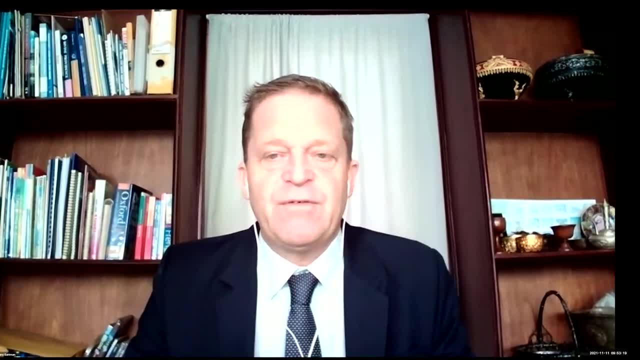 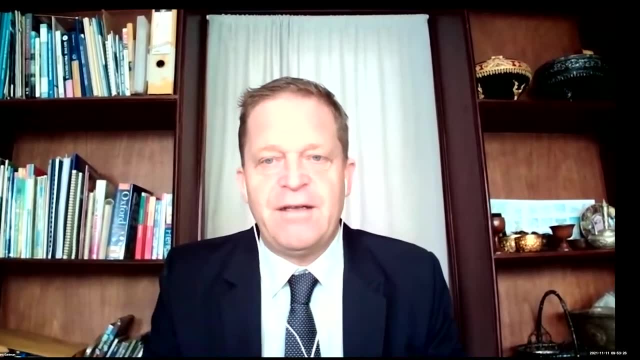 and efficiently perhaps engage a number of stakeholders and get them closer together, so to say. If the sort of science behind it can work more closely with the users and such, then perhaps there's better understanding on what's going to happen in the future. So I think that's. 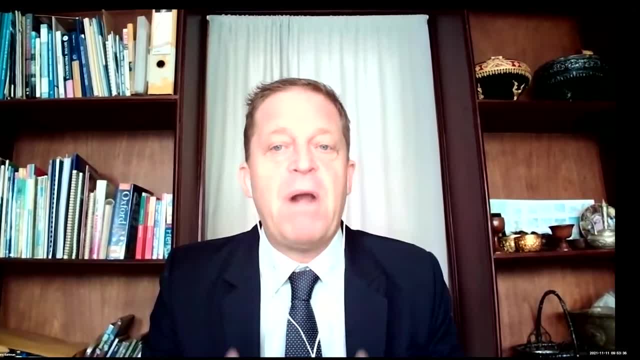 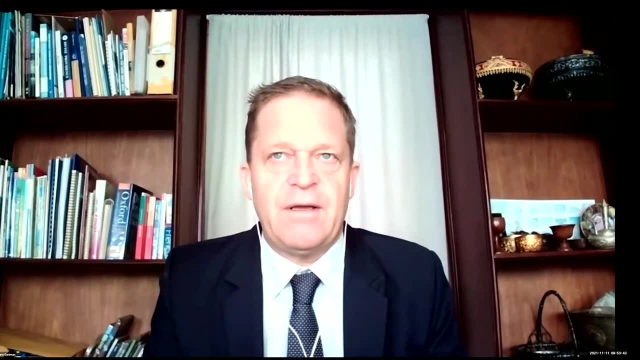 what the uncertainties and variabilities imply in terms of adaptiveness, et cetera. So I think there's a lot of work. There is, in my view, a need to revisit parts of it. It doesn't mean that we throw everything out with a bath, and maybe with a bathwater, so to say, but certainly 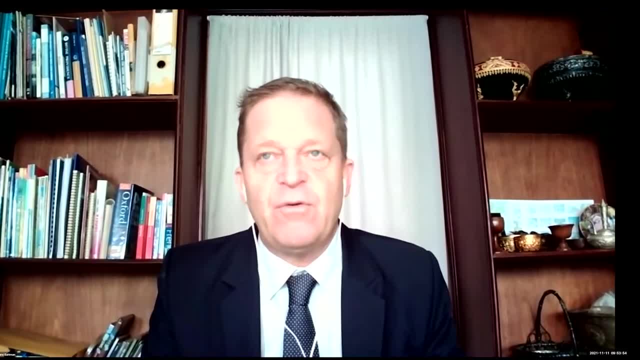 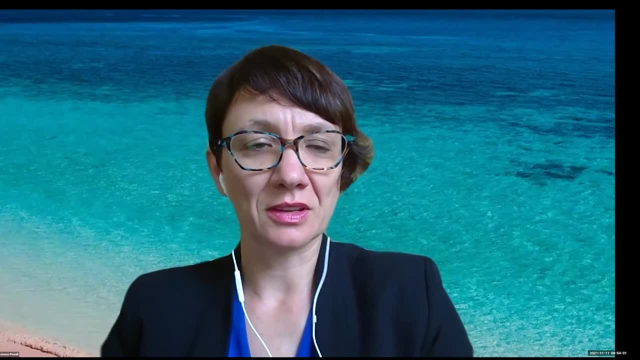 looking into some of the key elements that may not be as relevant or accurate any longer. Thank you, Yeah, thank you. I guess I'd be interested to go to our urban colleagues, Avi and Sharon and ask: have you included IWRM as part of your program? Is it something that is? 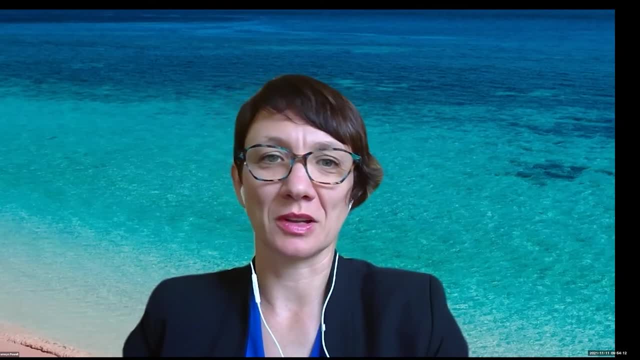 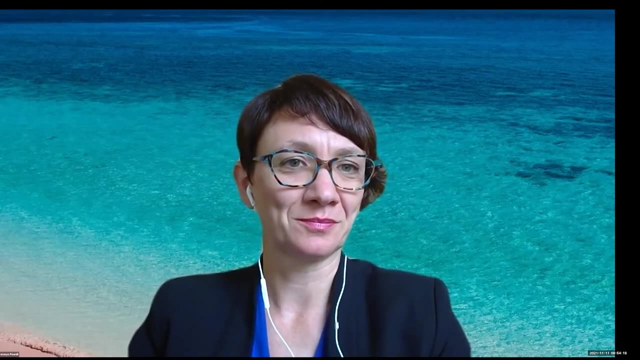 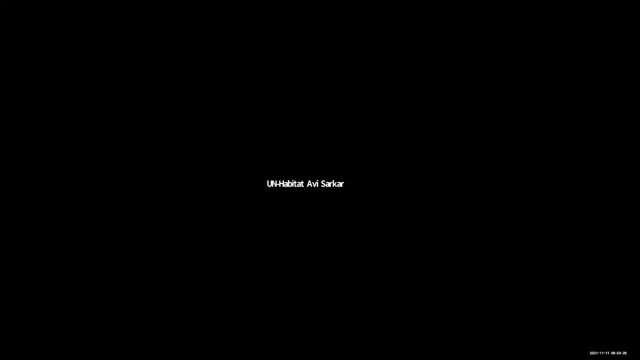 embedded in what you're doing, or is this something that would be applied over the top? I'm interested to see how much it actually comes up in the programs you're implementing. Maybe start with Avi. Thank you, Bronwyn. Yeah, IWRM is sort of a bread and butter of a UN habitat. 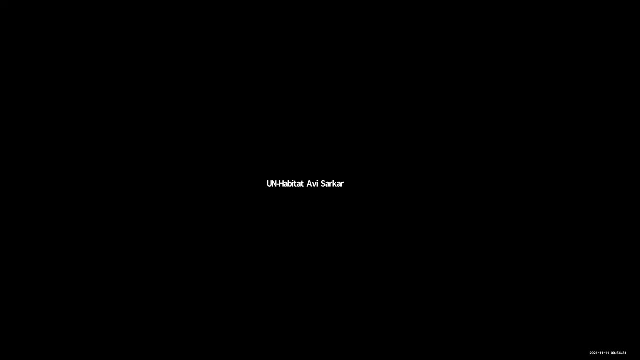 at least in Laos, because we have big water programs in the country. We have an investment. of course, compared to some of the IFIs, it is not that big, but we have more than $12 million of program related to water currently being implemented. 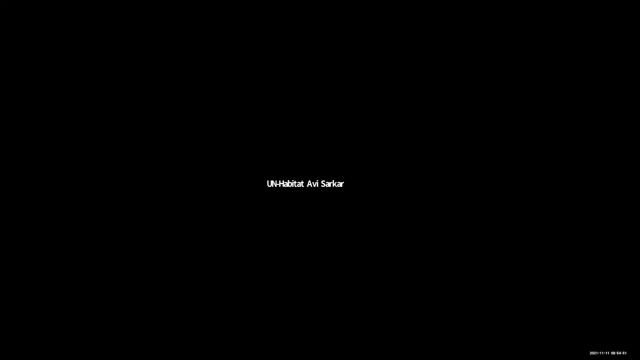 in Laos. So this is a big part of our portfolio in the country And, as I mentioned, we are trying to deal with it through active stakeholder involvement. at the community level, We are trying to find out solutions, bringing in tools and methodologies which can 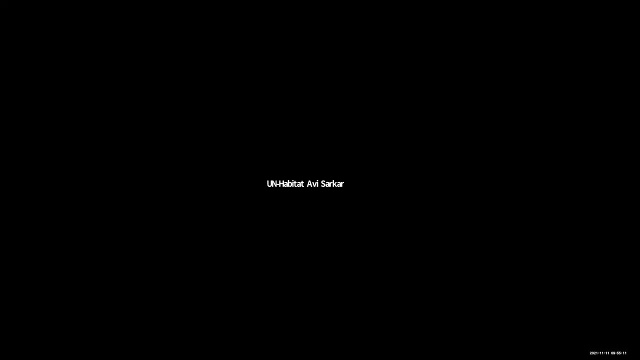 sort of integrate climate change science into the local planning and also trying to see that how we have these tools also in a way that it is easily understood and people can work with it easily. So we are doing a lot of this sort of integrating climate change into 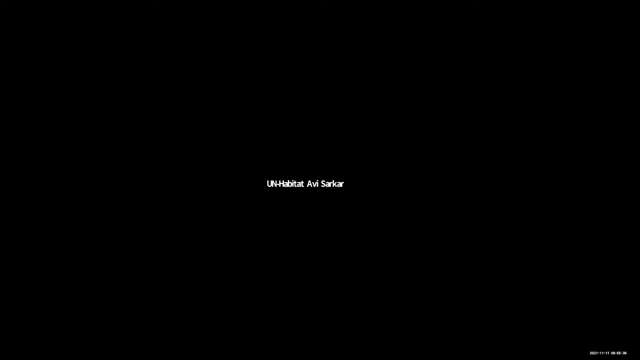 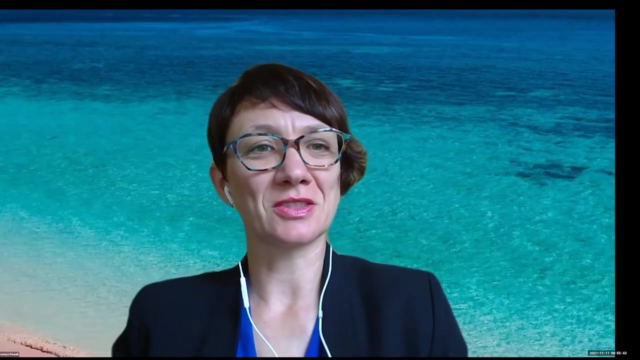 our day to day water projects that we deliver in this country. Yes, in that way, we are very much into it. Thank you. Yeah, so it sounds like, as you say, it's kind of embedded in the way you work. 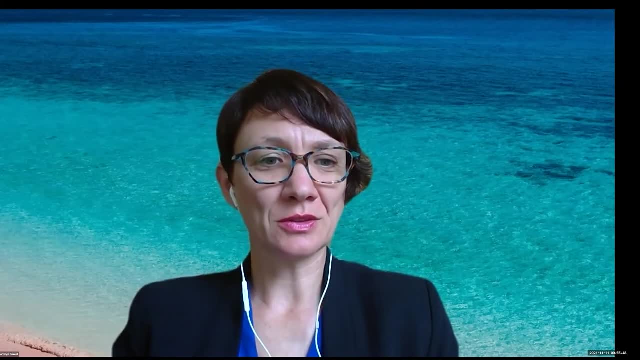 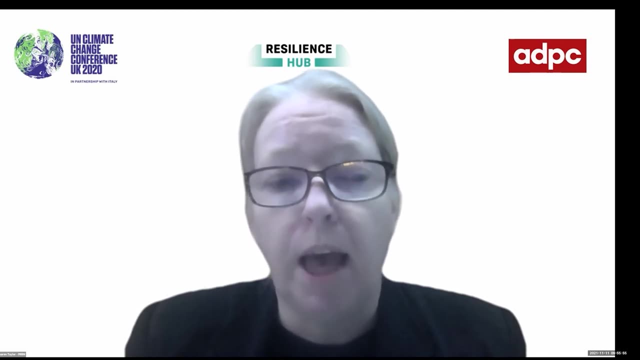 but you're adding more tools to it. Sharon, your response Yes. In three of our project areas in the Philippines, water was prioritized by the community as the major resilience issue they were facing. In the Trinidad up north it was basically. 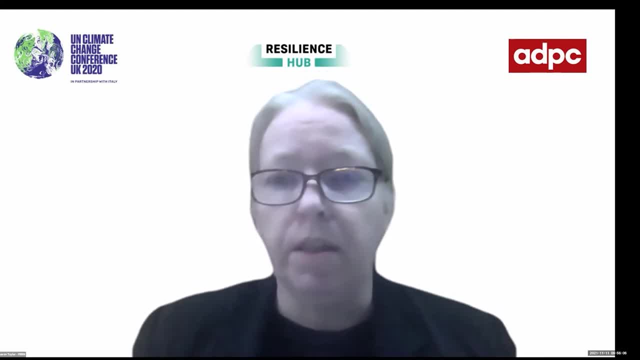 due to flood events. there was box culverts dividing in an agricultural area, but they weren't keeping up with the rainfall events that were happening. So basically, we looked at the historical events in the past and how the duration of the flood events did that whole analysis with. 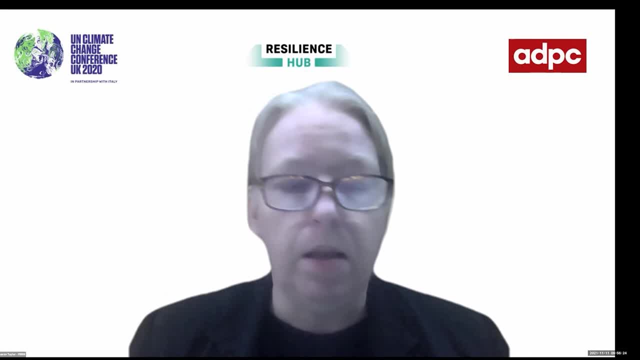 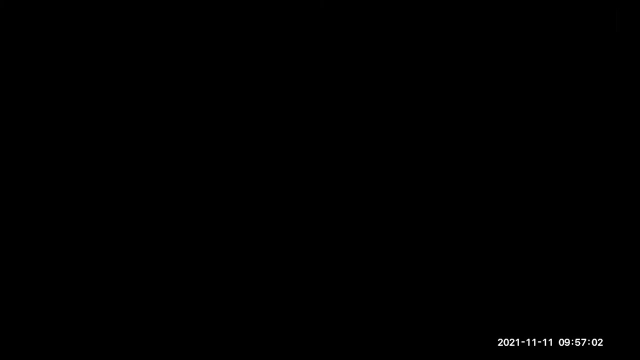 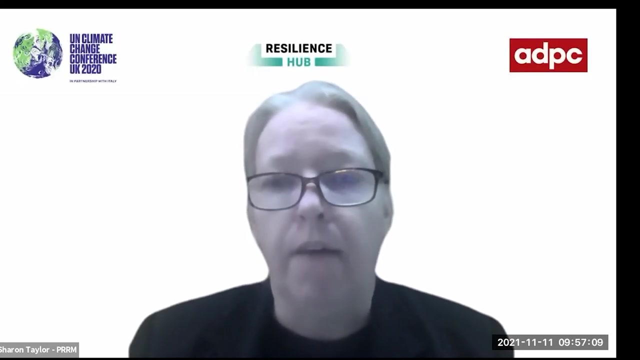 the communities and then brought in the climate change scenarios, worked with them with the community, and then expanded to enhance flow outflow. So we were looking at how can we make sure that the underserved population that didn't have access to water could get access to. 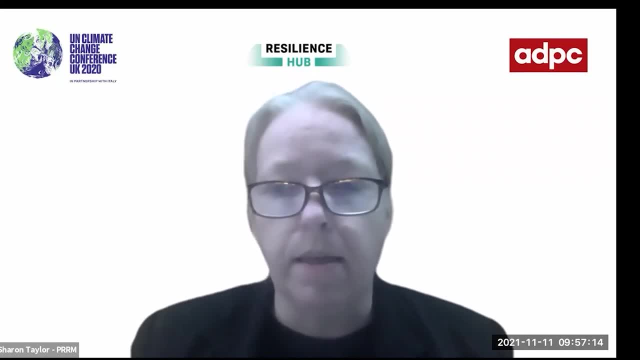 water using the normal water supply systems, but also looking at integrating systems, NBS systems, tree planting for preserving the water, aquifer replenishment, looking at rainwater harvesting systems and integrating that into a comprehensive mix as well. And then the fourth area we were 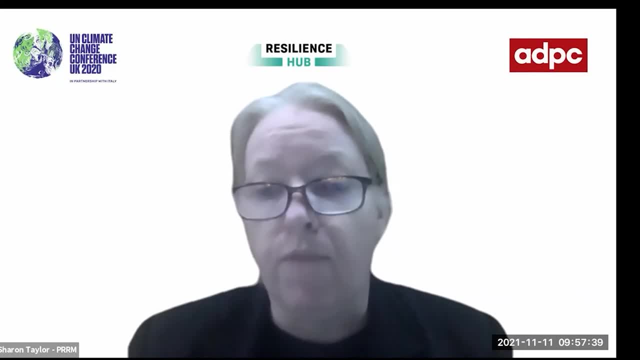 looking at disasters from rain-induced landslides, So looking at slope protection, riverbank systems and management, both upstream and downstream, of the affected communities community. so yes, very much so. it's IWRM is critical to resilience of the stakeholders and, I agree, I think the system in place works to a certain extent when we're looking at urbanization, 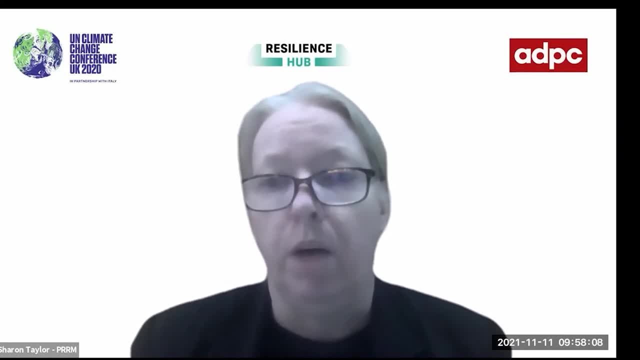 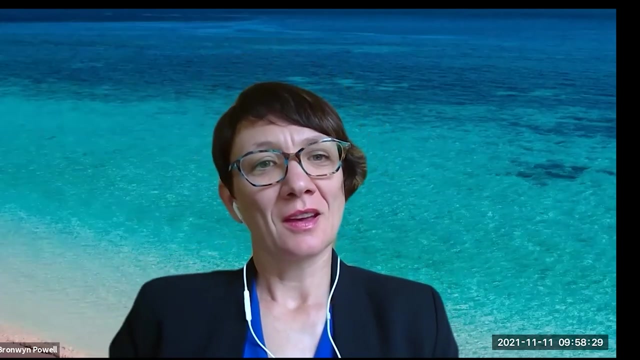 and climate change. it does need to be brought up to the current context and challenges and, as Hans quite rightly pointed out, all the opportunities that presents, as well from the wealth of knowledge we have already. thank you sorry, I was muted. thank you so much, Sharon. I wondered Dr Suttat if you had any thoughts on 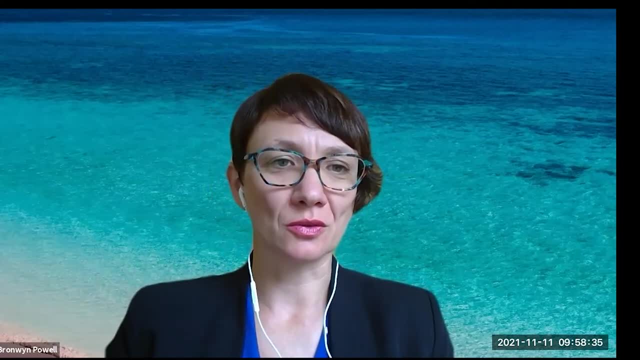 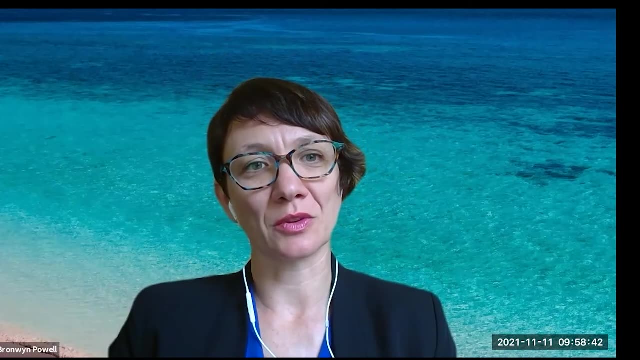 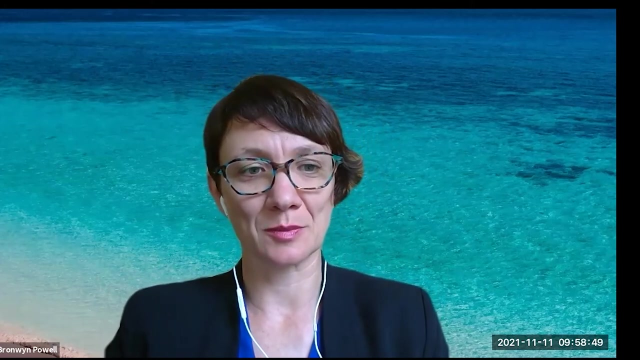 how easy or difficult it is to create new tools that really will help us with the forecasting that needs to happen at various scales to enable the kind of planning through the uncertainty ahead, and we saw some. we just got lots of very nice local examples from Sharon of what that actually 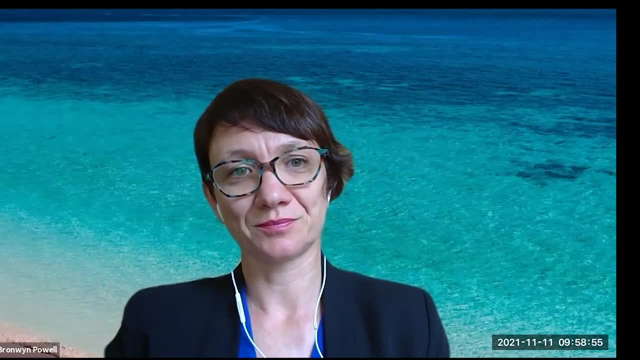 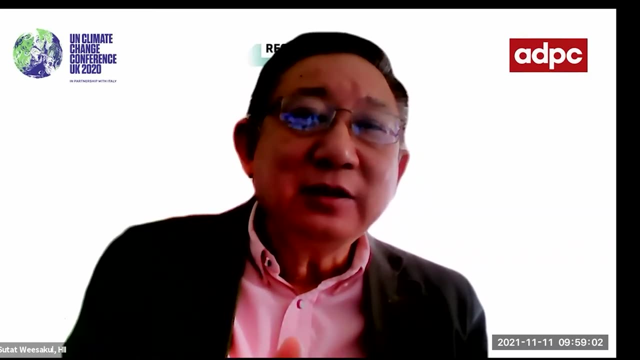 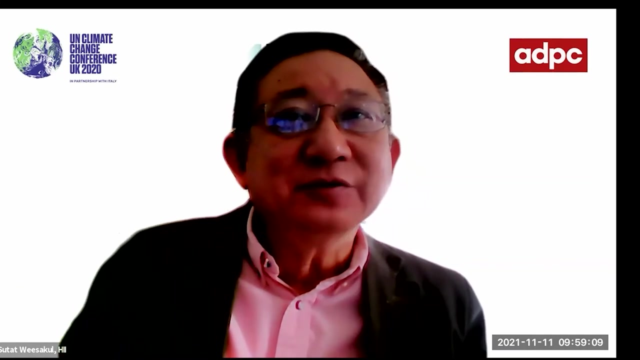 means for local people. yes, for the forecasting for the climate. first, it is multi-scale, from daily to weekly, to monthly, to sub-seasonal, to annual and to the long terms. there is a multi-scale for the forecasting, with different techniques and with different uncertainty and variability. also. 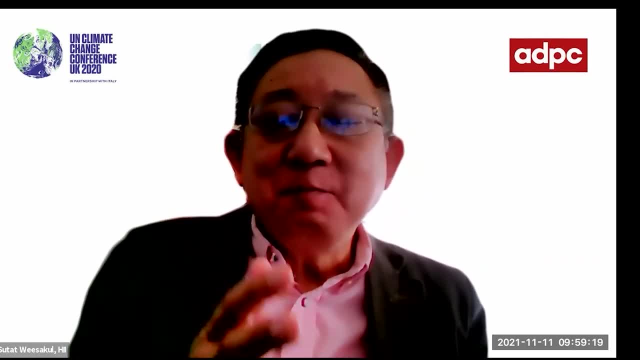 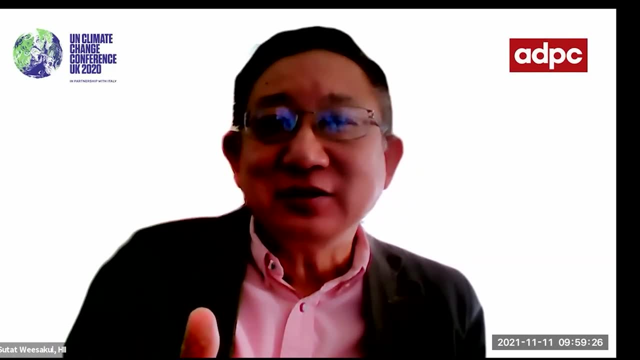 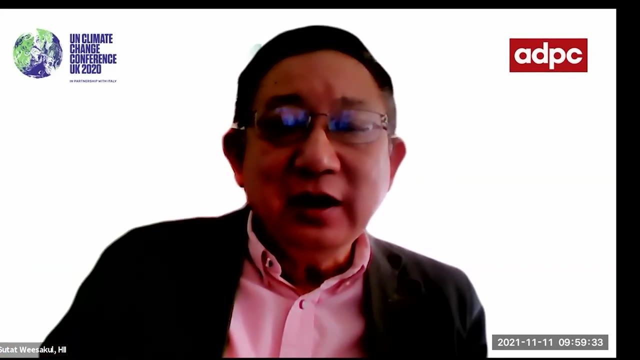 but therefore you need to test your systems with the field measurement to be sure that that is the good forecasting. you need to test it and, of course, really long-term forecasting is difficult to to test it, therefore, you need to involve in the accepted and uncertainty. so, in order for the long 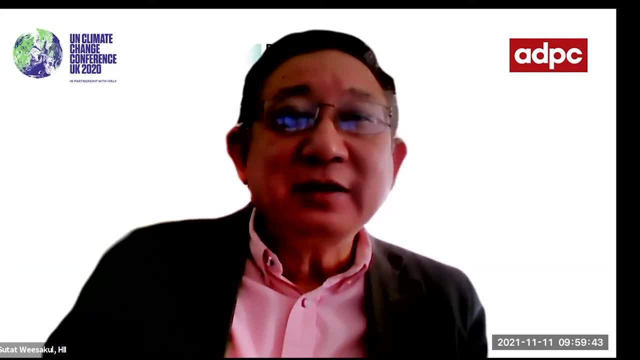 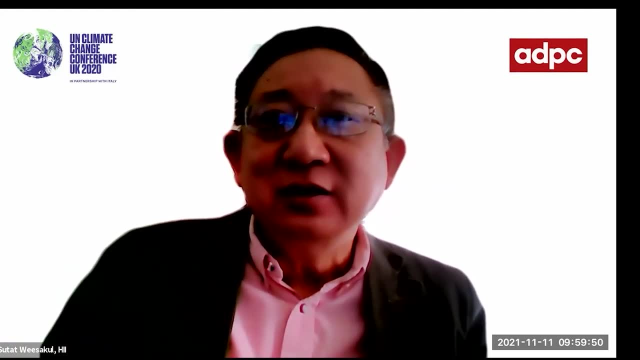 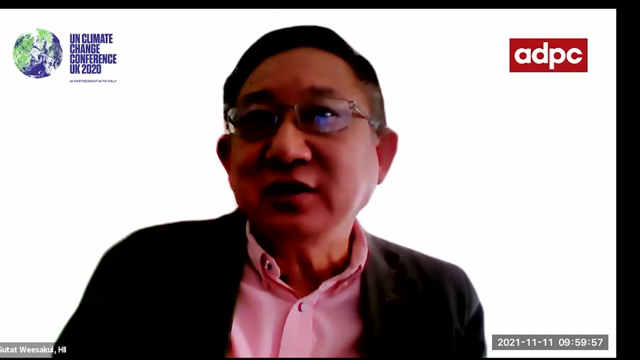 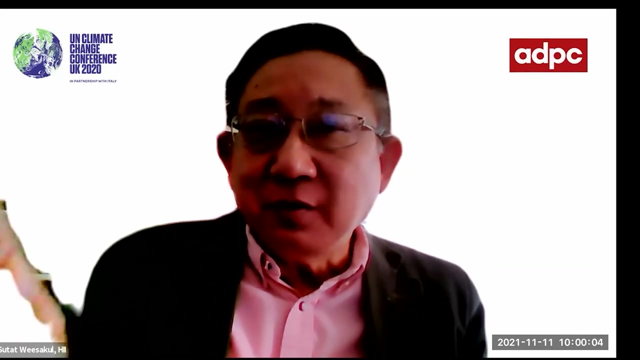 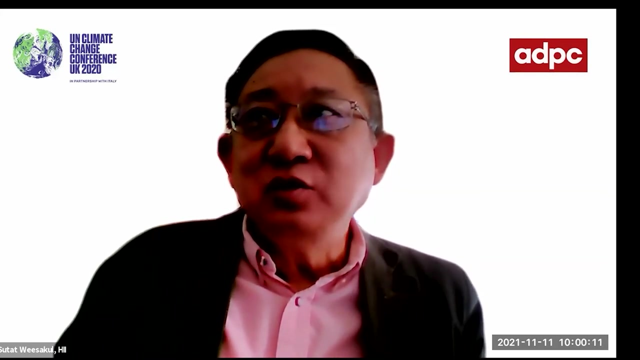 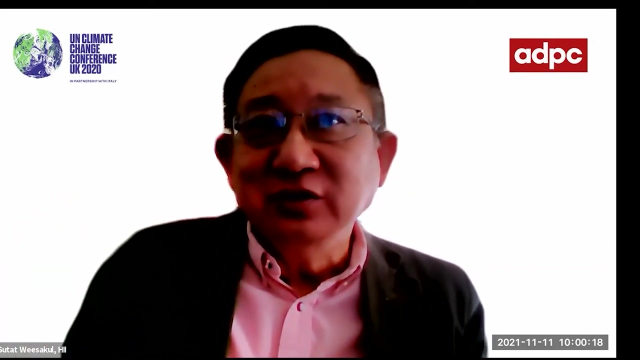 terms of the modelings, you need to do multi-criteria analysis and focus on different places like the the on the on the on the the on the on the on the set and the length of the monsoon. so if there are different, different parameters to forecast, 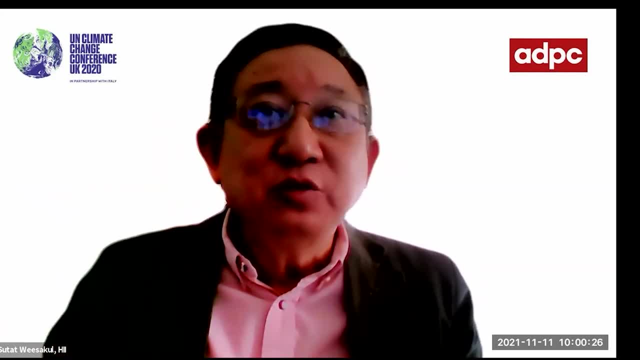 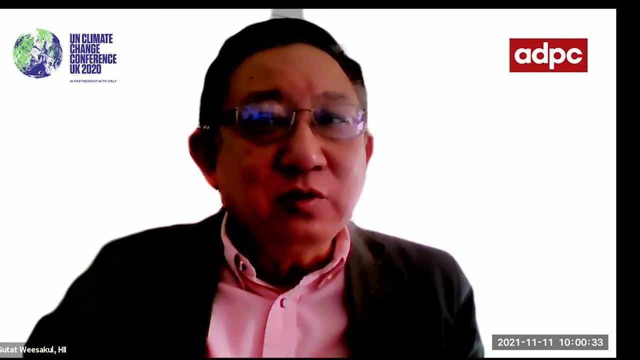 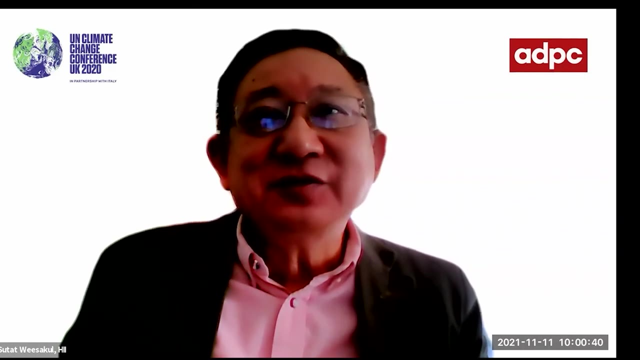 therefore, if you imply that which model should be suitable, if there are many models, you, you rank in, you rank it and then you, you, you can take an ensemble from those selected models. so i think this is the the good method to select with reasonable, and it can be put into into iwim. 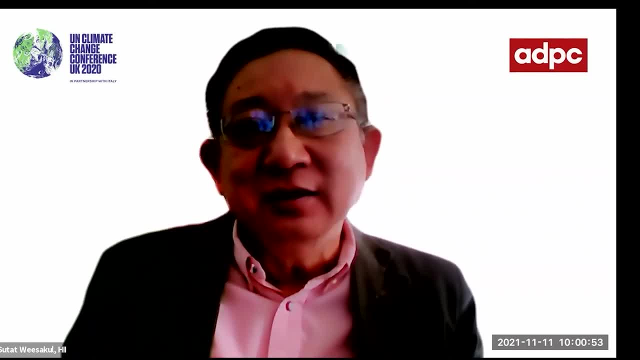 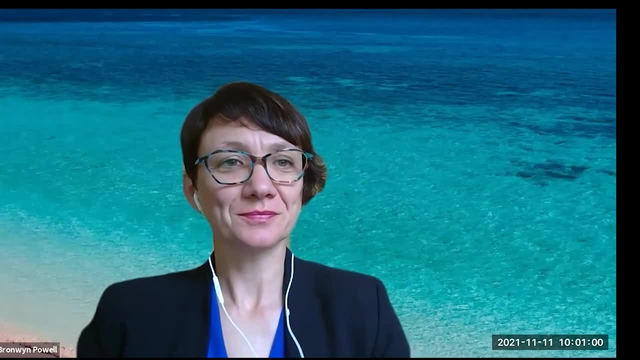 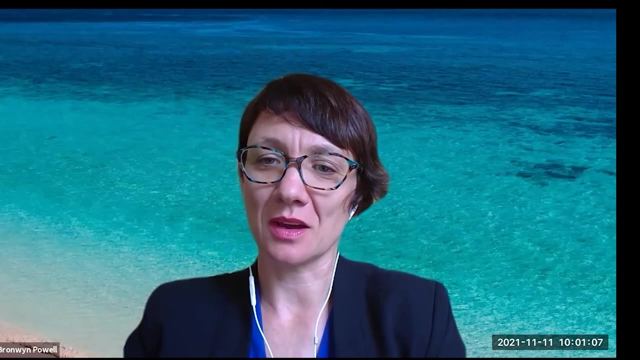 to have a bigger scenario for the operation and planning and the policy. thank you, thank you, dr satat, i am. i've noticed that there we have a question that takes us back towards food security in the chat, which is a question about, um well, the effect of climate change in. 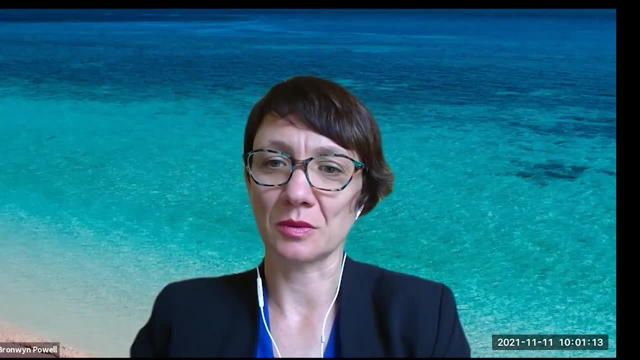 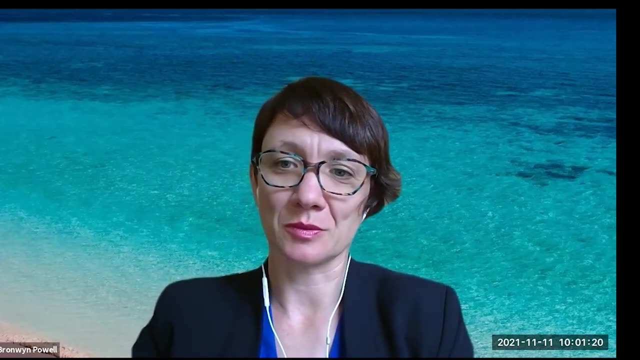 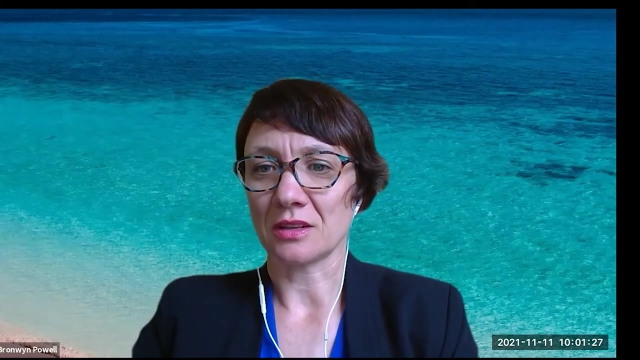 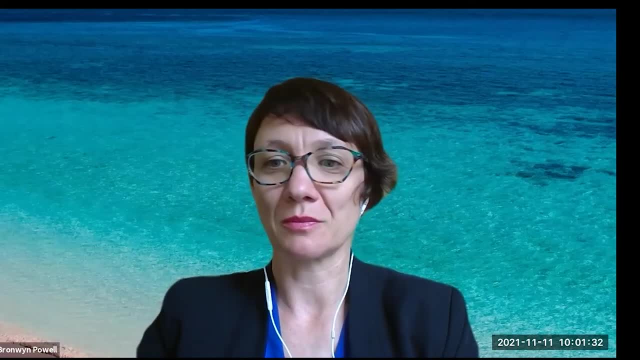 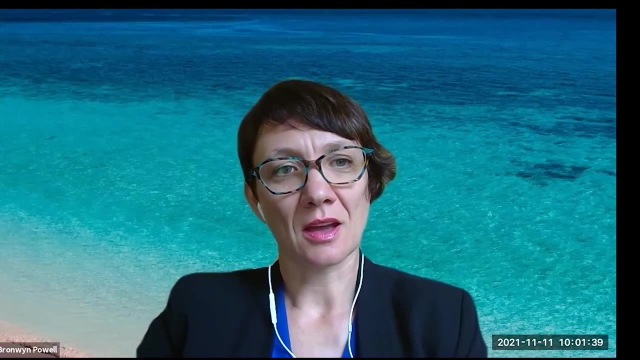 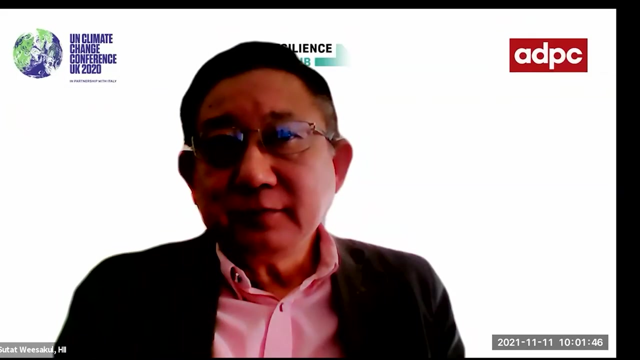 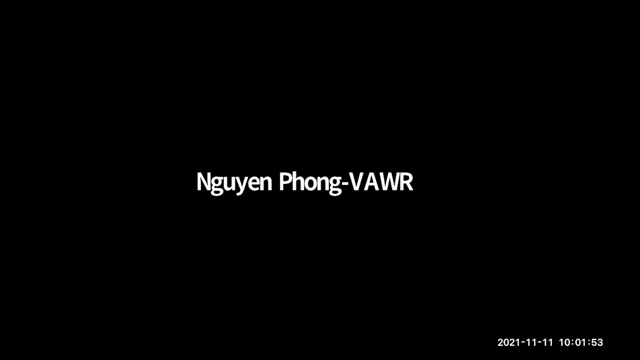 and volume determinations, and are there new modules or manuals or guidelines that can help with this? so i guess in the agriculture and irrigation sector um have new models got to the point of being implemented in this way. okay, so i i sorry i opened my camera, i don't know why, but okay, can you hear me? 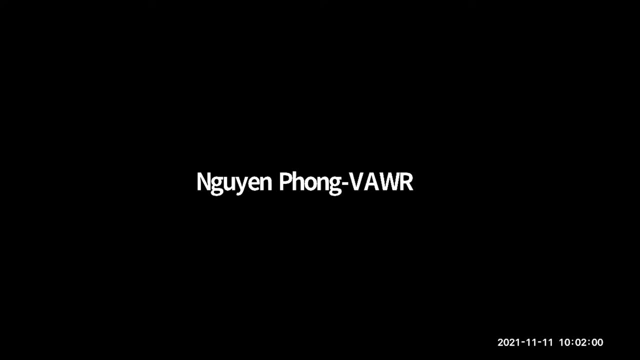 yes, we can, we can hear you okay. so, uh, i think very good question, because it's really unnecessary to to uh to calculate irrigations consumption: um, um, um, consumption for the um, for the agriculture production. actually we also developed some, some seeds, some other variety that's need less, worse consumption. 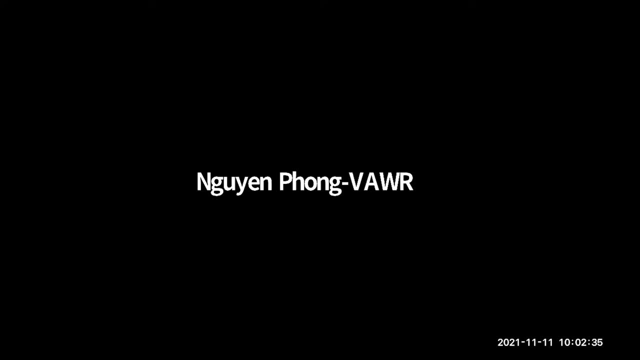 and also um can uh can use uh for the uh salinity institution. so it's really necessary to to calculate the water consumption in the irrigation schedule and of course it's so necessary also to have a new manual on guidelines for the irrigators. and even in vietnam we have the irrigation. 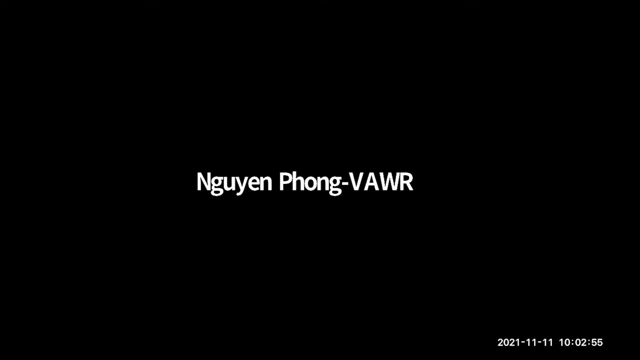 management company who will? who will manage uh water for irrigation? so, um, um, the, some manual and some uh guidelines also need to prepare. of course, you need also need to need it need to to fit to, to fit to the uh, to the, the seed and the variety of the petty rice, for example. 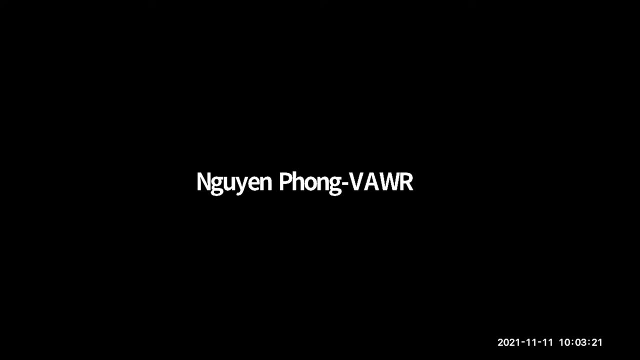 and the second ones in the for the highland, for example, we have to plant coffee and pepper, for example. so more and irrigation saving, irrigation technology applied to reduce water consumption. of course also have already manual and guideline for the irrigation for the high valley crops and also in the highlands crops. thank you. 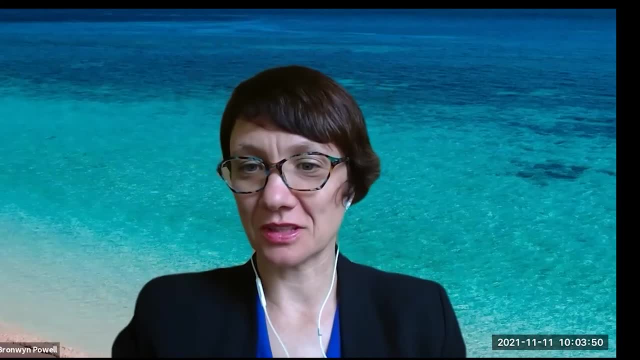 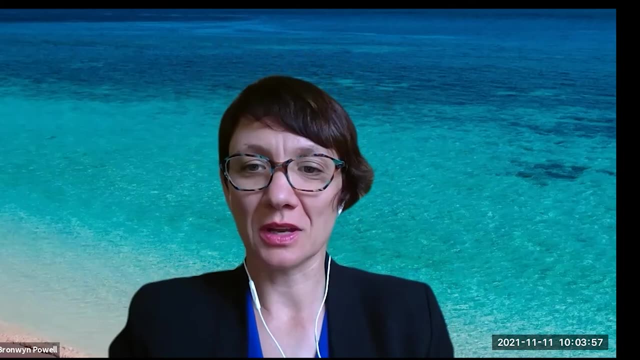 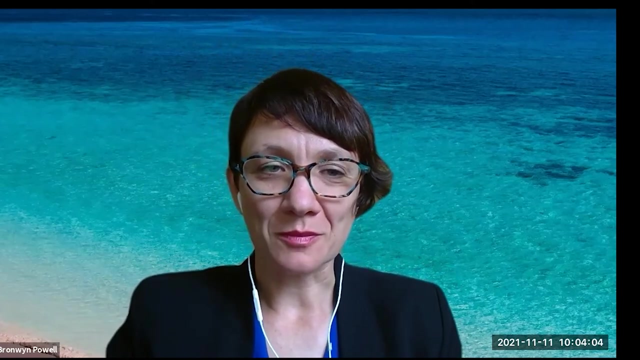 uh, thank you, dr. yeah, it's. uh, it's interesting to hear about the kind of water efficiencies and water saving um mechanisms beginning increasingly being needed to be put into place. i think i might just open it up to the um panel. do you have a question of each other at this point? 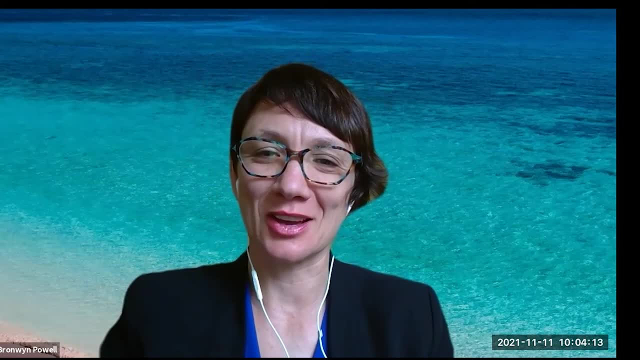 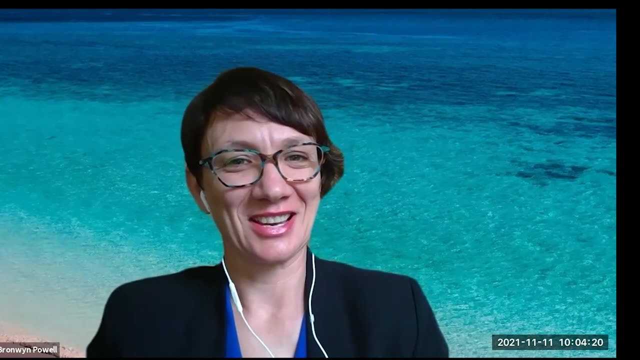 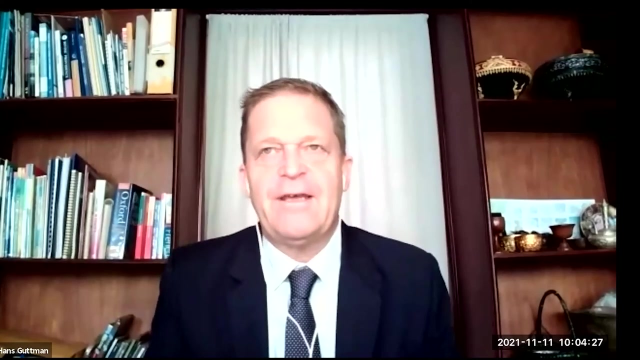 i mean, it's a, it's a rare collection of experts here. we might as well, uh, open the open the floor a little. i know, hans, you had so many questions. yes, you've got your hand up good. yes, if i may, perhaps, and direct to avi, i think, uh, your presentation an example of of having 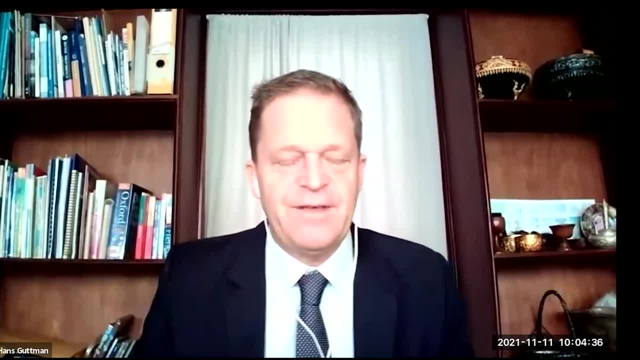 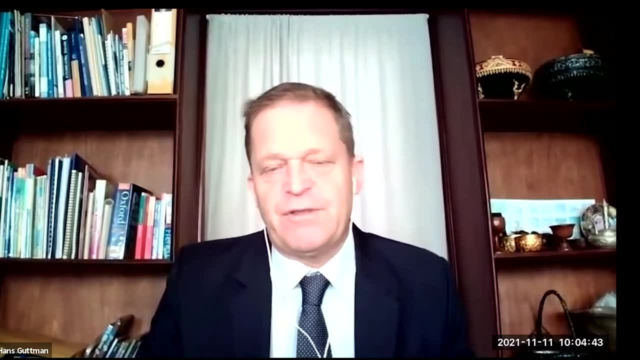 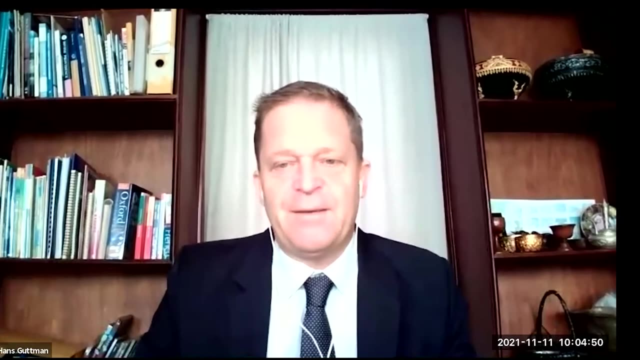 uh, going ahead with a sort of nationwide comprehensive uh assessment? um, do you see that as a replicable approach- not saying that you should do all of india in one month or anything like that, but um of taking this bigger picture, because with that amount of data also some of the 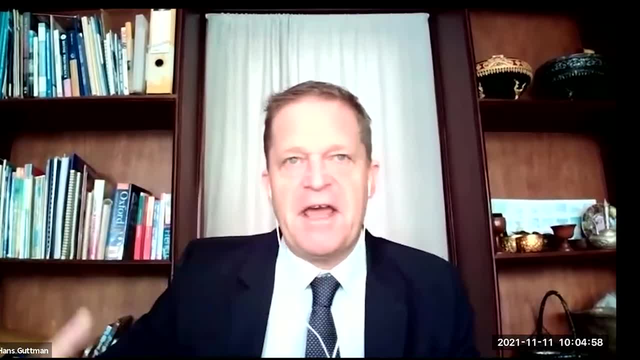 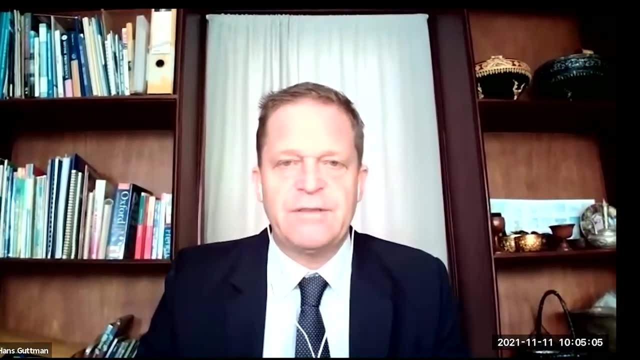 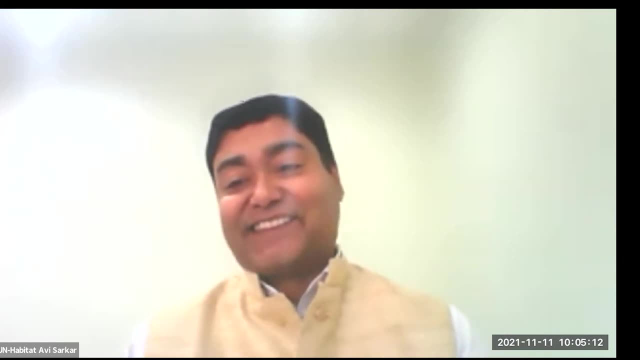 difficulties in statistics and aggregation are reduced because the sample size increases. so just your reflection on that in this context. um, thank you, hans. i mean, hans himself is such an experienced person, i think he knows the answer to this. i mean, laos is a. laos is, of course, a very 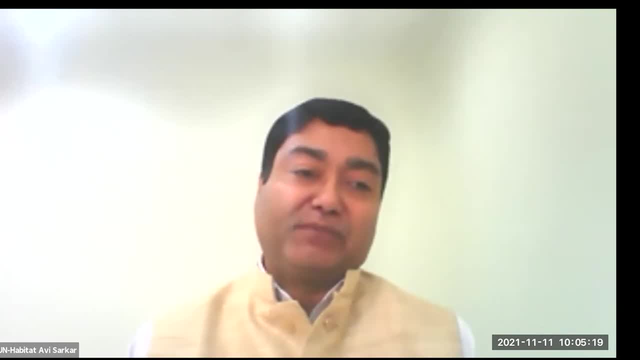 uh, interesting case and also it's 7.2 million people- it's a very small country we are talking about, and there's a lot of homogeneity. of course there is diversity, but there's a lot of homogeneity. and and there is also the system of governance also helped in the system on the data collection. so 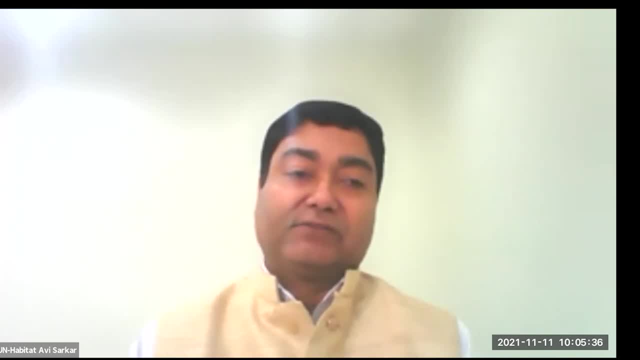 there are many advantages of collecting data in that way in laos. but of course, what is very important that we found out and which i mentioned briefly earlier, is the leadership, also the interest of the minister himself to drive that agenda and to collect that data, and also the 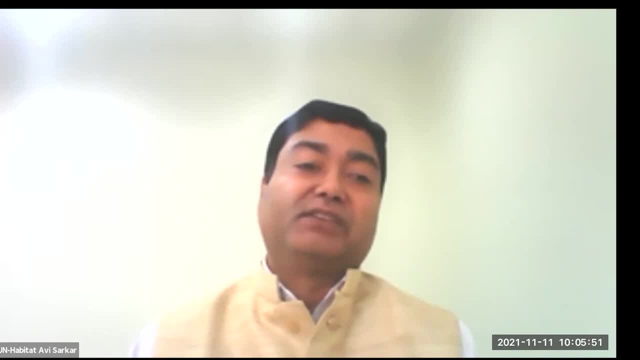 interest of the national assembly. i think all these different factors sort of spurred the data collection and we also kept the the design of the data collection as simple as possible so that the numerators, who are the legwork at the field level, could collect it. and it was not a sampling exercise, it was. 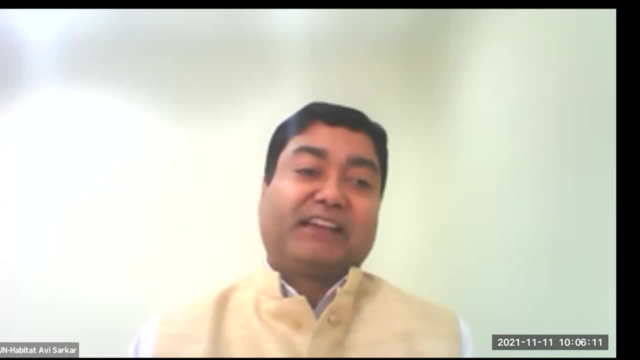 it ended up being a census. you know, it was like we collected data from each and every village regarding these vulnerabilities. um, in a different country, in a different context- i think you're very right, hans. i mean, possibly in a country like india. i mean, can we do this sort? 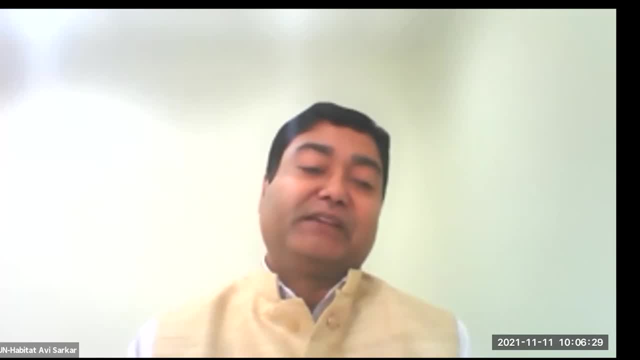 of an exercise. i mean, perhaps we have to end up doing a bit of a sampling right, um, but from our experience we have never done in any other country. this was the first time we were thrown a challenge and we did it and and thankfully it worked well. but what we are planning to do is that 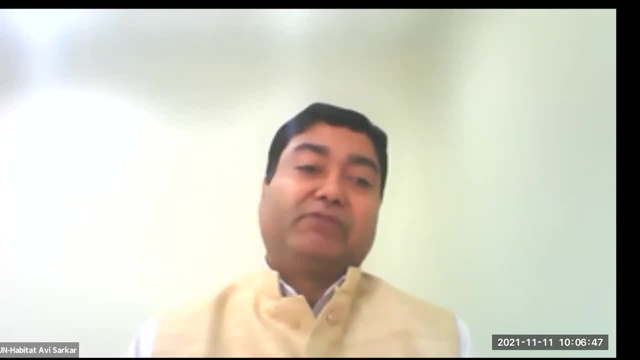 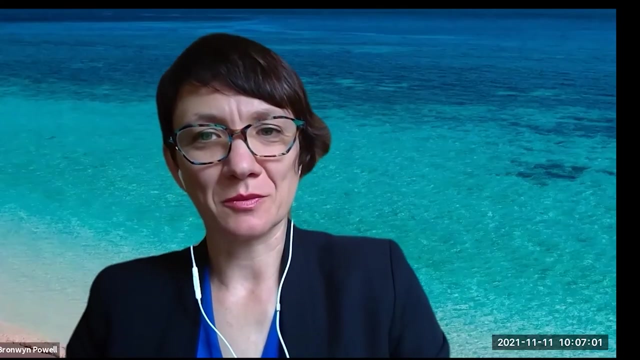 since we also liked what we have done, we envisage that we will continue this exercise over the next two, three years so that we have a sort of an annual check and see where what is the sort of dynamic movement, if any. thank you, yeah, thanks, avi, i guess i'll just jump in. i mean, it was interesting. 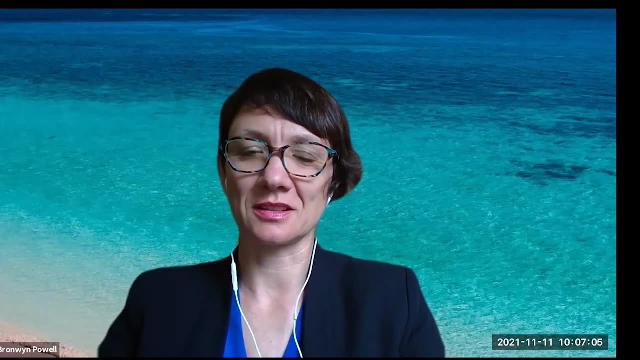 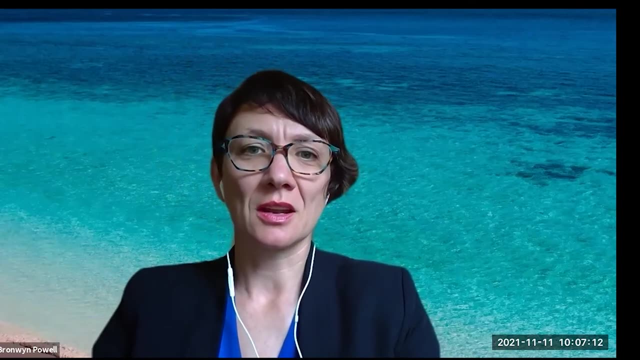 you've done this massive vulnerability assessment and clearly that's the um community's priorities. you said you collected a lot of data on what they see as their priorities and challenges- and i guess that links a little bit to what sharon was talking about as well- and community-led solutions. so perhaps first to you. 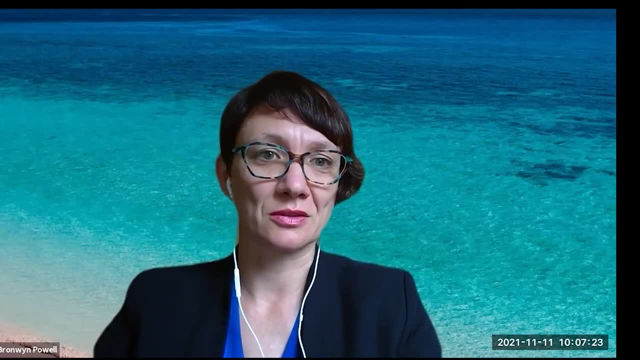 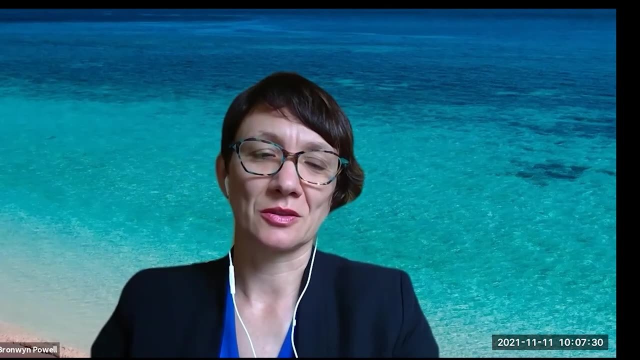 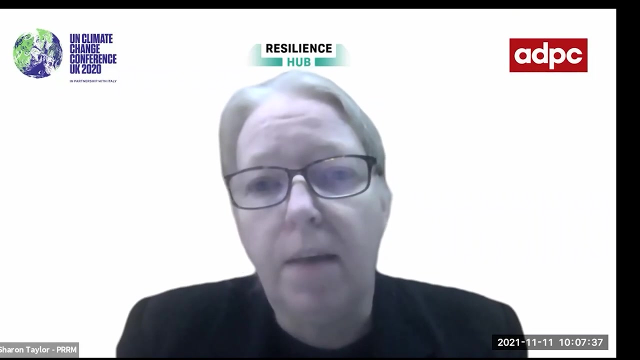 sharon. how do you see the kind of models that dr sutat is talking about, uh, meeting somewhere in the middle with community-led solutions? so how do you see these two realms um coming together positively? yeah, we did have one direct example of that in one of our project areas, where 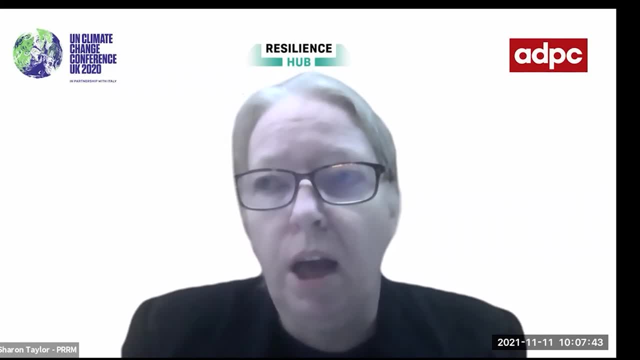 our participatory approach to guiding the communities in identifying their priority issues and developing solutions. integrating the nature-based solutions into those was actually taken up by the local government unit, as they saw the um the importance of the community voice in the planning and budgeting process processes, so they integrated some of the tools and methodologies that they've been a participant to. 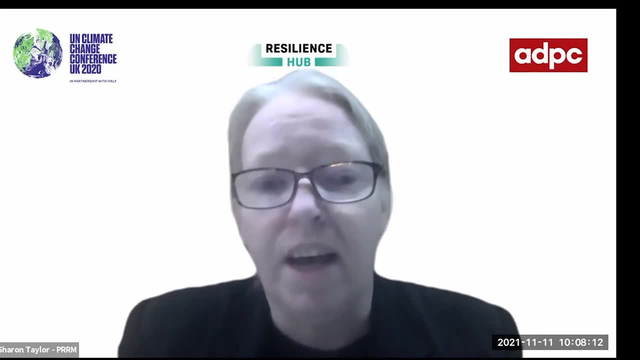 in our series of workshops and data gathering into their own planning methodologies as well. so there is scope, yet that that's. I admit that's just one example, but it gives hope, there is scope. there is scope and even the marriage between the scientific climate change data and the community's. 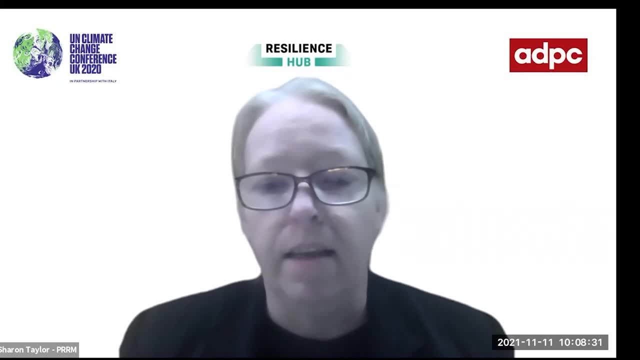 indigenous knowledge of events in their areas can be married perfectly as well. it all depends on the facilitation and the guidance given during these processes and to show that, yes, it can be done, and to try and maximize the opportunities for where that can be done as well. thank you, 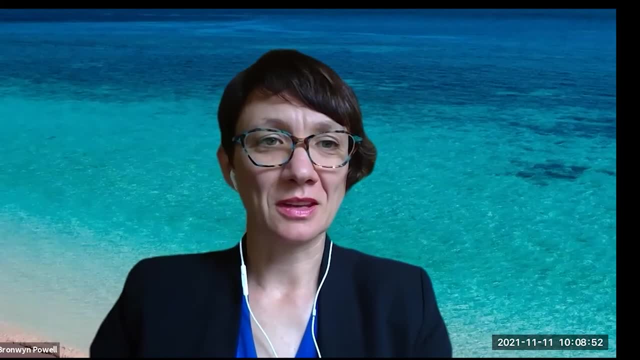 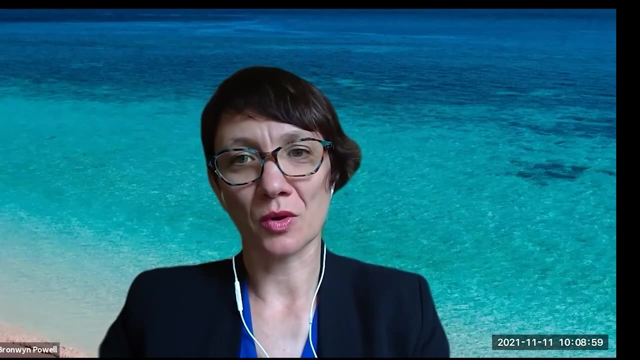 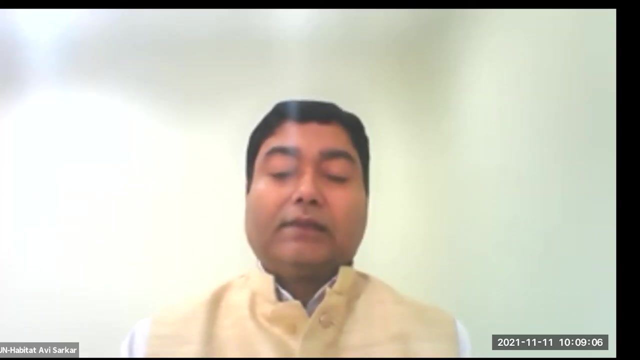 thanks, Sharon. and then, yeah, really interesting example. and then, Avi, I guess I'm wondering, with all of those, the vulnerability data that you have now, what, what will be put in place to support communities develop their own local resilience strategies? yeah, it's a very good question and actually, 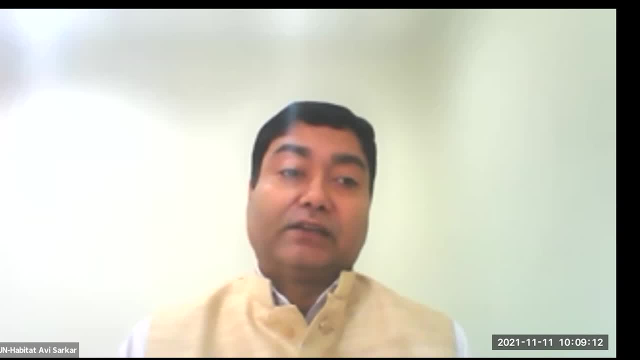 we're working on it. we are currently working in 200 sort of settlements in Laos, as I mentioned, big and small, and and so we are working in some of the biggest cities in central Laos, in the province where the city is about 40,000 people. 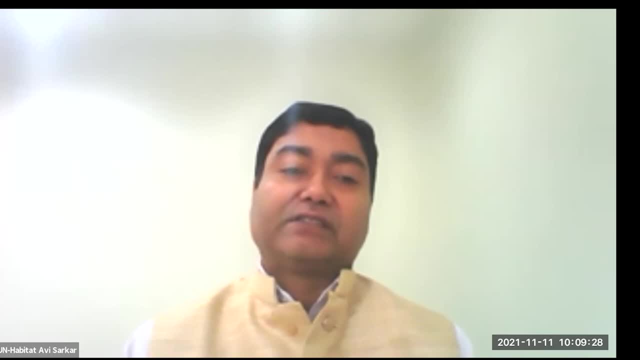 so we are working in those sort of cities in that, at that scale, and then we're also working in very smaller cities, smaller communities. so what we're doing is that, building on this vulnerability assessment, we are engaging with the local stakeholders in defining what we call action. 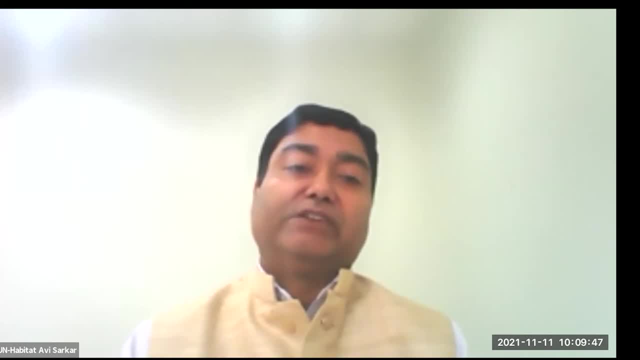 plans and sort of coming up with a set of menu of interventions that possibly could enhance the resilience of those communities, and then we are picking up from those sort of communities that are of actions identified on those action plans. we're picking up one or two and then we are carrying on. 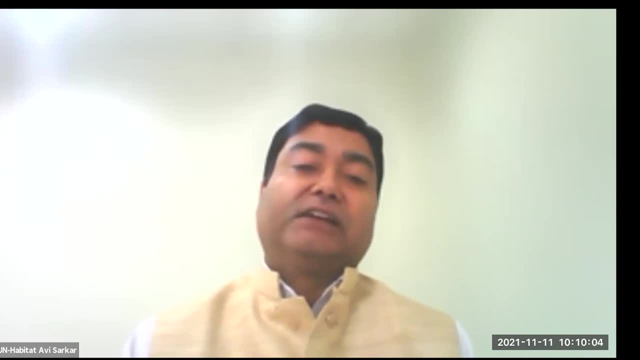 some small level infrastructure at the community level. but what is happening is in this process is that it's empowering the communities, their understanding and also they also now have a menu of sort of of sort of interventions they can ask for if some other development partner comes in. 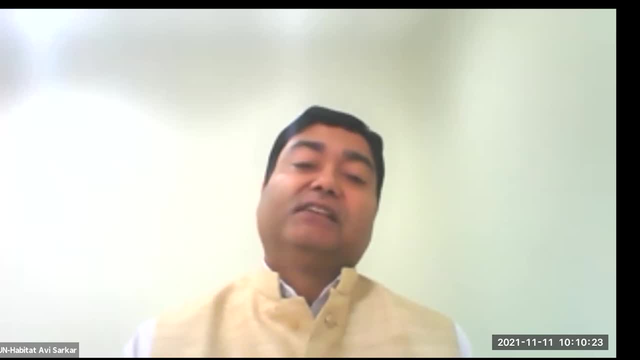 into that sort of community to engage in. and then just to kind of go back to what Sharon was mentioning, I mean we had some very interesting experience in Laos that after all this different data and analysis and all what we found, and when we went back to the communities we found that their indigenous knowledge and they're so good at it- 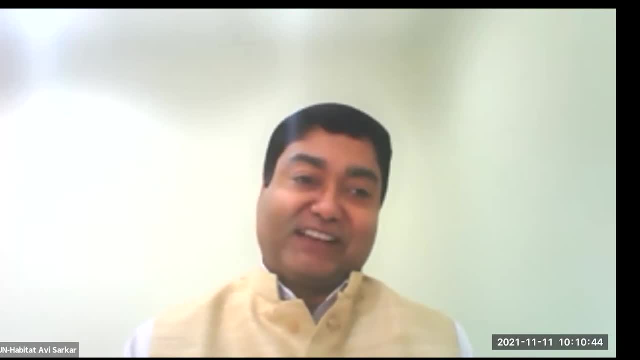 that they basically said: whatever we had to do with so much of analysis, they said, yes, it is getting a bit warmer, yes, rainfall is more intense, and they knew everything I mean. so I think it was a good experience for us that we need to, so to learn from the local communities as well. thank you, yeah, thank you. I mean, you've all. 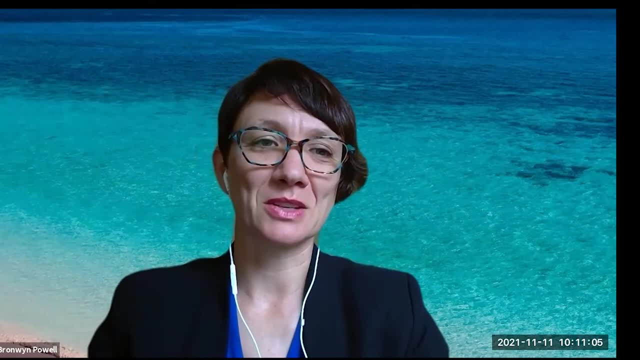 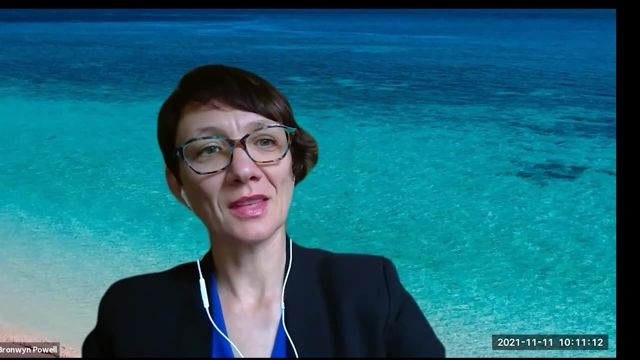 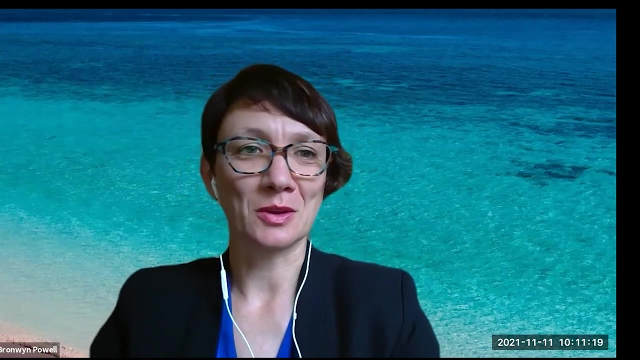 raised such an interesting point and I think um mentioning the local knowledge and indigenous knowledge meeting scientific knowledge halfway, um that it all can contribute to a resilient future. it's been an absolute pleasure hearing from you all, talking with you all today. I'm going to hand over now to uh Hans Goodman. 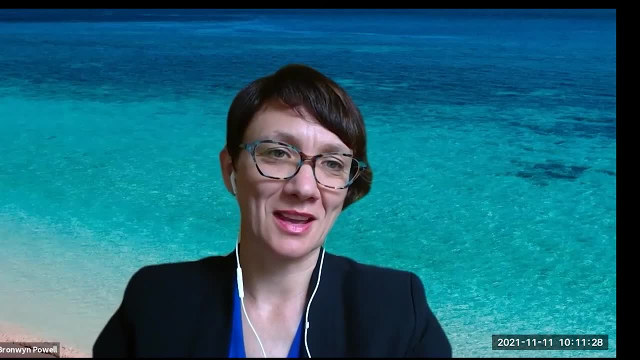 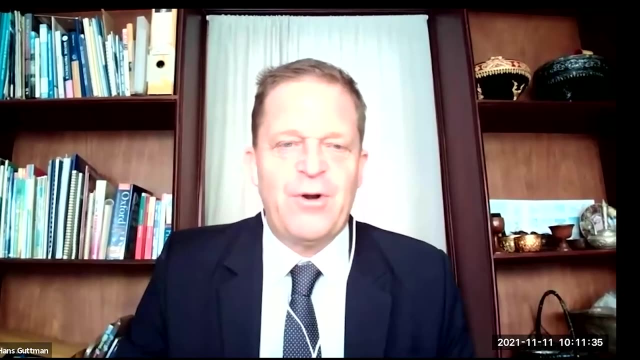 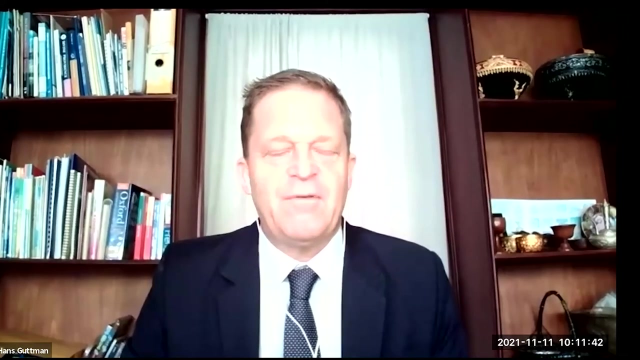 who is going to give us some concluding remarks and close the session. thanks for having me. it's been a pleasure. well, thank you. thank you very much, Bronwyn, and let me just jump in here. I mean, if we go back and look at the beginning, apart from my own presentation, there was some urban key issues. 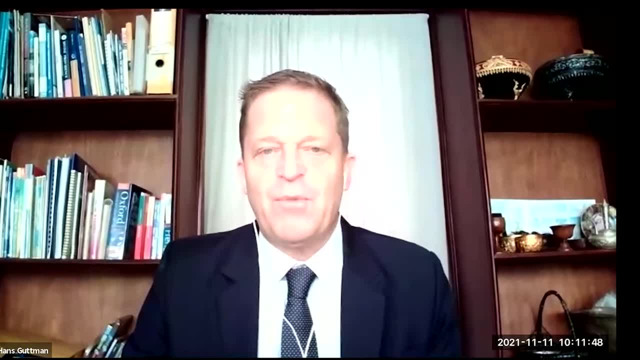 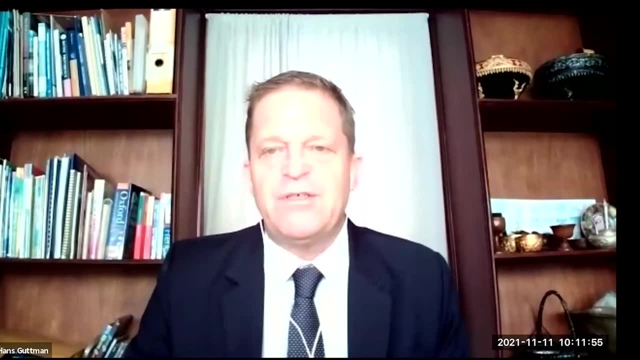 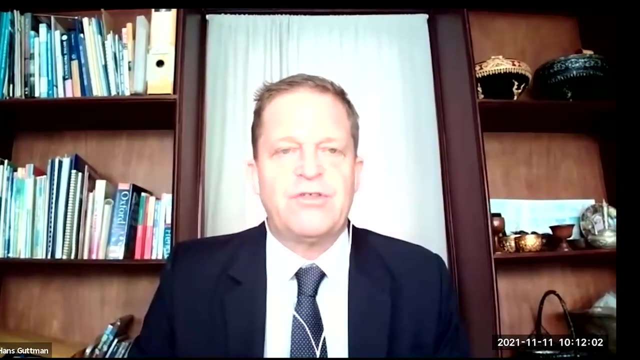 put forward. there was this nationwide approach presented for Lao PDR and and how the community day's planning can be improved um in decision-making processes to respond by having this vulnerability information now. we then also touched on food security and agriculture and I mean, as pointed out there, it's 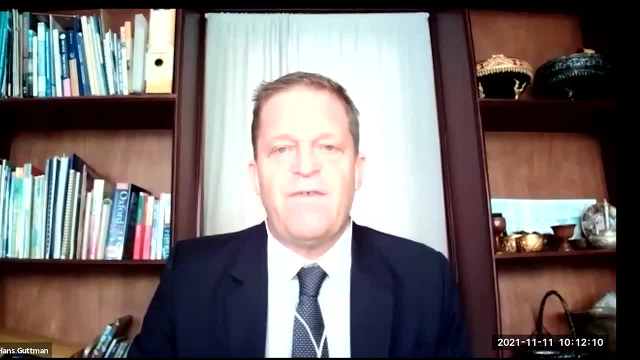 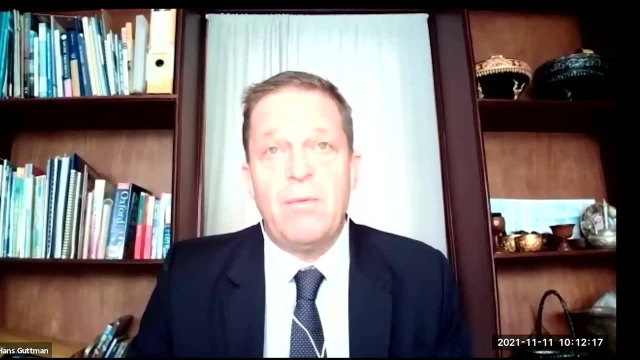 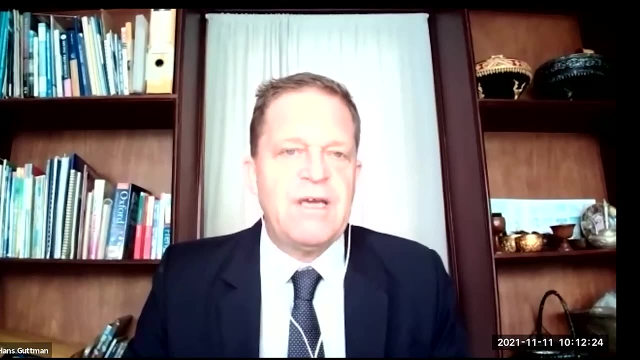 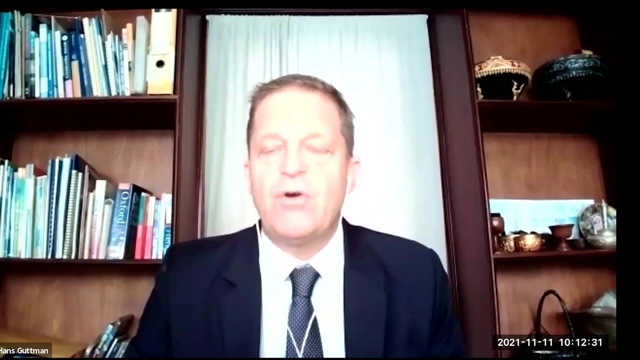 the biggest water user in many countries and thus it's vulnerable to change in hydrology. and from there on there are many challenges and many opportunities and listed water and efficiencies, nature-based solutions, Etc, Etc. but if we look at the some key messages, perhaps here I think um. what was clear is that resilient urban water management is an iterative and long 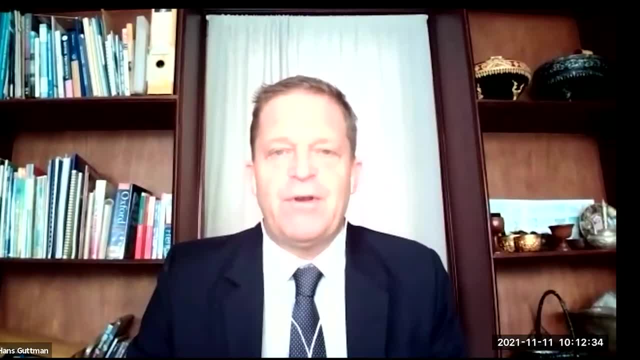 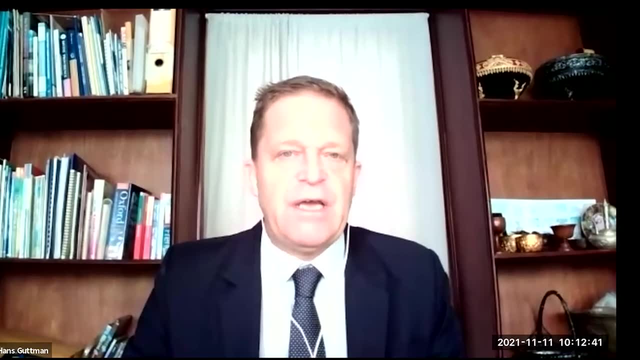 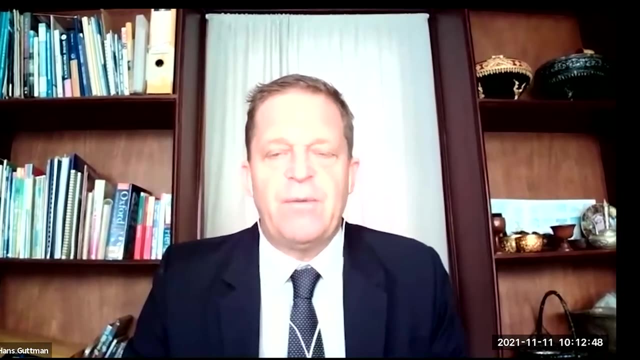 term process and the unpredictable population growth and urbanization patterns add to the uncertainty in water demand, Etc. and exacerbated by climate change. so these uncertainties, they are compounded and thus the cities should incorporate analytics on vulnerability and resilience and uncertainty in water system planning. and a conclusion: it's very complex. 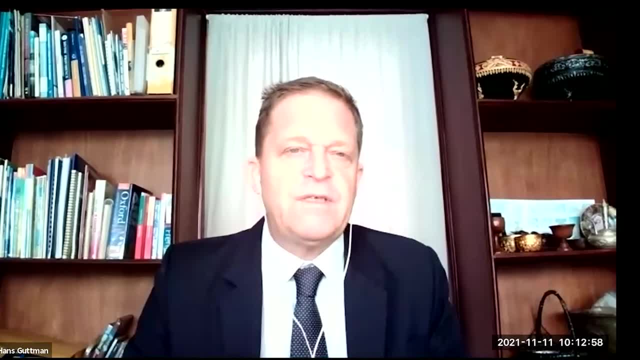 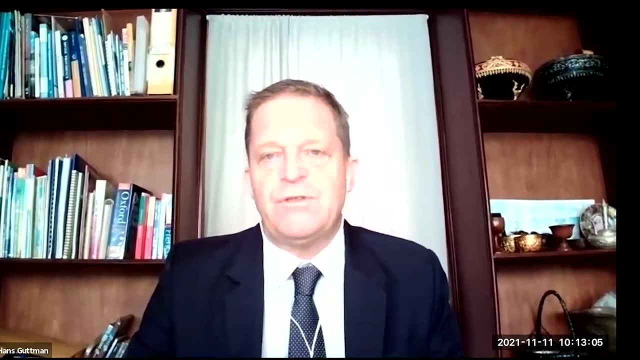 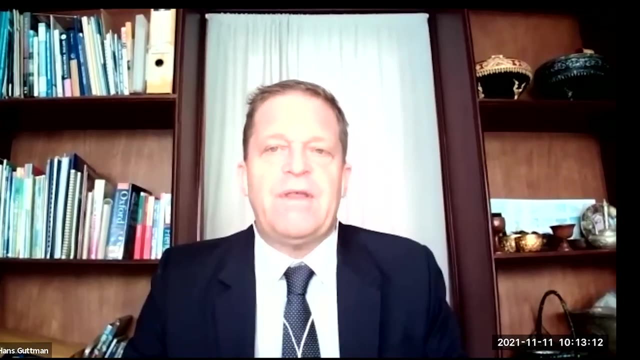 but not insurmountable. another point is that iwrm approaches needs to be incorporated by, or needs to incorporate, Futures and extreme events and other things that may become more normal than now, but the approach um will. we will need to revisit it, not just from a climate change perfect. 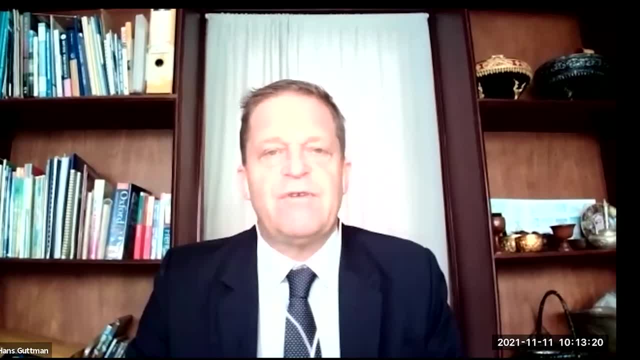 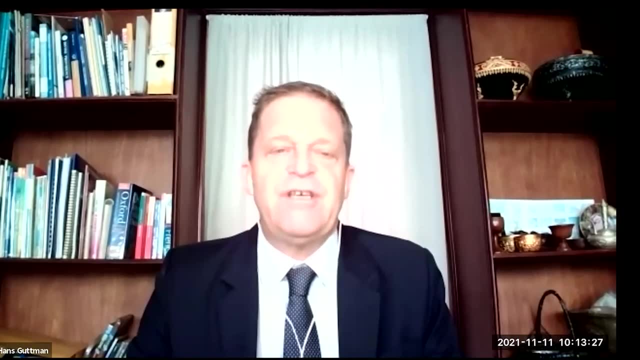 perspective, but also the changing roles of actors, whether it's regional or local level, and the governance- and I think that was good forward in the governance, in building water resilient and achieving water security for the future. so there are some examples. we're on strengthening the link between the- let's call 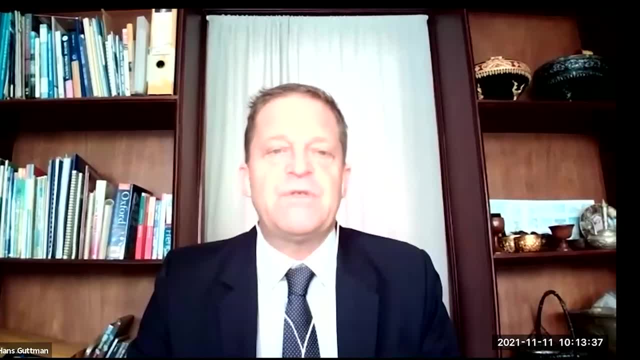 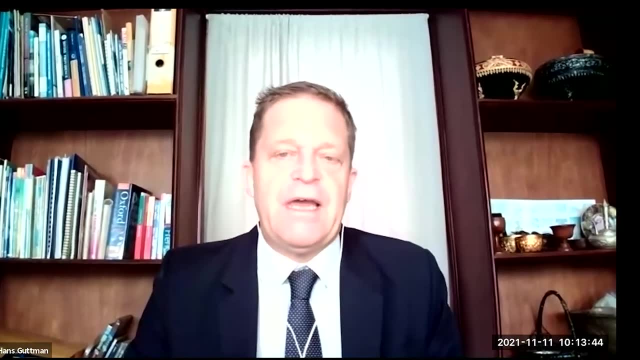 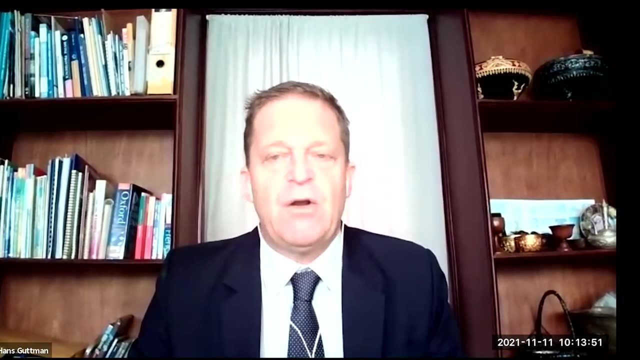 it the users, the people or water users as such, and the groups that are providing information as a basis, and we refer to forecasting or other types of predictions. it's also clear that there is advantages of bringing communities even further into the process and being closely involved, addressing inclusion- I think again there from the 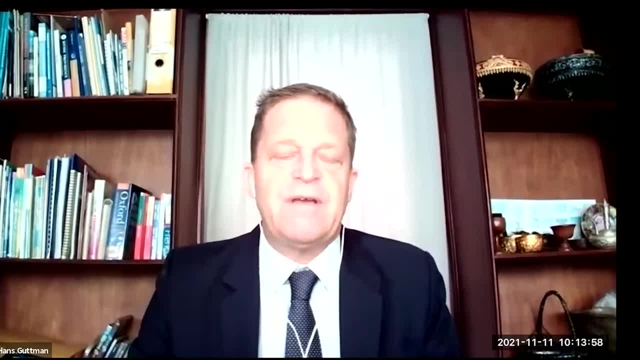 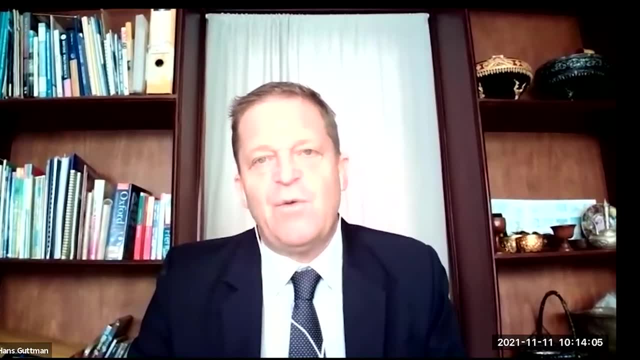 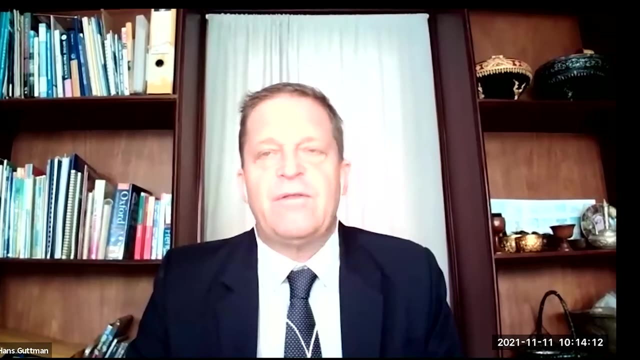 experience. we had some good examples on how engaging communities help dealing with some of the uncertainty, and I mean in in some their idea. iwrm, I think, was said it works but it needs some refinement and upgrading and I think that is a take-home message. um also the recent lessons from 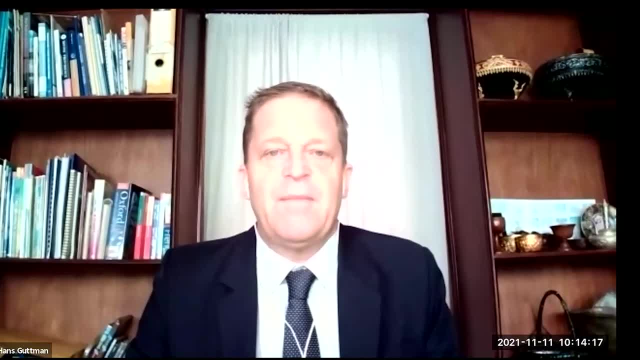 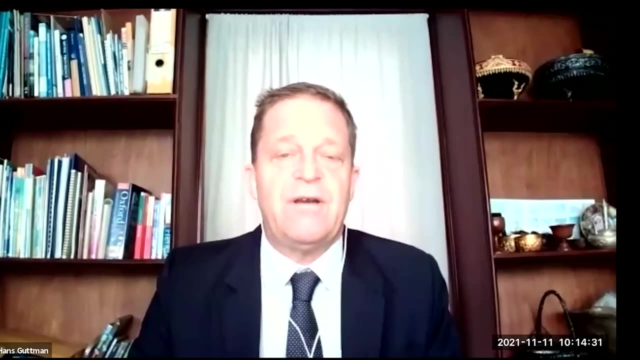 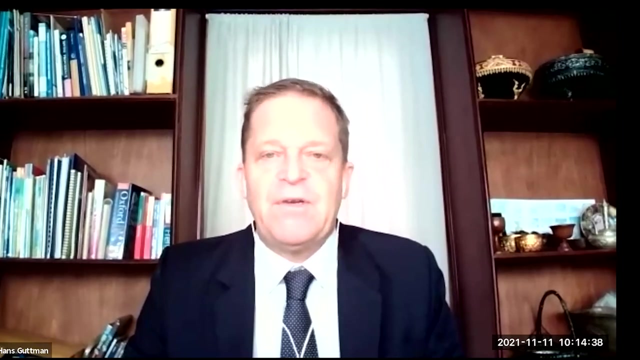 extreme events globally calls for better practices and being able to work on applying this in an uncertain environment. now clear that this is not only for building water resilience, but also National water security. and and as the world, as Asia, is recovering from social and economic setbacks by covid19 and adapting to 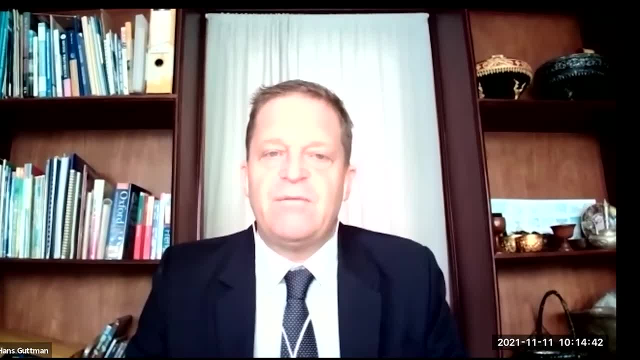 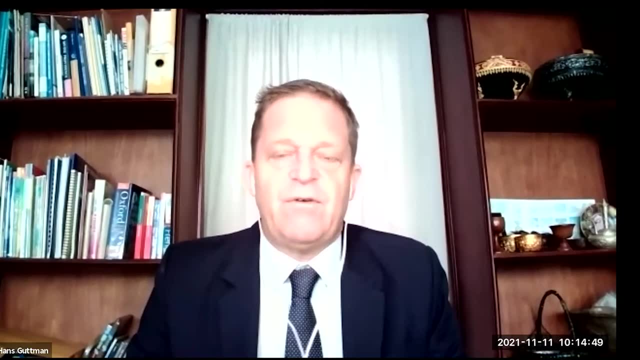 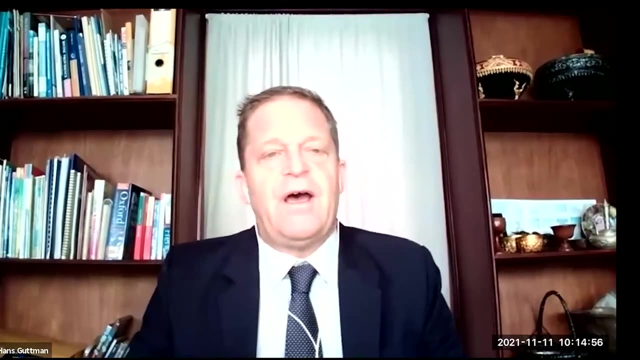 climate change. this pushes water security high on many countries in agenda and therefore learning from these approaches is important. water security, after all, enables social and economic development and conditions for a healthy and prosperous society. so, to conclude, iwrm is a key component of resilience building in, including in urban areas. 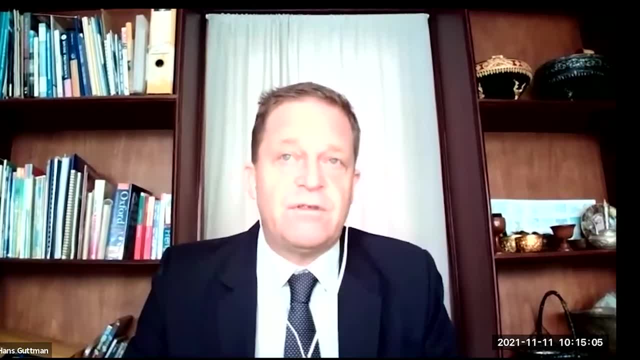 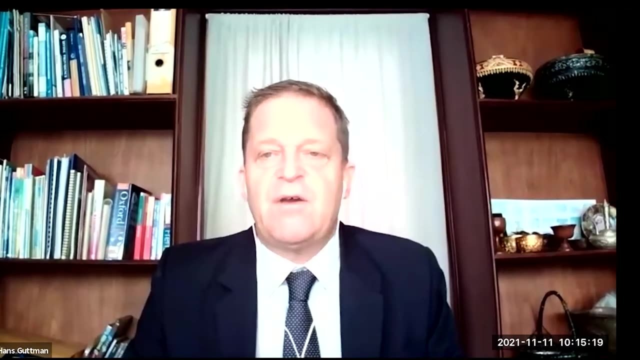 where we have many people, and for food security, which is the greatest user of water. but it needs to be further developed to better handle uncertainty, consider the scale of information collected and the approach available, and the significance of extreme events and the complexity due to other interactions, as well as enhancing the governance and reach into communities. 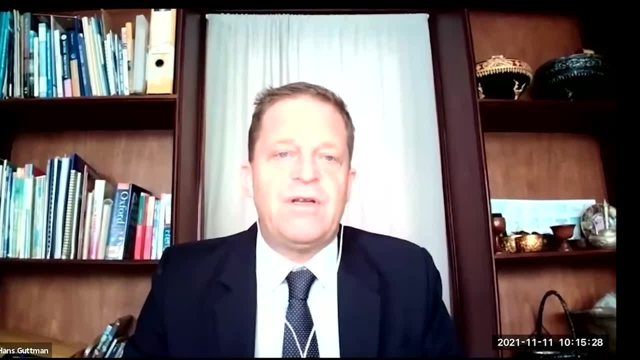 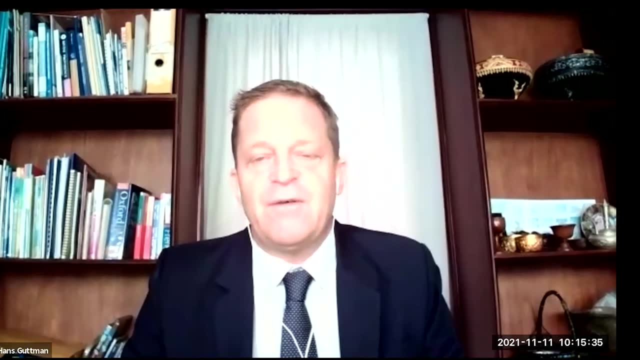 more effectively. leadership was touched upon and is perhaps in many cases more important than the resources available for undertaking this data collection or other functions. and then we had example from lao PDR there and also our experience in the Philippines. there was opportunities to let the communities lead in the resilience building. so with that I would like to thank all of the.